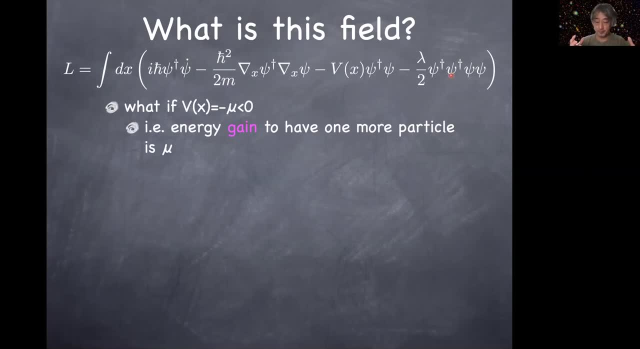 last term here. the particles repel with each other, And especially when the system is very cold, then the system wants to sort of spit out particles, because that is the way you would like to minimize the repulsive energy. But thanks to this addition we are able to do that, And so 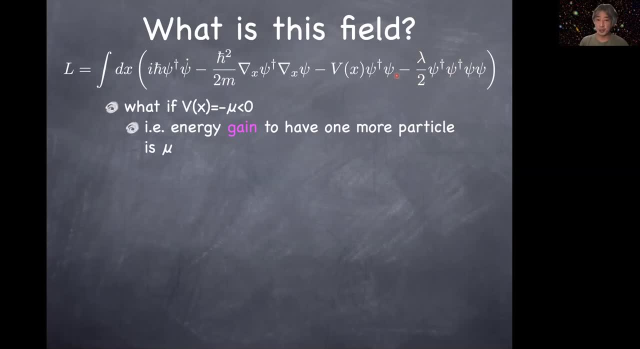 we are able to put in the system because we have the positive chemical potential. you also gain energy by putting more particles into the system. So that is how you can have an equilibrium where you have a certain number of particles, like we are talking about thousands to millions actually. 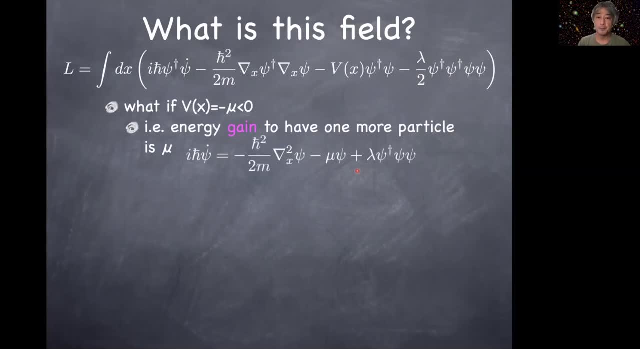 despite the fact that there is this repulsive potential And because we are looking for the classical limit of it, we study the Euler-Lagrange equation. So this is what we have done on Wednesday. In general, we cannot solve this equation, but there are special cases where we can. 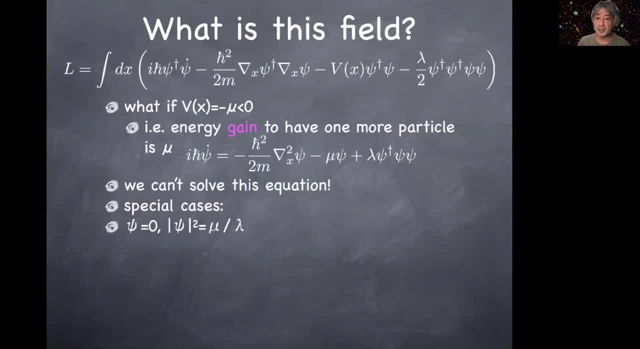 In one case it's sort of trivial, where psi just identically vanishes, so every term in this equation is just zero. But there's a slightly less trivial solution where psi is still a spacetime constant, so that you can ignore these derivative terms. But you can balance the last. 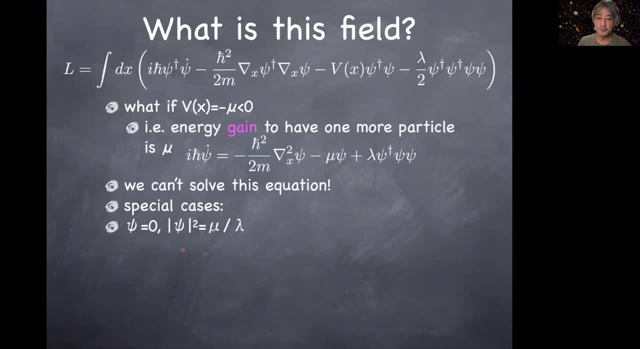 two terms against each other to make sure that that actually vanishes, where psi modulo squared is given by chemical potential over this coupling of the repulsive potential. So that is an exact solution to this Euler-Lagrange equation. Now you can ask the question: which one is more? 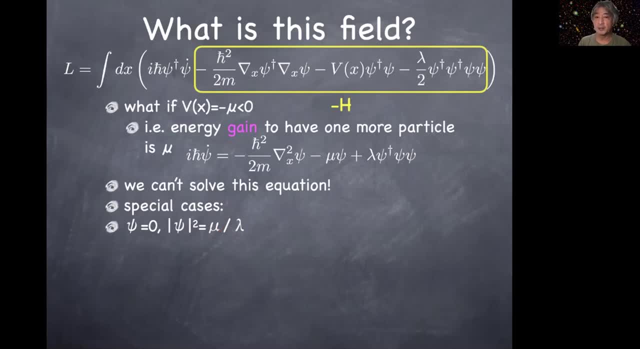 appropriate for us And to answer that question, we looked at the Hamiltonian, which is just a negative of the thing in this yellow box. So this is actually the Hamiltonian now, now that we don't have the derivative of psi because it's spacetime constant, So this is now the. 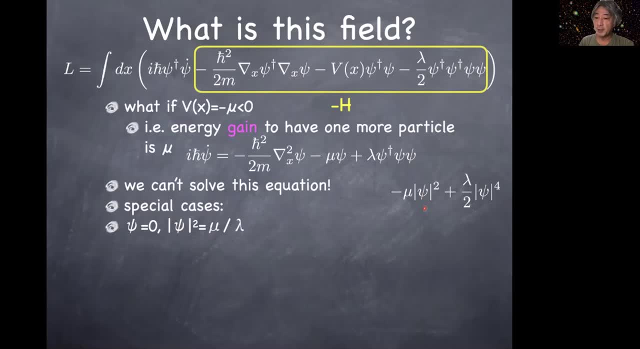 Hamiltonian. So this is the derivative of psi, because it's spacetime constant, And then we can see how this function looks like on the complex plane of the complex variable psi. So here's a real axis, here's the imaginary axis, and on top of this complex plane I plotted. 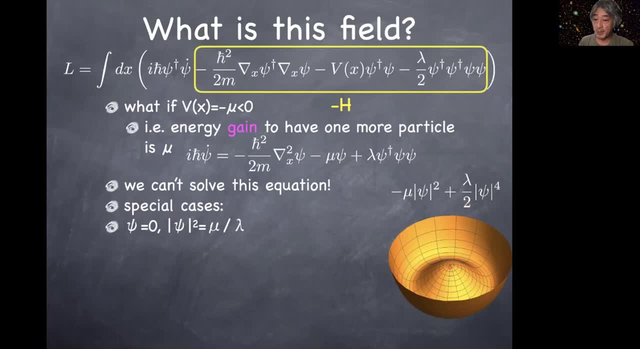 this function here And you have seen this already. So at the origin it vanishes, but you have negative coefficient for the quadratic term. So from the origin the potential starts to go down. But once psi becomes large enough, then quadratic term always wins because of the higher power. 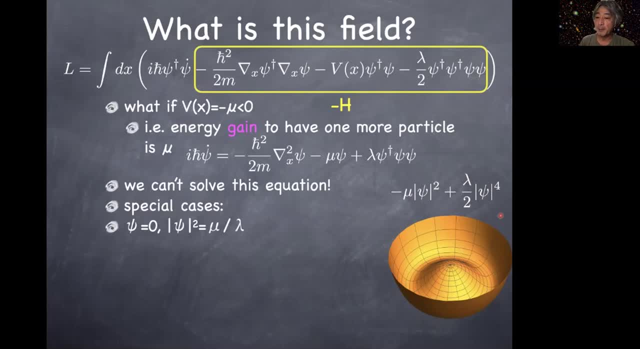 compared to quadratic term. So potential turns around and become larger again, So that develops the minimum somewhere in between. And also because this is a function of the modulus of psi, absolute value of psi. that's the real part squared plus imaginary part squared. it depends. 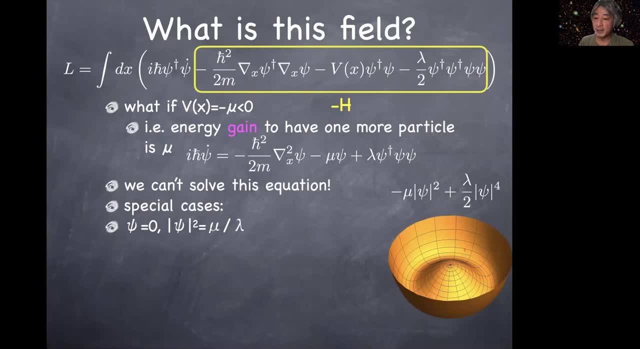 only on the distance from the origin And therefore potential is rotationally or axially symmetric, Rotating around the z-axis. So that's how you understand this formula: potential. And now that if you bring in a ball and put that at the origin and this in principle can stay there forever in 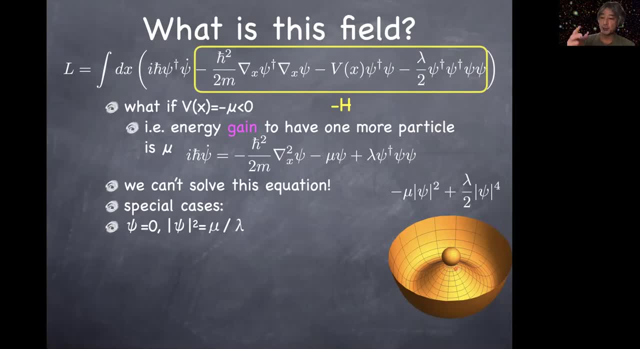 classical mechanics. unless there's some fluctuation that jiggles the balls around, then setting at the origin is indeed a solution of the equation of motion. But you clearly see that this is an unstable solution. if you just nudge it just a tiny bit, it starts to roll down the hill and settle at this, one of the minima. 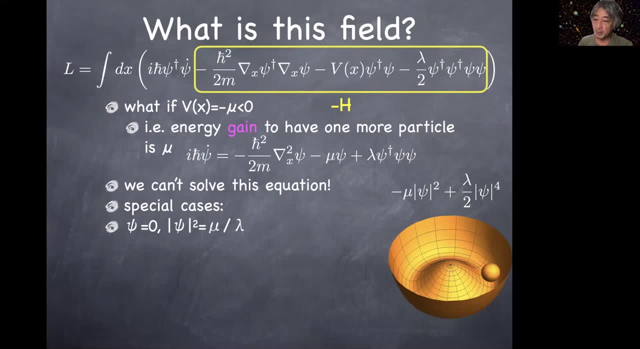 And you see there are actually infinite number of minima around this, at the bottom of this potential, so it settles down somewhere. So, as a result, this seems to be a more appropriate solution to look at. And if you just take the square root of this, psi is given by square root of mu over lambda, but it 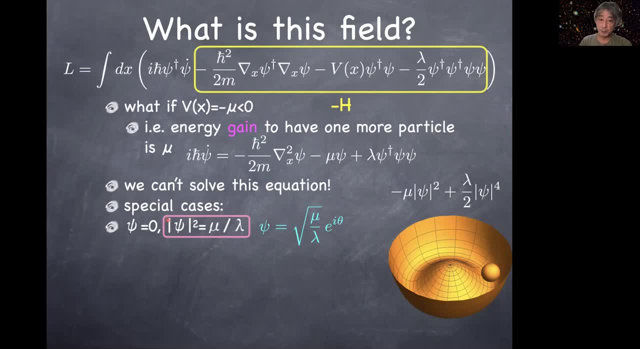 can have an arbitrary phase, because this phase disappears when you take the absolute square. So this phase represents where the minimum can be anywhere along this bottom of this potential. So on the complex plane of the real axis and imaginary axis, the phase e to the i theta corresponds to the angle. 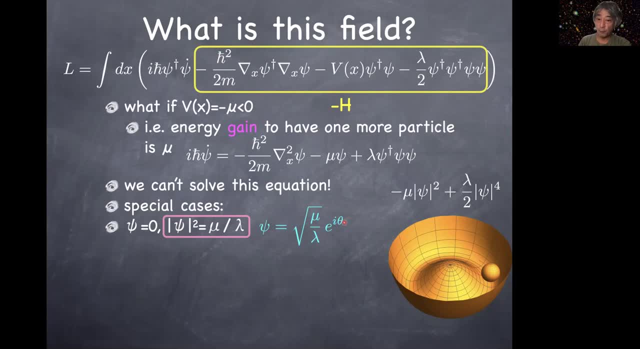 in this direction, And so this is the solution for any theta you like. So there's an infinite number of solutions of this type solving the Euler-Lagrange equation, And once you have the solution, we can actually also go to a different reference. 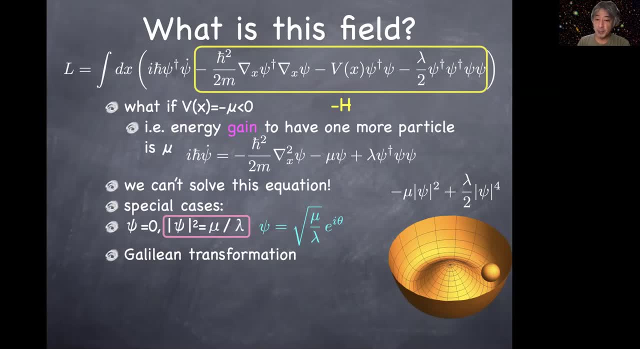 So we can actually also go to a different reference frame by performing Galilean transformation. So this solution basically corresponds to the gas of atoms sitting at rest. But if you go to a different reference frame then you're looking at the gas of atoms sitting at rest from your reference. 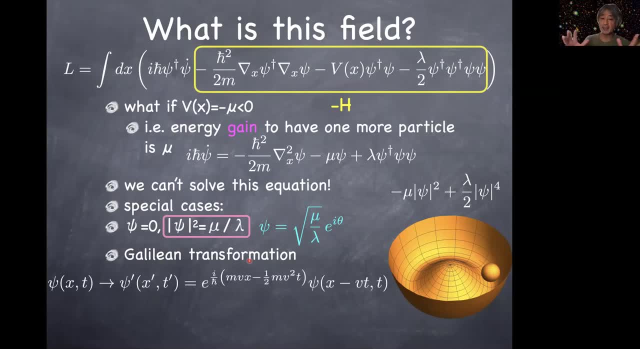 frame that's moving relative to it. So from your point of view, this looks like it's a gas of atoms moving together in a flow. So, going to the new reference frame and we can see that it's the gas of atoms that's moving in that direction And that's the 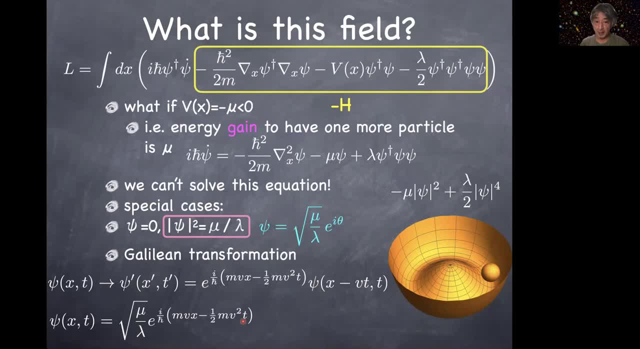 Euler-Lagrange equation. So the Euler-Lagrange equation and you can see that it's actually going to be the Euler-Lagrange equation. So in this case I'm going to use the Euler-Lagrange equation And the Euler-Lagrange equation is going to be the Euler-Lagrange equation. Okay, good, So now I'm going to show you some more examples. So this is the Euler-Lagrange equation and this is a just a very simple transformation, So it ends up in this form over here. So now you have a solution which depends on space and time, but because of the fact the Euler-Lagrange equation's covariant under the Galilean transformation, it is guaranteed also an exact solution. And 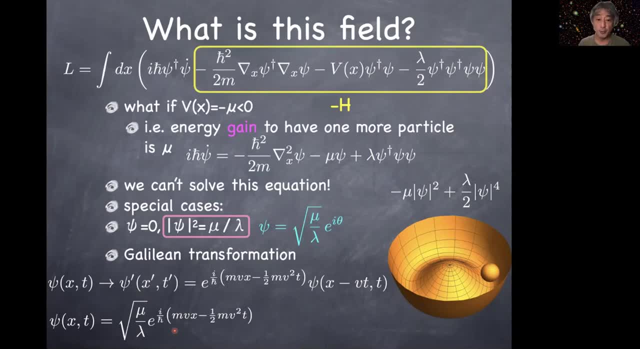 easy to verify and that is going to be part of your next homework problem. If you stick in this solution to this order Lagrange equation, the time derivative will pull out half mv. squared spatial derivative will pull out mv and, together with this prefactor, you are just basically saying that half mv squared is. 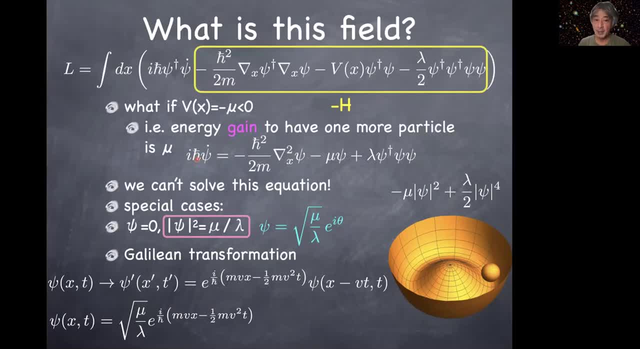 the same as half mv squared. So that's how you see the first two terms balance against each other, And the third and fourth terms has to do with taking the absolute square of psi here and putting them together. So just the condition that this is at the bottom of potential is already good enough to show that this is. 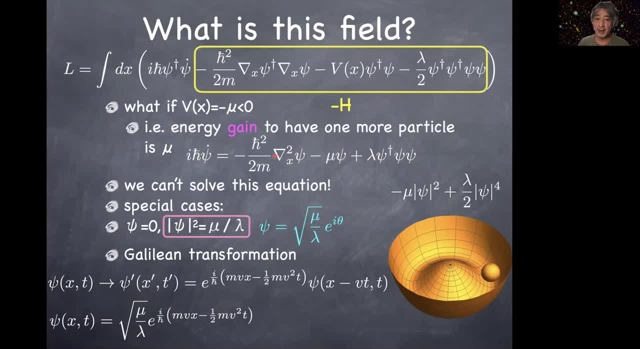 actually zero as well. So first and second term balance against each other. third and fourth terms cancel against each other, so that this equation motion is satisfied. So this is yet another special case where we can solve this nonlinear derivative. So let's look at the differential equation exactly, And there's also a 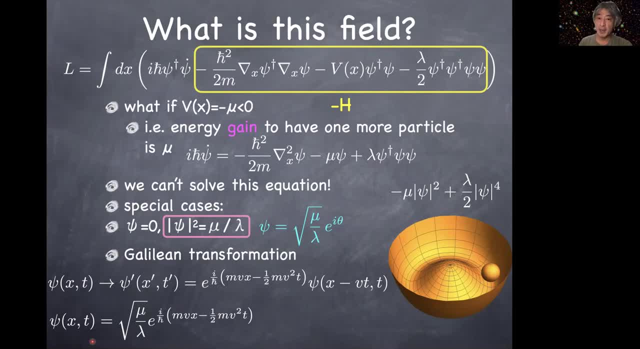 physical meaning to it because, if you remember, psi dagger of psi, integrated over the entire space, is the number operator of particles. So psi dagger of psi has a meaning of the number density. So the prefactor here ends up having the meaning of the square root of number density, together with this plane wave. 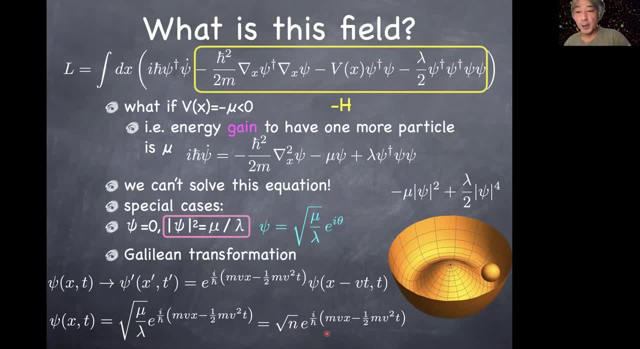 factor. So that's a definite solution to the order Lagrange equation coming from this Lagrange. Okay, let me stop here Then pause for some questions. Well, you've seen this already on Wednesday, so maybe not that many questions, But you know I nonetheless 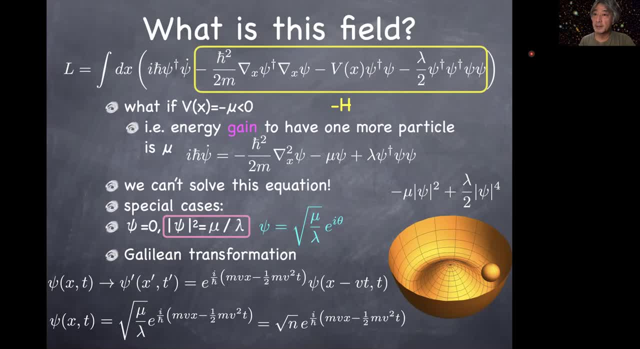 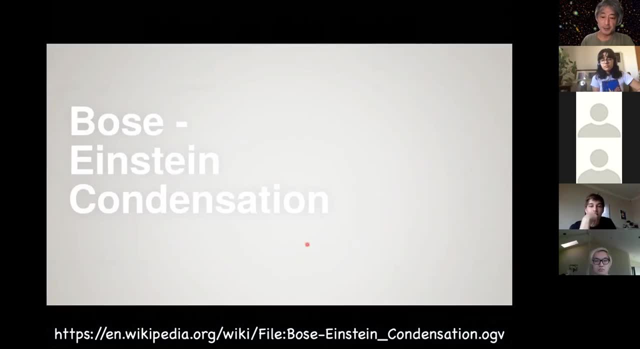 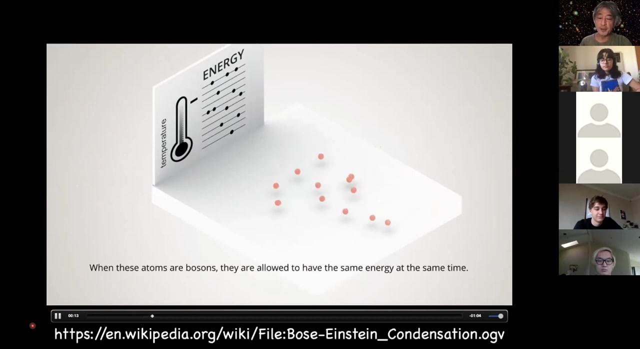 ask for a wait for that. Everything okay, All right. And you have seen this video too, but it's such a fun, So let me show this again. So, at high temperature, all these atoms are moving fast And you start to cool this system. 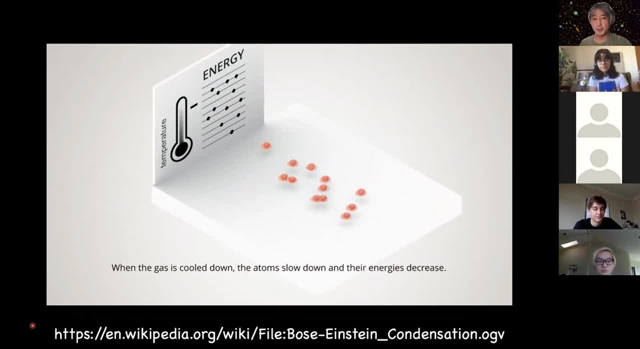 And these fast-moving atoms correspond to some of these excited states on this chart. But as you cool the system they start to come down to a lower and lower energy force And size of each wave function grows, because being thrown means no momentum, All right. 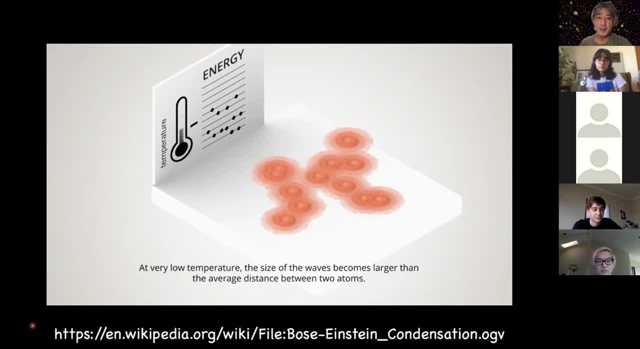 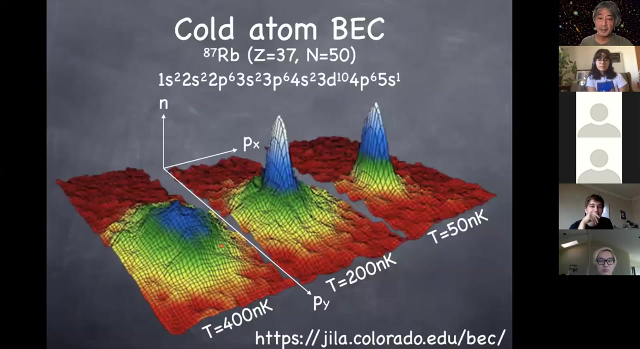 and this is also what I have shown you on Wednesday, and people have done this experiment using rubidium atom, and rubidium is one of the alkaline elements, so you have one free valence electron in s orbital and all the other orbitals at the lower levels are: 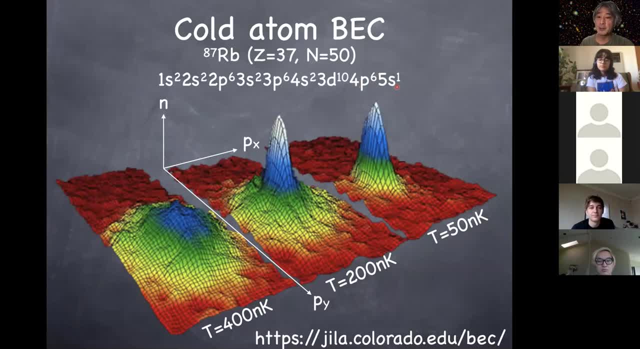 occupied in their closed shells, and the reason why this atom is actually useful is that, because of this isolated single valence electron, an electron has a magnetic moment when you actually apply magnetic field to the system, and that basically creates a potential to the atoms, and so, by shaping the form of the magnetic field appropriately, you can produce. 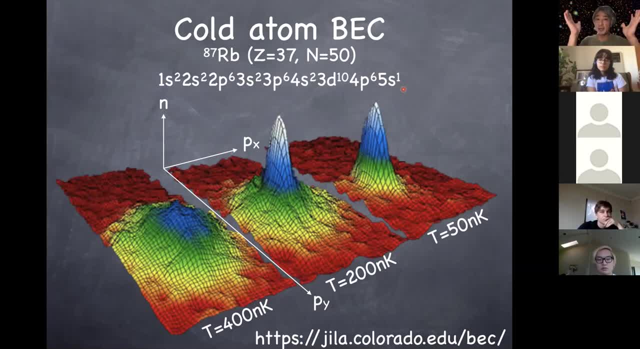 basically parabolic potential, like in a harmonic oscillator, to trap these atoms and and then you can start to see how this system would cool and eventually form a macroscopic number of the atoms occupying zero momentum state. so this is the plane of px and py, so this is a momentum space in x and 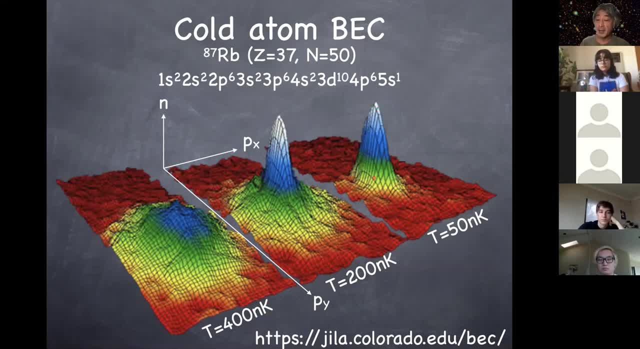 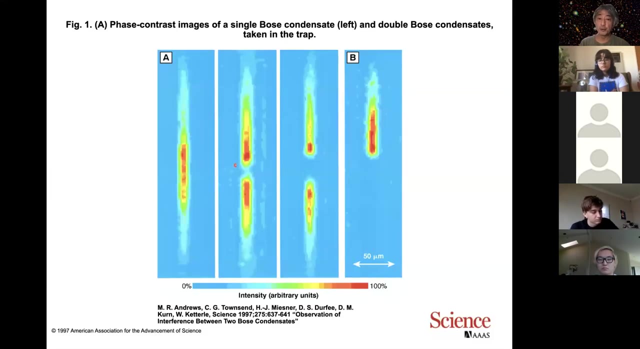 y directions. the fact that you have this big blob at the center means that you have this macroscopic number of atoms all occupying the zero momentum state, and so that's the idea of boson and condensate, and I told you already that you can let two bosons and condensates to overlap with each other, and so each boson condensate. 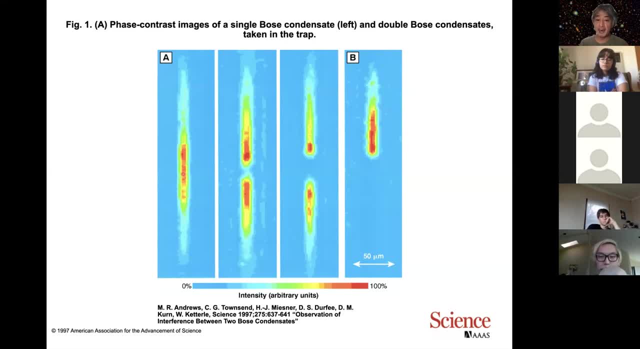 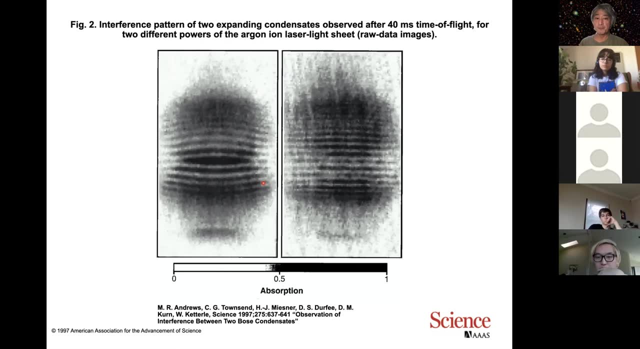 consists of thousands or even millions of atoms and, and, but they, when they overlap, they actually show this fringe pattern and that's an evidence that you can actually see that this is the actually show this fringe pattern and that this is the effect time where the Over Cruz. 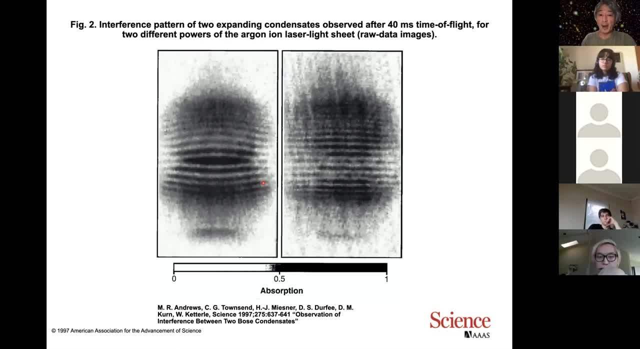 Pushedир aqui. both of these, both pige and condensates, actually behave like a classical wave. so that's a demonstration that the macroscopic number of atoms together will behave as if that whole collection is a classical wave of some sort. and that's the weird thing about both aisle and condensate. so 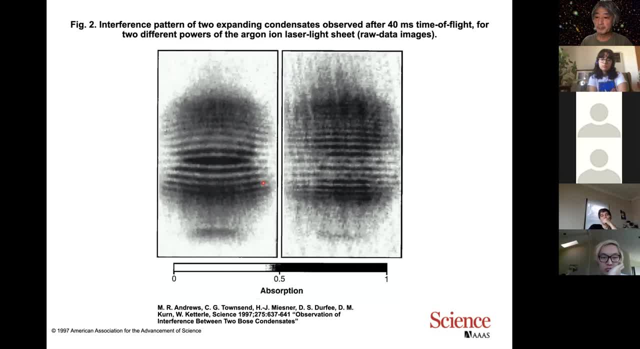 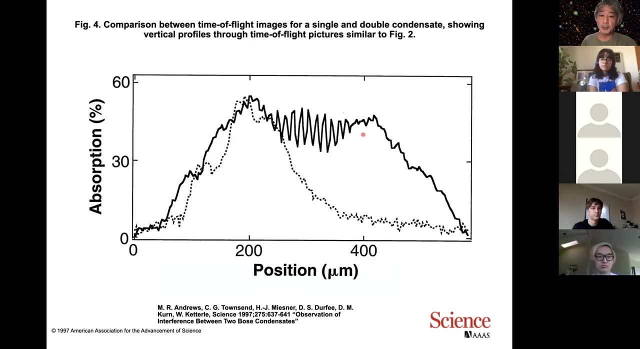 let me stop here and if you have any questions, everything okay, not good, all All right, and we can be more quantitative about this. So this fringe pattern is basically the variation in number densities, And so this is actually a picture of the data by shining light on the system. 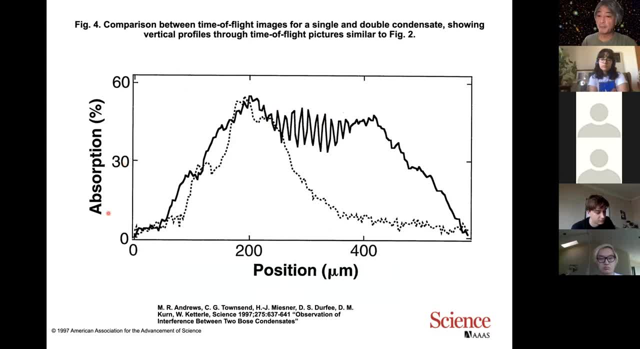 This zigzag curve shows the absorption probability of the light you have shown on this system And this zigzag means that you have high density, low density, high density, low density, variation in density over this range of the system, And this is what corresponds to the fringe pattern you saw on the previous slide. 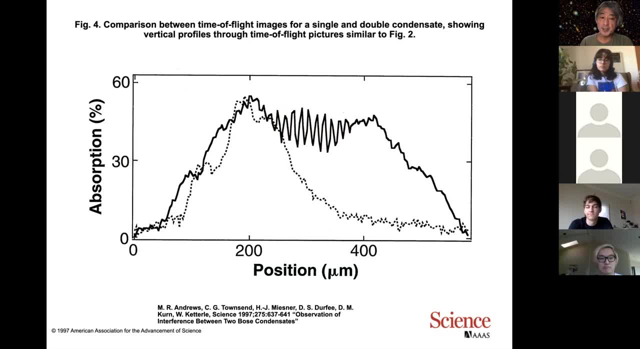 But if you don't have two bosons and condensates overlapping with each other, you basically have this sort of Gaussian-shaped blob. There's no zigzag going on there. Only when two of them overlap you have this zigzag. So that's the fringe pattern of two classical waves. 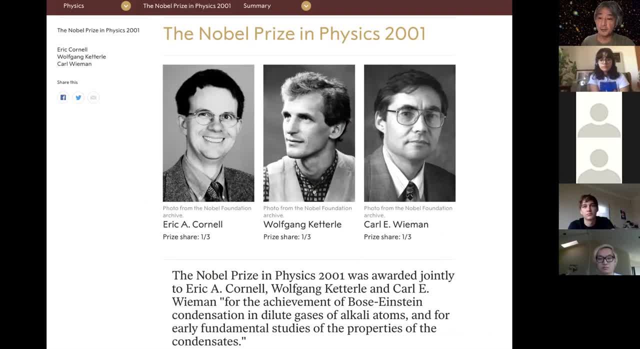 And so these gentlemen received the Nobel Prize in Physics. Nobel Prize in Physics in 2001.. Is that about the time when you were born? I guess, But in the history of physics that's fairly recent. You need to understand that. 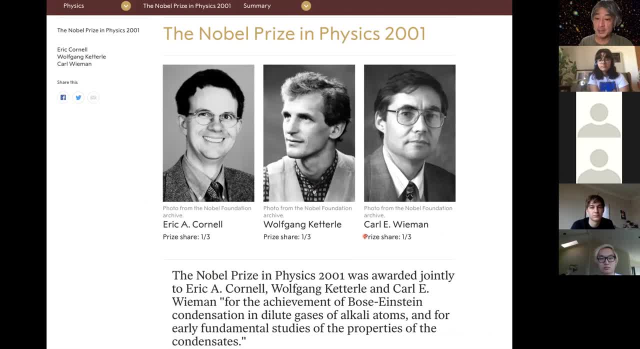 So this boson-shun condensate of cold dilute gas of atoms is a relatively recent discovery, And that's because people had to do a rather immense technological advancement to be able to produce a system like this, Because you have to go to incredibly large amounts of energy. 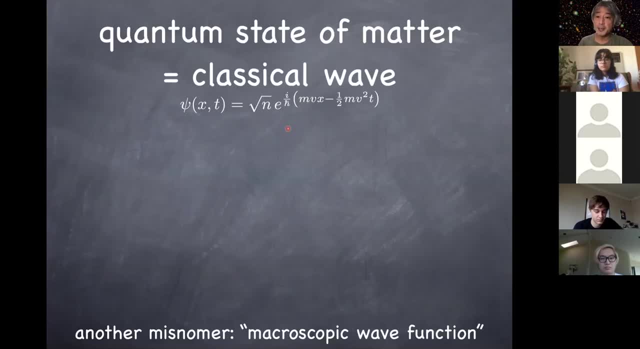 And you have to go to incredibly large amounts of energy. And you have to go to incredibly large amounts of energy. And so the problem is that in the literature we would not have known that these two thing with the burns of very high temperature and very low temperature for this. 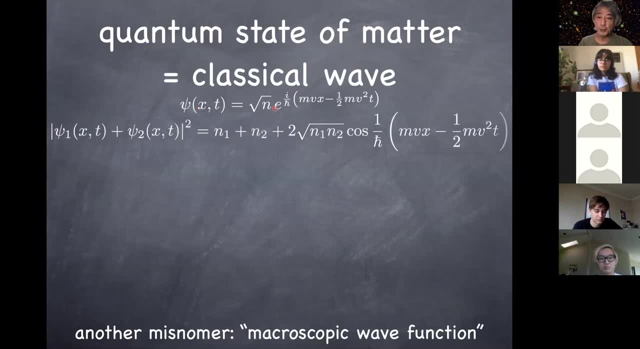 But anyway. so let us just verify that interference of two waves- we have obtained these solutions already- would actually produce this fringe pattern. So I have this solution, So I use two of them. So one, psi 1, has square root n1 and specific velocities v1.. 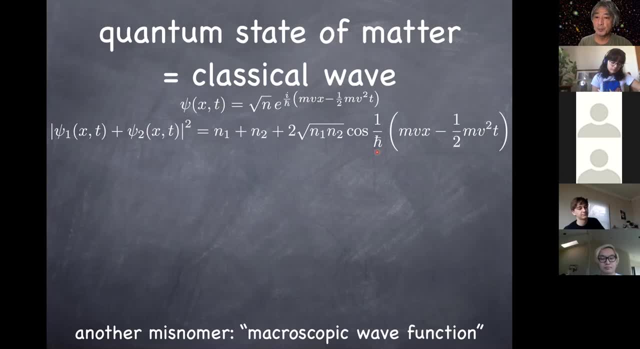 Second one, psi 2, has the number, there's the n2.. then you find this result: So this one squared would give you n1,, this one squared would give you n2, then you have the cross terms. the cross term has, of course, square root of n1 times square. 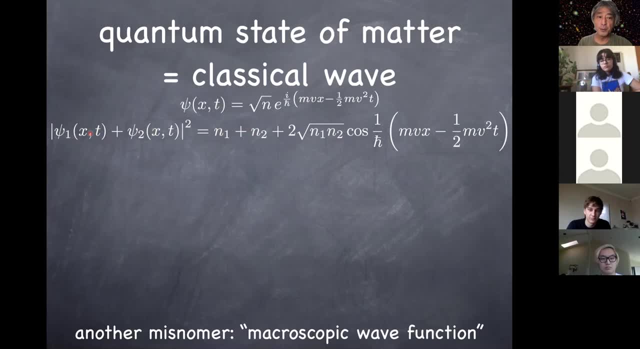 root of n2,. and then you have product of the plane wave factors and one of them is complex conjugated. So using this solution for v1 and using the complex conjugate of the solution v2,, effectively what you do is to subtract v1 from v2.. So in this expression this v is meant to be: 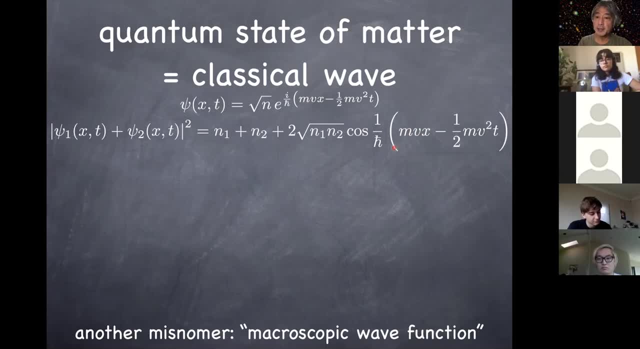 relative velocity. So this is the way you can see that you have this cosine variation in space and that's the zigzag you have seen in the data on the previous slide. So I would like to emphasize that this psi1, psi2 are definitely not wave functions, on two accounts. First of all, 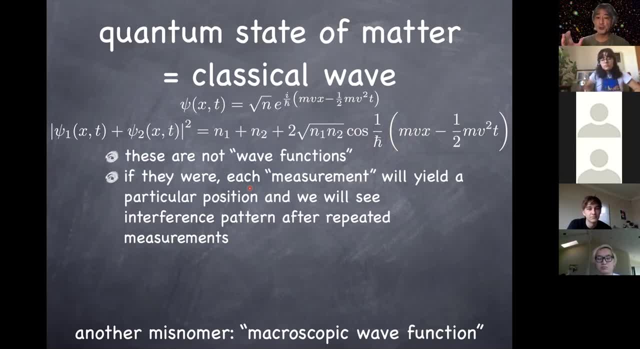 if they're not wave functions, then they're not wave functions. If they're not wave functions, they were wave functions, then each measurement would collapse, the entire system to the position eigenstate. So you have to keep repeating the same measurements over and over again. 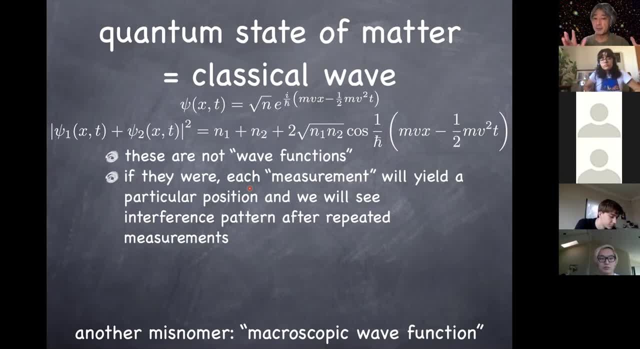 until you can see the fringe pattern, And that's what you have seen, for example, in double slit experiment, right, But this time you just shine the light and then you see this zigzag pattern all at once. So this is not quantum mechanical wave function, this is a classical wave. you 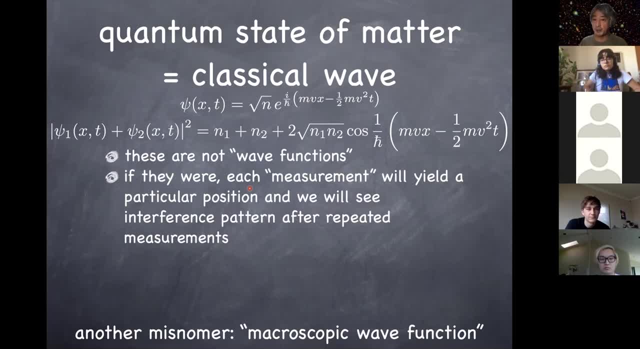 can measure as a whole by single measurement. So that's one reason why this is definitely not a usual quantum mechanical wave function. Another reason is that this is the multi-body system of thousands of atoms and the wave function has to be a function with arguments. 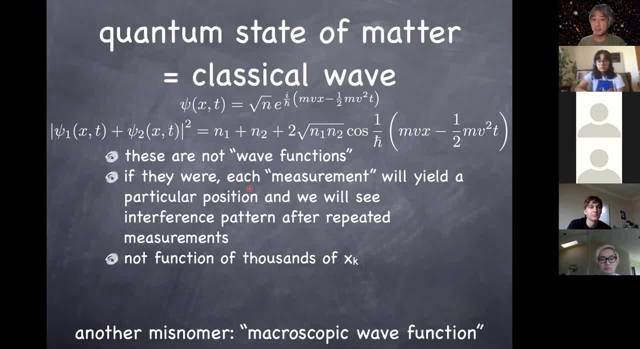 each of which correspond to the position of one of these atoms. So it's a huge function that has something like a three times thousand coordinates inside the function. But this is not that. This is a function of just space and only single spatial position, not thousands of them. So based on these two reasons, this psi should not be looked at. 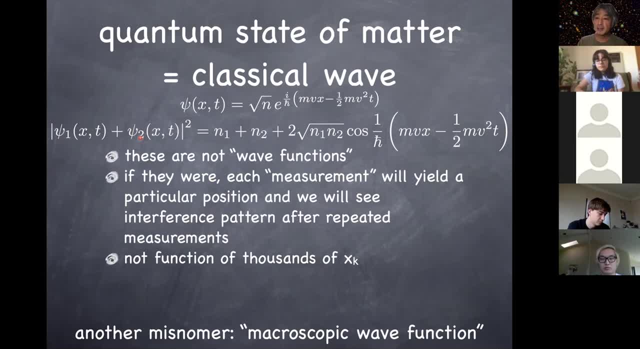 as a wave function, but rather this is actually a classical limit of the field we've been talking about, And it's a field because it's a function of space and time, And that means this is actually a classical wave. So this is actually a very strange thing that you have these thousands of atoms. 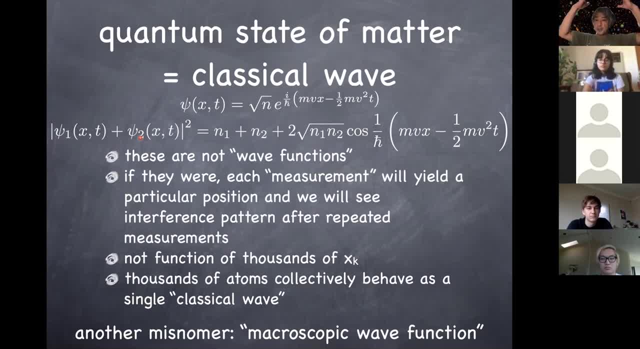 interacting with each other with possible potential, and you're cooling the system without an incredibly low temperature. But after cooling it down, this collection of particles will start to behave as if this whole system is a classical wave. So from the point of view of standard quantum mechanics, this is a highly quantum phenomenon. Macroscopic numbers. 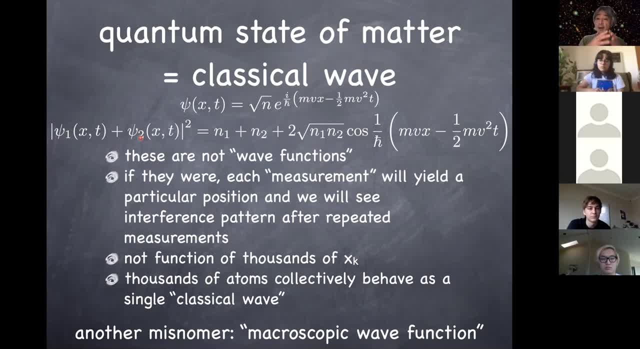 for example of quantum objects, behave collectively as a classical wave. On the other hand, from the point of view of the quantum field theory- the quantum field theory describes multiparticle system, as you have been going through in your past two homework problems. 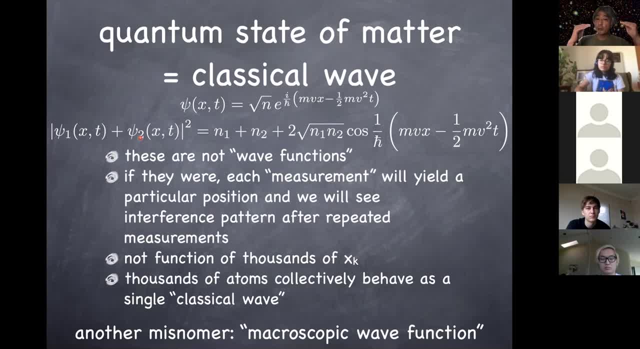 So now you know that is the case. But quantum field theory can also describe physics. when you take a classical limit, where the classical wave actually represents this highly quantum state of which is called a quantum dimension And its complex domain is called a quantum dimension. 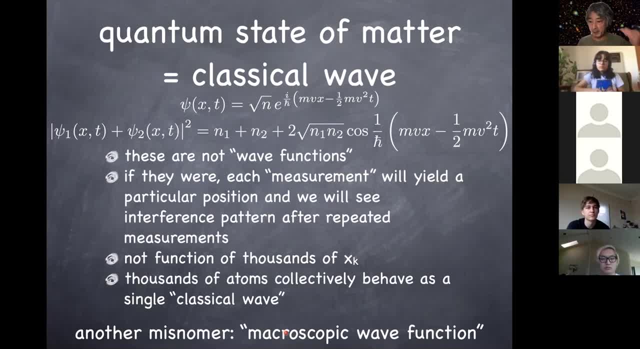 And some of you might be wondering: what are theAU? all these things, And I've described them in the last lecture, but once again, that's a mathematical number that I can show, because I'll show you what an entire wave is instead of a quantum dimension. 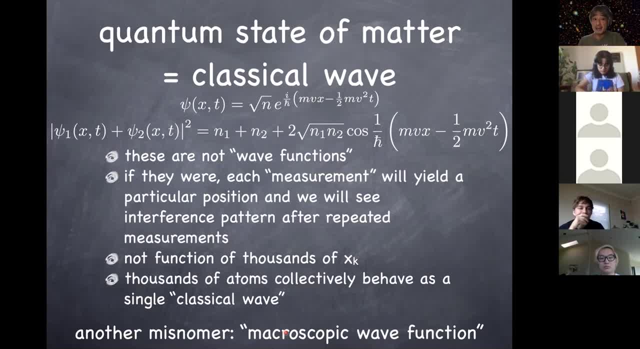 Now what we're going to do is I'm going to explain something called a quantum dimension. So what they called the quantum dimension is a quantum dimension, and at the beginning of this lecture we explained what a quantum dimension was. know, it's also nonlinear, so it's definitely not Schrodinger equation, but looks similar. 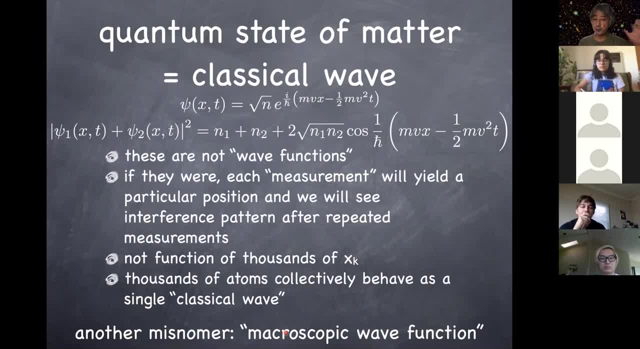 You also now know the reason why they look similar: because both Schrodinger equation and this field equation have to be invariant under Galilean transformation and that's why they both look similar. with a combination of time derivative and spatial derivative squared, 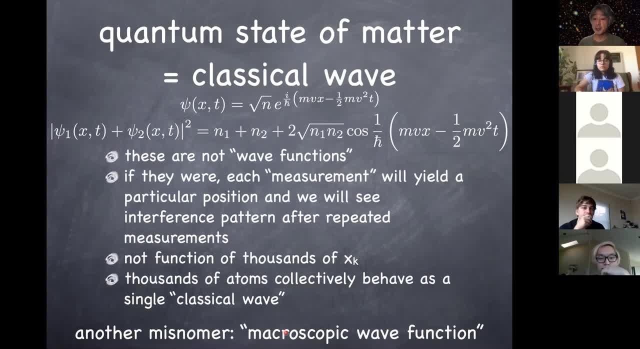 So you know all these reasons by now. So now you see why this is a wrong name to use. but just in case that you might come across this terminology in reading papers, what they actually mean is this classical limit of the quantum field. So this is how you can. 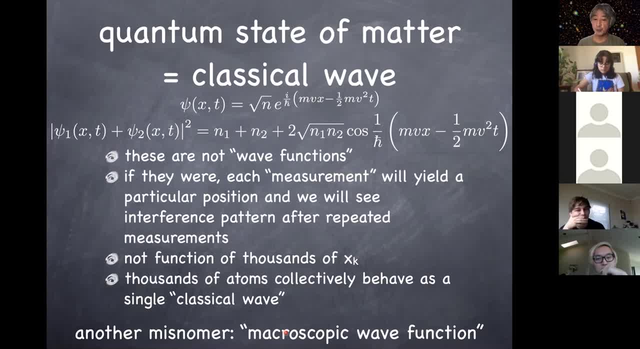 really understand this zigzag behavior of the two boson-Schrodinger condensate using the exact solutions we have gotten for the Euler-Lagrange equation in quantum field theory. Okay, let me stop here and pause again if there are any questions. I just wanted to quickly ask was: 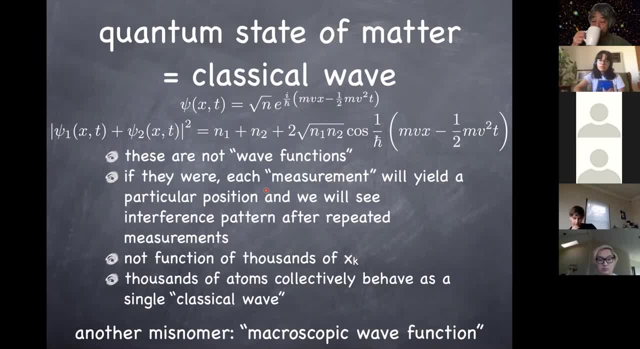 there a reason for the quantum field theory to be so similar to the Euler-Lagrange equation? Is it because of the particular onsets of having a constant psi, or is that just an easy solution? Yeah, so this is definitely the idealization right, Because this is if you take absolute. 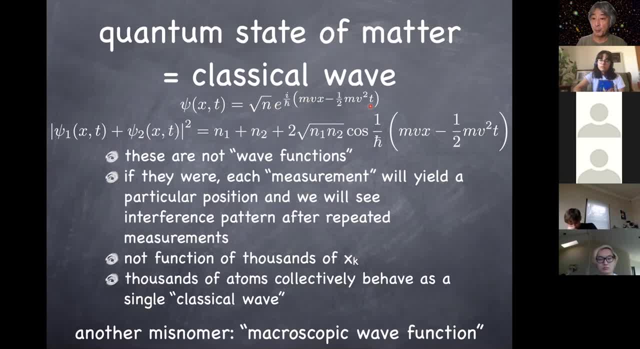 squared, that's constant in space and time, And the real boson-Schrodinger condensate have been produced by creating a trap, So it's inside a potential and so it has a sort of Gaussian-like shape in it. So this is definitely an idealization. But in order to solve this Euler-Lagrange equation, 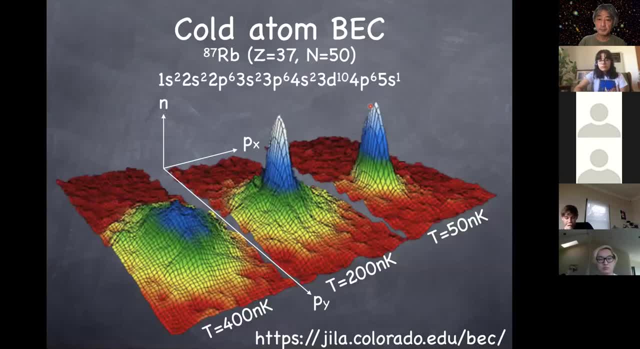 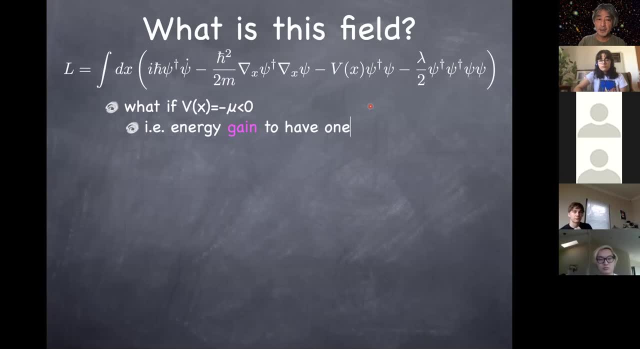 in the presence of both. you have to have a constant psi and you have to have a constant psi. So you have to have a constant psi in order to solve this Euler-Lagrange equation. Sorry, I'm trying to get the Euler-Lagrange equation in the presence of this. 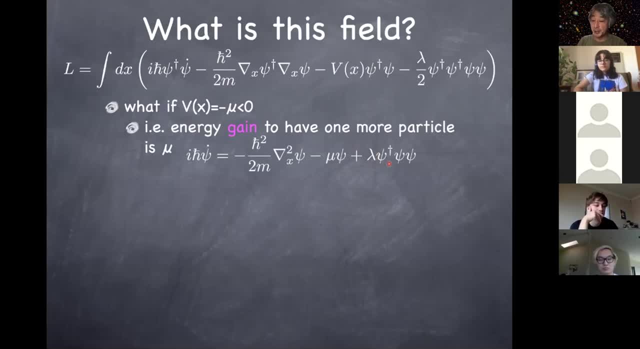 the interaction term, And this is a nonlinear equation, so you can even use a superposition principle to obtain new solutions out of two solutions, And in general this is very difficult to solve. Numerically. it's not that hard, So once you're given the solution, 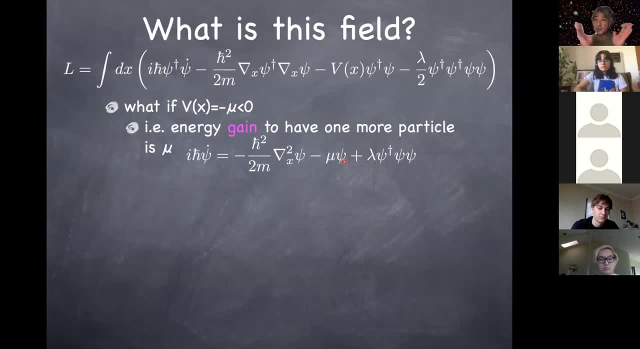 and you can also put in this external potential if you like, with this potential well, from this magnetic field, then you can go ahead and solve for the solution together with the external potential and this interaction term as well. So it's not a difficult problem numerically. 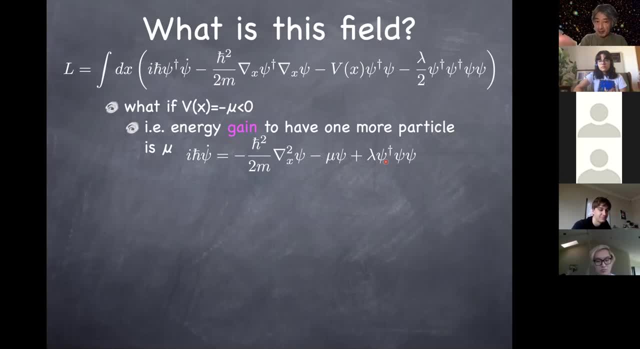 but because I'd like to show you how things work on basically the blackboard or slides on a piece of paper or whatever. That's why I wanted to specialize it to sort of the idealized situation of the space-time constant solution without any external potential acting on it, And we have this boring solution which is just purely constant. 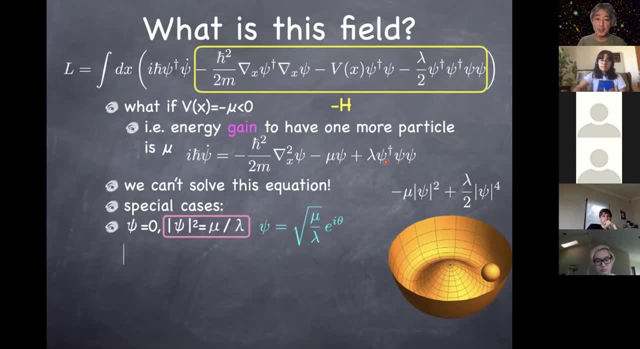 But we also generalize this a little bit by going to an arbitrary reference frame, so that we at least have this exact solution which corresponds to this moving Bose-Einstein condensate. So the fact that two Bose-Einstein condensates are moving with relative velocity. 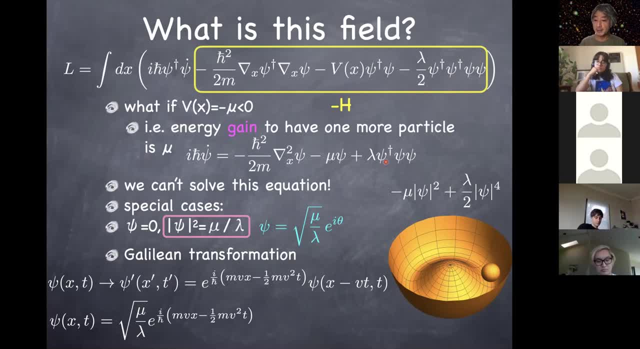 is what's causing the interference pattern, as you saw on the last slide. So this is at least generic enough for our purposes to understand the origin of the fringe pattern. So once again, this is not general enough. Actual situation is more complicated. You have to resort to numerical. 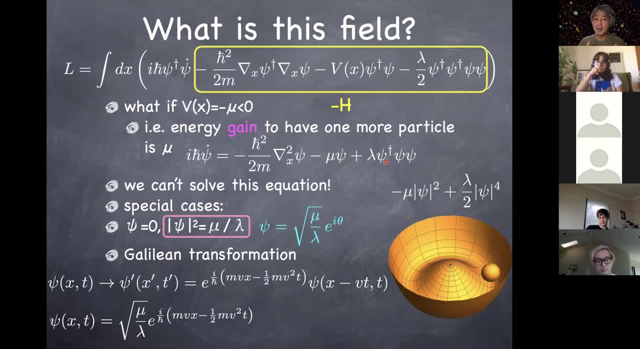 solution to the differential equation, But for the purpose of understanding why you expect to see the fringe pattern when two Bose-Einstein condensates overlap. this solution turned out to be general enough, and that's why I'm using that solution. Does that answer your question? 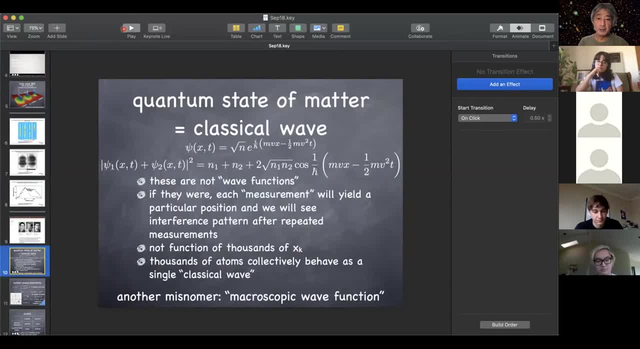 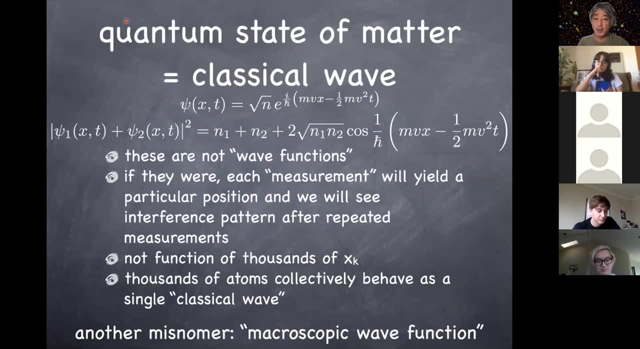 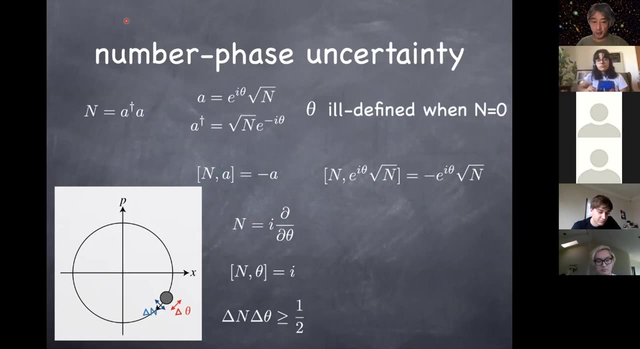 Yeah, thank you. Okay. So we have now gotten to this origin of the fringe pattern by looking at the solutions to the classical Euler-Lagrange equation, And here is a reminder that this solution can be understood as the coherent state we have studied in harmonic oscillator And in 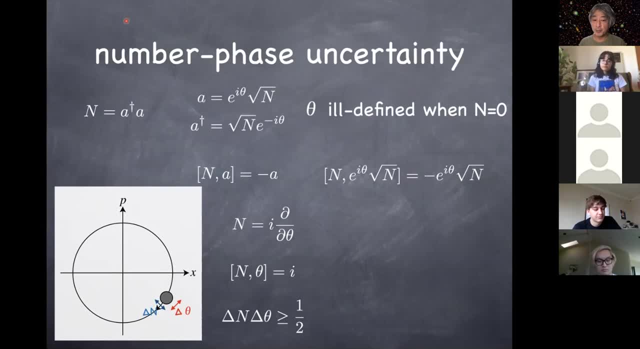 the case of a harmonic oscillator, the coherent states correspond to slightly uncertain n, and n is the level of the excited states. But rather, when we look at the harmonic oscillator, we can see that n is a well-defined phase, And now that we are dealing with the quantum field, 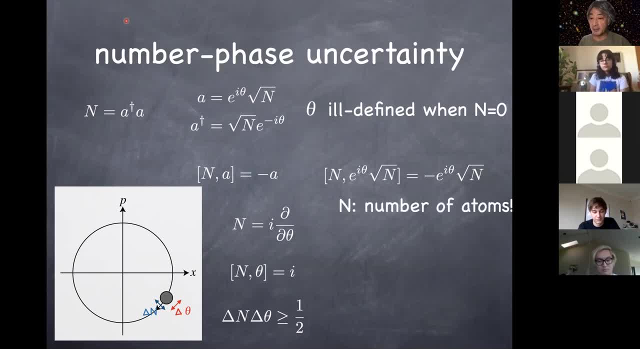 theory rather than the harmonic oscillator. now, you know, n corresponds to the number of atoms in the system, So number state has a definite number of atoms. So in our case we have two Bose-Einstein condensates and total number of atoms is clearly a fixed number. However, when you 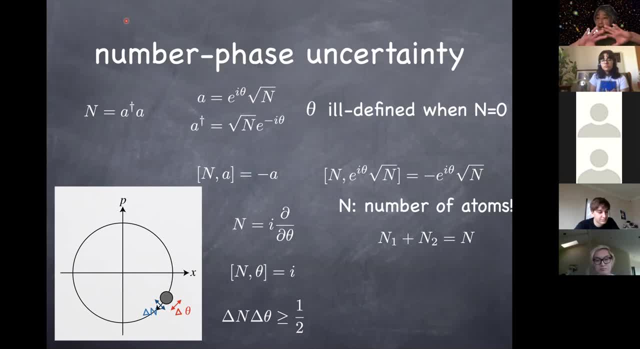 look at the number of atoms in each of the condensates. every atom is an identical boson. They can sort of freely move whether they belong to the first condensate or second condensate. So n1, n2 each can be actually uncertain. And because n1 minus, 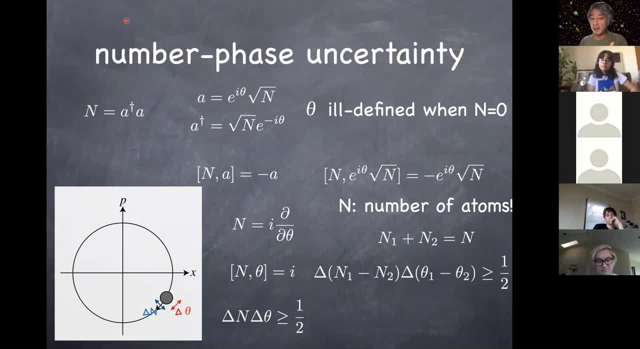 n2 can be uncertain. correspondingly, the relative phase between the condensates- theta1 minus theta2, can be certain to a certain degree. Pun not intended, But anyway. so you can see that n is a well-defined relative phase between two condensates And the relative phase. 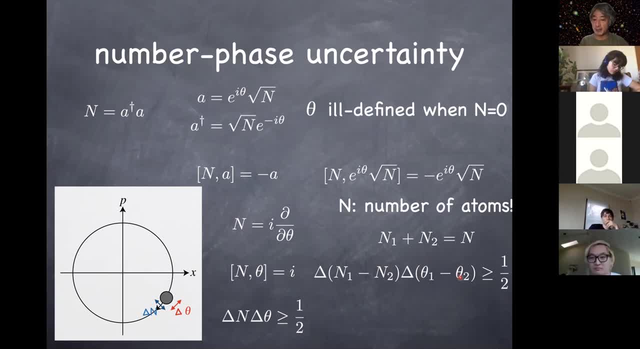 is what's really causing this fringe pattern, as you saw in the previous slide. So that's really what's going on here. So, as a matter of fact, this Bose-Einstein condensate described by this classical wave corresponds to the coherent state. if you build a Hilbert space And coherent state. 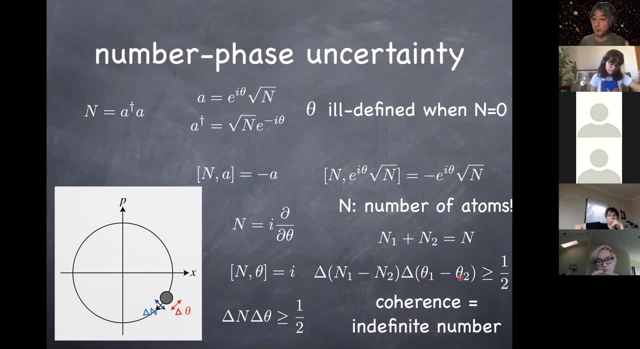 is coherent, namely that it can have this rather well-defined phase At the expense of making the number somewhat uncertain. And this number phase uncertain principle is really manifested in this system And the coherence is what makes the Bose-Einstein condensate behave like a classical wave And they interfere and shows the fringe pattern. 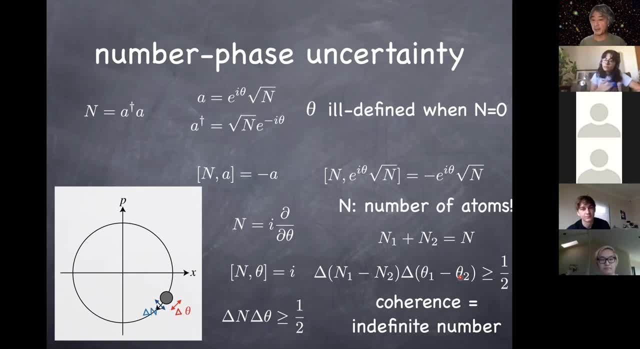 And ultimately the origin of that has to do with the fact that relative number of the two condensates can be uncertain because the atoms can move back and forth between two condensates. Okay, this is just a little conceptual point about this. 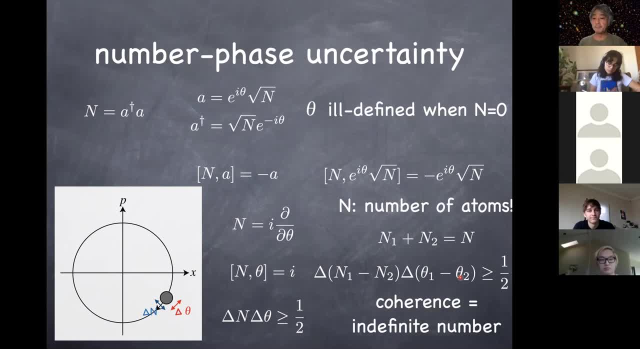 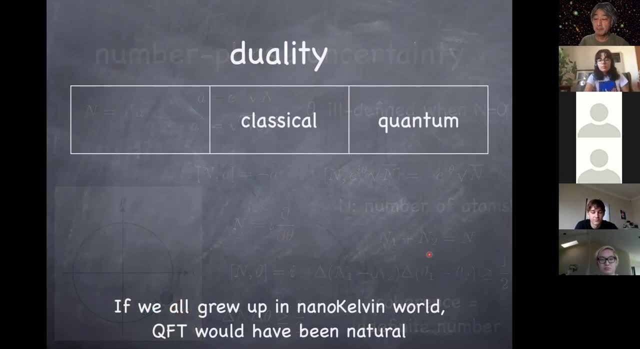 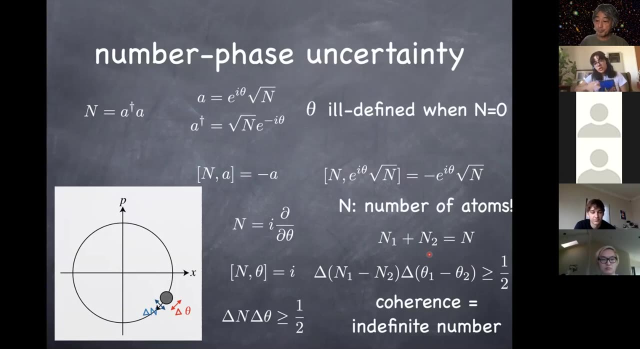 Any questions about that? Everything clear? Okay, go ahead. Oh yeah, I was just wondering. I mean, because we've had the coherent state in the harmonic oscillator system, kind of correspond to more classical, like our classical expectations in here again. 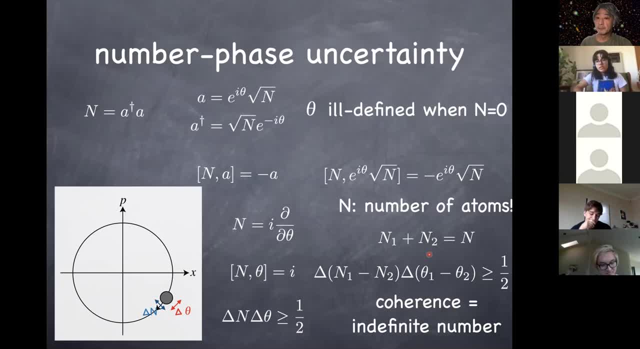 Right. So is that like a general rule because of this kind of definite phase property that they end up recreating kind of the classical limit of the system? That's right So, if you remember the way we introduced this idea of coherent state. 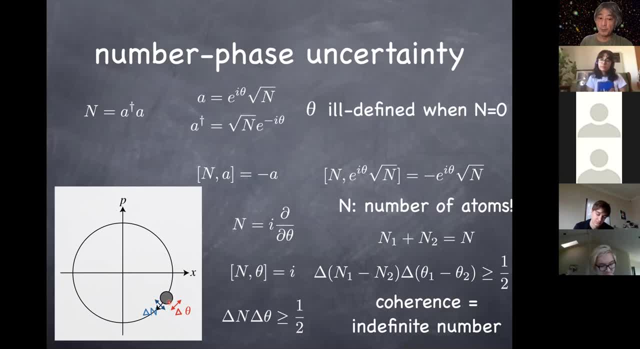 is that, to mimic classical pendulum, we want to have both x and p specified within the uncertain principle. So having both x and y specified was achieved by having an eigenvalue of the annihilation operator, because annihilation operator is, roughly speaking, x plus. 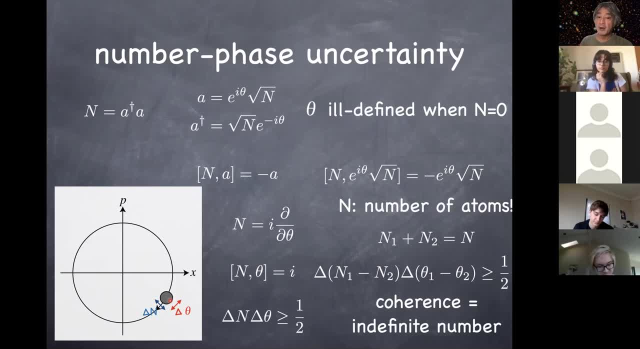 ip. So eigenvalue, which is complex, of the annihilation operator, tells you that real part corresponds to x, imaginary part corresponds to p, so that you have both x and p specified, to the extent that Mr Heisenberg wouldn't be mad at us. So now that you have both x and p, 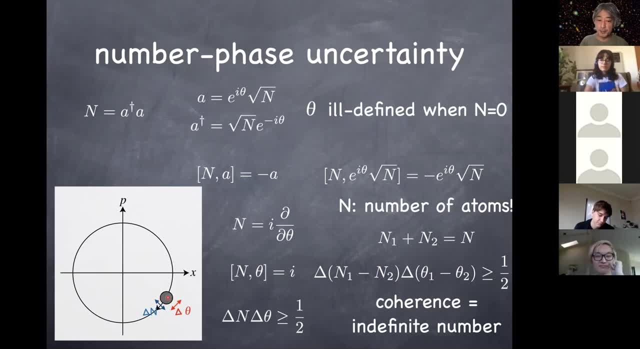 that mimics this classical pendulum, especially when this blob is away from the origin. So we're dealing with the same situation. The psi is annihilation operator. Now we are talking about eigenstate of the annihilation operator, where you have n times e to the i theta is the. 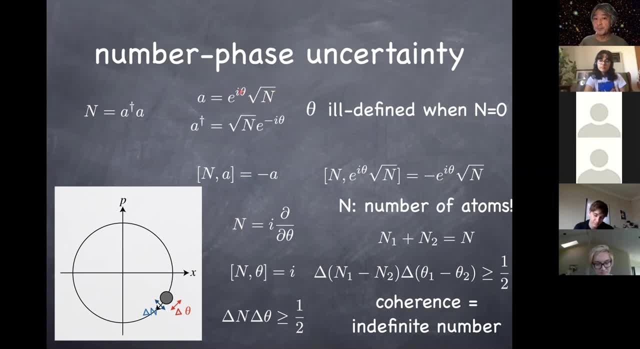 annihilation operator. So now you have both n and theta specified to a certain degree. So that's how you can have more or less well-defined number, but it's a little bit uncertain. And then you have also more or less well-defined phase, which is also 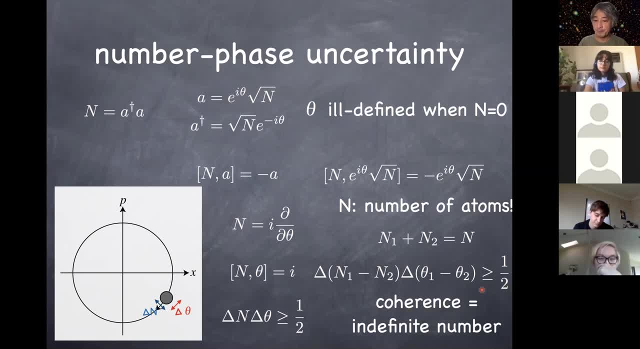 a little bit uncertain, allowed by this uncertainty principle, But when the number of particles is macroscopic, thousands of millions, even if you allow say uncertainty by a couple, this is a big number, so the theta can be extremely well-defined and hence you can observe 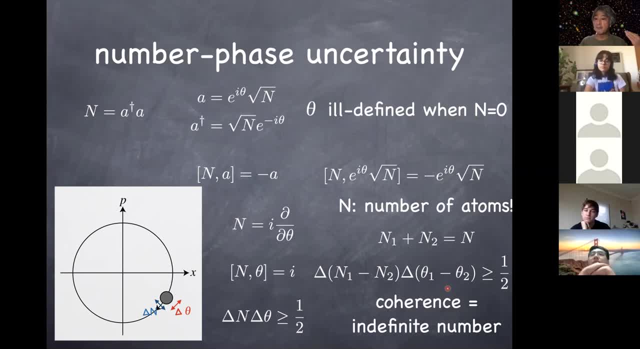 this coherence of the waves in fringe pattern very, very clearly in experiments. Thank you for asking the question, Anna. Yeah, thanks, That makes a lot of sense. Okay, any further questions on this, And I forgot to mention something very important. 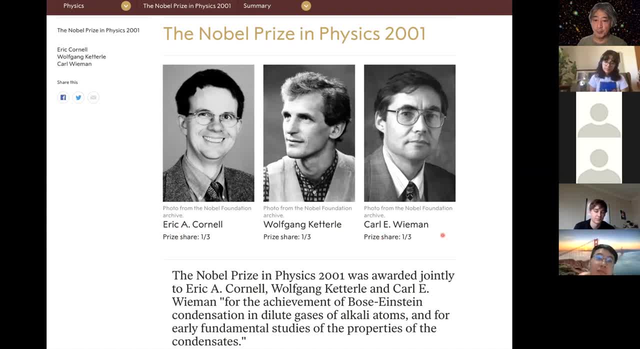 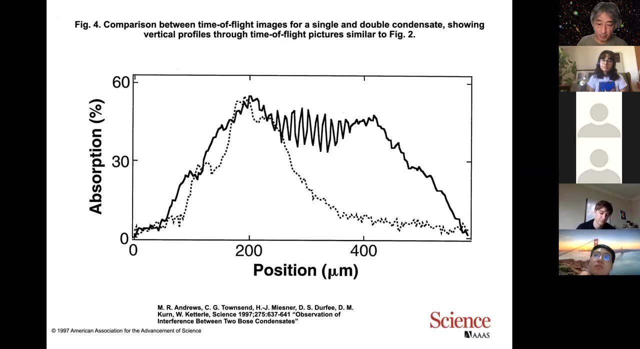 So there are three people who got an Nobel Prize and shared an Nobel Prize, And Wolfgang Ketterle worked at MIT, Eric Corden and Carl Wieman worked in University of Colorado and NIST in Boulder, And the work done by Wolfgang Ketterle, as you see in this reference here, is, of course, multi-order. 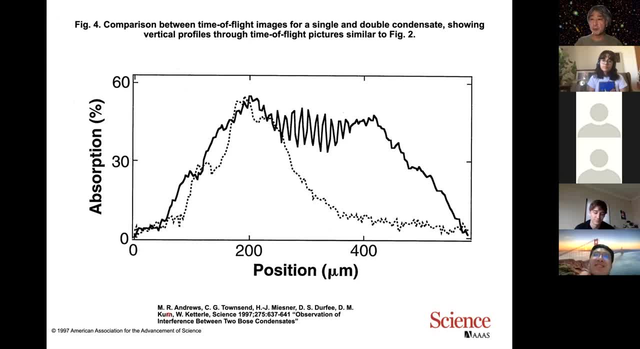 paper And this, DM Kern is our own student, So we're going to talk a little bit about this. So we're going to talk a little bit about this. So we're going to talk a little bit about this. So 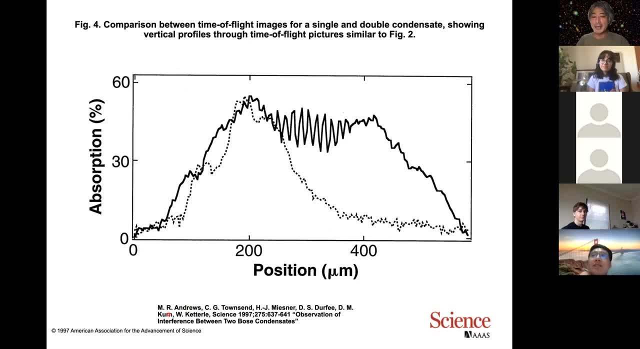 he was postdoc in that group So I kind of suspect it was he who made this observation possible. So you know too bad that he didn't share the Nobel Prize but anyway. So he contributed a lot to this experiment, as far as I know. So that's a way you might also 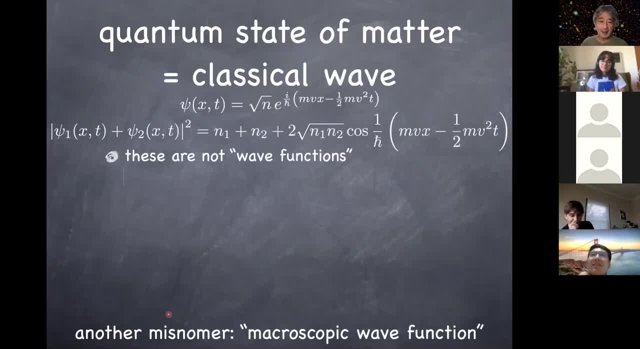 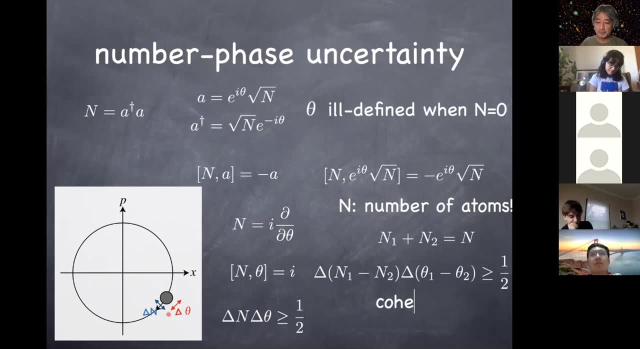 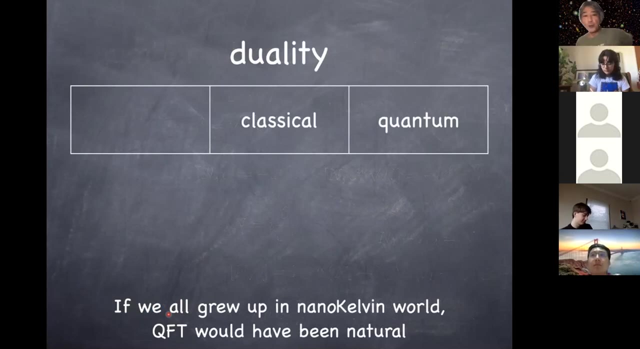 appreciate being in the physics department here in Berkeley. We got a lot of great people, So let me finish this up. Am i talking volume? So now just recap what we have done. So there's always this duality between wave and particle in quantum systems. 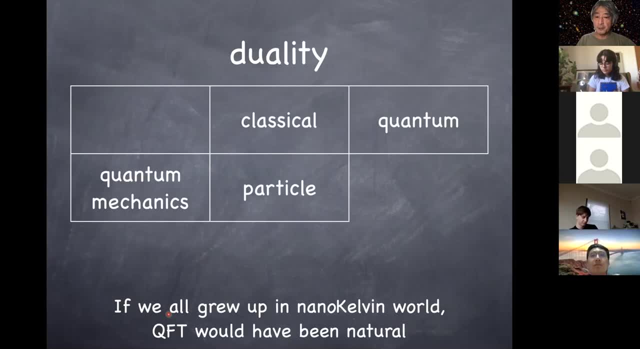 And what we used to do in quantum mechanics is treat particles as a classical objects. Then you say you quantize your Lagrangian Hamiltonian and get to quantum theory, where you see wave equation following the Schrodinger equation. So that's what you have done many, many times over. 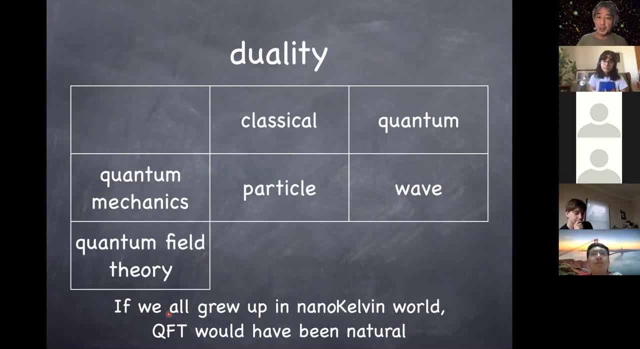 in quantum mechanics, class in 137.. What we are doing here is basically the opposite. In quantum field theory, you take the classical object, which is the wave- and wave is a function of space and time, hence a field- Then you quantize it. and whilst you're quantizing it, 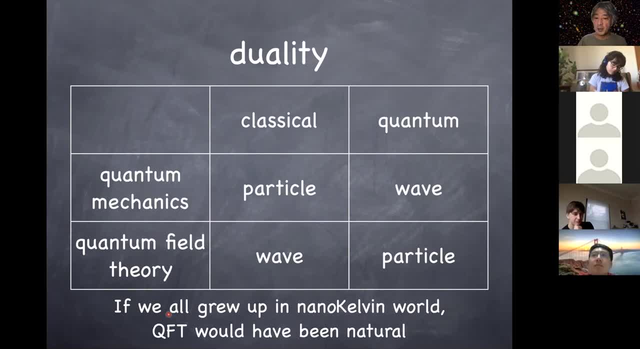 now, as you're doing the Cormorant problem, you get the multi-particle quantum mechanical states. So the role of particle and wave are the opposite, And the reason why doing quantum mechanics was the natural thing to do is because we perceive atoms as the tiny particles. 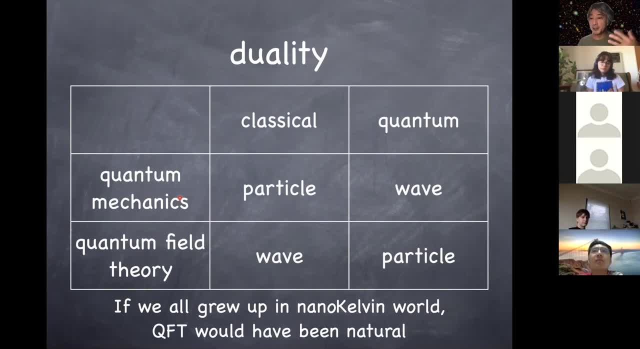 and that's something we can picture in our head. And then it's a surprise to us that those tiny particles actually behave like a wave, following the Schrodinger equation. So starting with the particles and going to wave later is kind of natural thing for us to do. 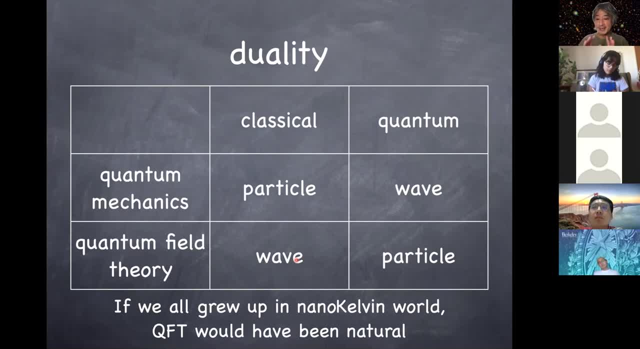 And starting the wave of this boson's geocondensate is definitely not a natural thing for us because you know, we haven't seen this until 1995.. So human beings have known this only for the last 25 years. But if you imagine a creature, 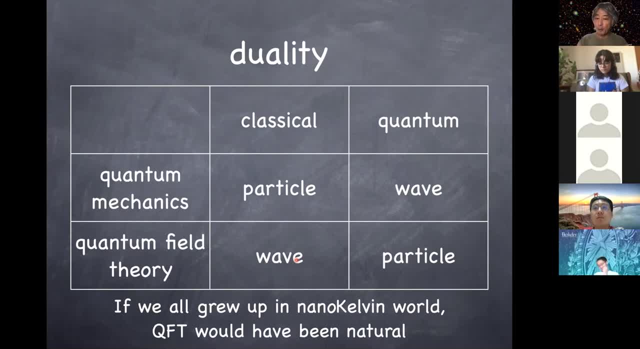 that is, living in nano Kelvin world, so you were born to that world. then everything around you is a boson, geocondensate, So you see these classical waves all the time. So if you do live in that kind of world, you'll be very surprised that once you actually going up. 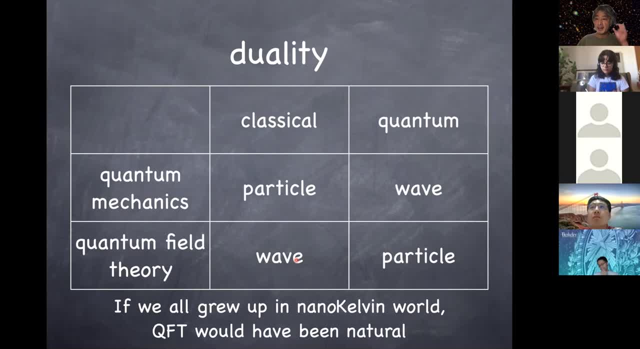 to higher temperature, higher energy. you're going to be surprised, Because without energy you can knock out individual particles out of this classical wave, right, You'll be very surprised to see that So you might be with the large Hadron collider. 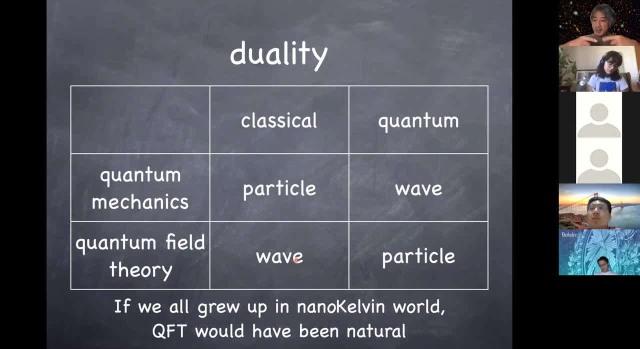 in this nano Kelvin world, inject enormous amount of energy into the collision point, then outcomes particles And you go what we only have known waves. So it just depends on your perspective in what kind of experience you have in a daily life, simply because we are much more used to particles in daily life. going from 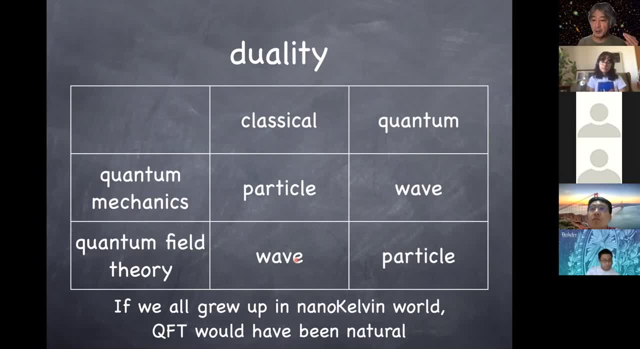 particle to wave was the first step we took when we start to talk about the quantum physics. But if you had lived in this imaginary world in nanokelvin, that everything around you is the classical waves because they are condensates, then finding a particle would be a huge surprise to you. And that's exactly what. 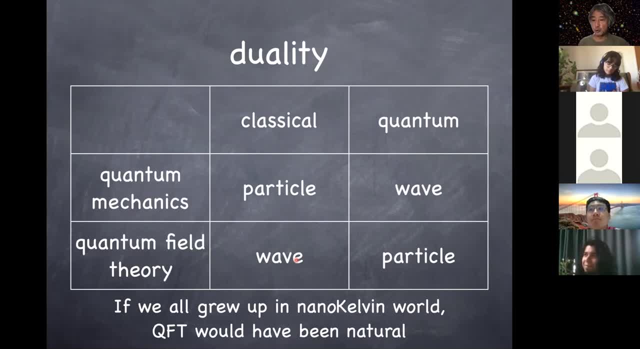 we do in quantum field theory. You start with a classical wave, you quantize it, then you find particles and then you are talking about again this particle-wave duality, just in the opposite order. So that's just a conceptual point to just to recap what we have done. Any questions about this? 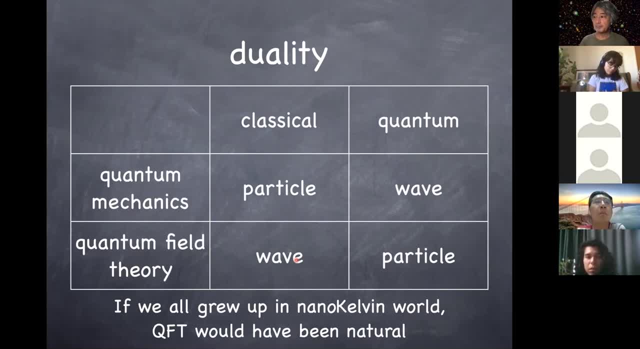 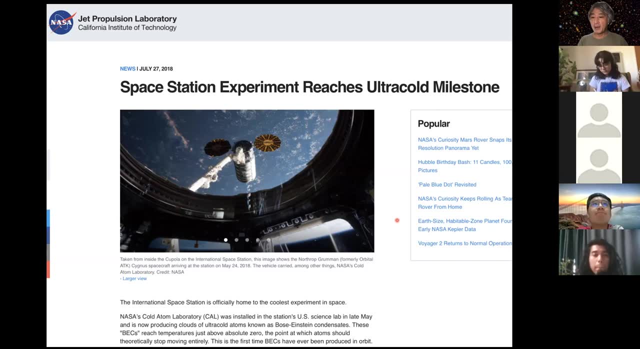 idea: Everything okay, All right. And one thing actually I learned recently is that the International Space Station actually has a lab that produces the boson-zhengan condensate in zero-gravity environment, And the reason why I want to do this is that, let's say, you do make this. 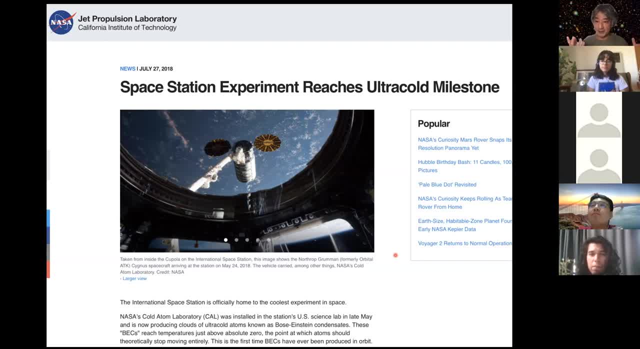 boson-zhengan condensate. that takes a lot of work with a lot of technology, but once you actually release it, then what happens is that it just drops because there's gravity. These atoms are moving so slowly that gravity is just enough to. 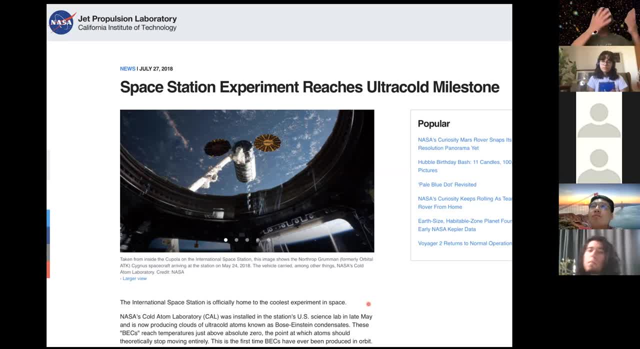 pull them down. In normal life, when I have the air around us, it's made of tiny molecules, as you all know, and they are not dropping to the bottom of the room, right? And do you know why that is? Any volunteers? Why don't all the air molecules drop on the floor? 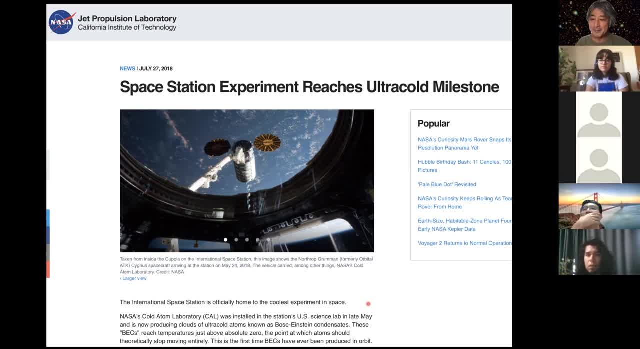 It's thermal energy. Good, That's exactly right. So we live in a high-temperature space. So every molecules are moving because of the thermal energies dictated by the equipartition theorem, And that speed or kinetic energy is far, far bigger compared to the gravitational potential energy. So half mv squared is much. 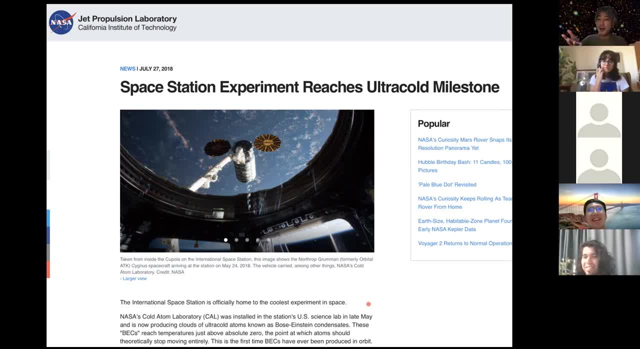 much bigger than mgh. That's why you can breathe Air. it can come into your lungs, and otherwise you'll be all dead by now. So that's why air molecules don't drop on the floor, But once you go to this, 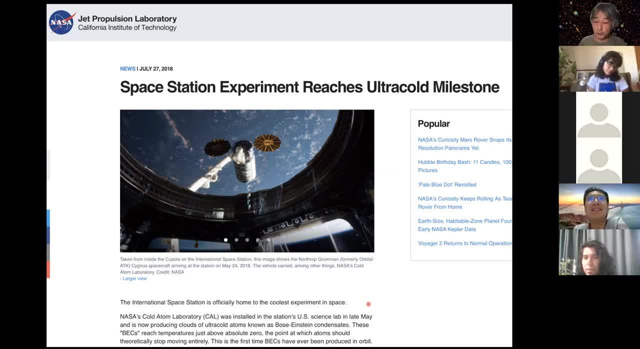 nanokelvin temperature that each particle is moving so slowly the boson shunt, condensate just starts to drop. So precious condensate you worked so hard to produce will be lost. But in zero-gravity environment it just stays there and you. 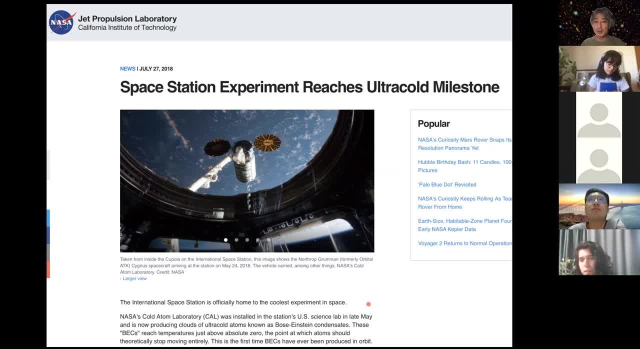 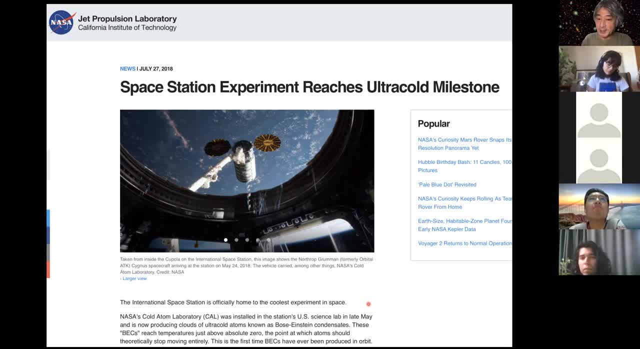 But you still have to come up with a way of cooling the gas of atoms to nanokelvin temperature. And because NASA is doing this on the International Space Station, they produce really cool video to tell you how they actually cool the gas of atoms down to this incredibly low temperature. 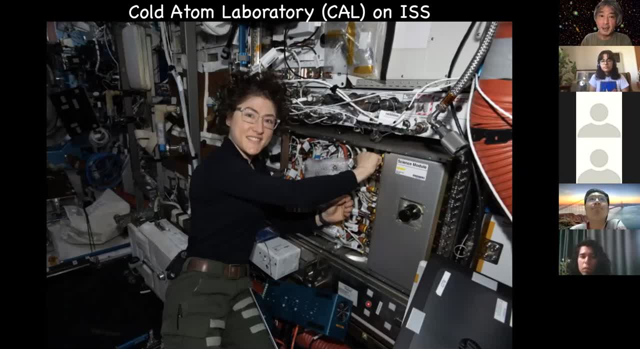 of nanokelvin. So this is the picture of this, what they call the cold atom laboratory, short CAL C-A-L. So this is the picture of this, what they call the cold atom laboratory, short CAL C-A-L. 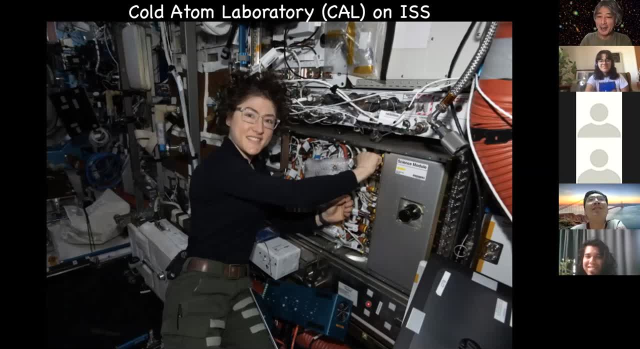 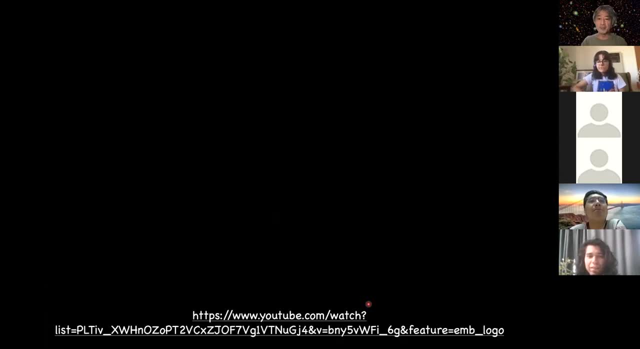 Kind of confusing for us, right, You know, go bears. Anyway, this is the cold atom laboratory sitting right on the International Space Station, and this is what they do: to cool the system down to the temperature instrument. Jeremiah–Yong refining labor. 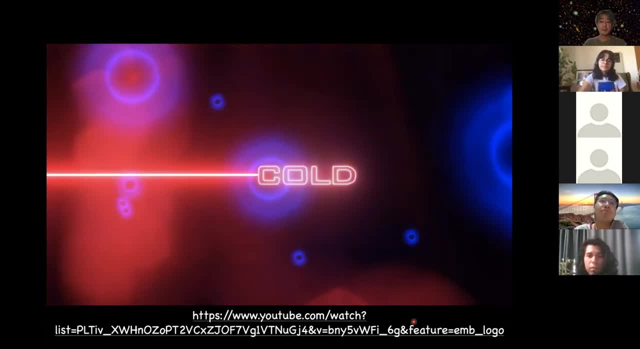 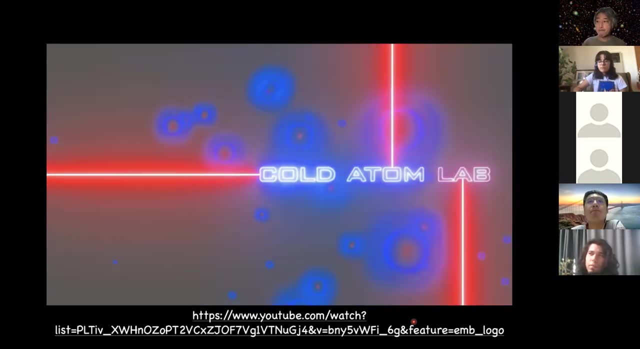 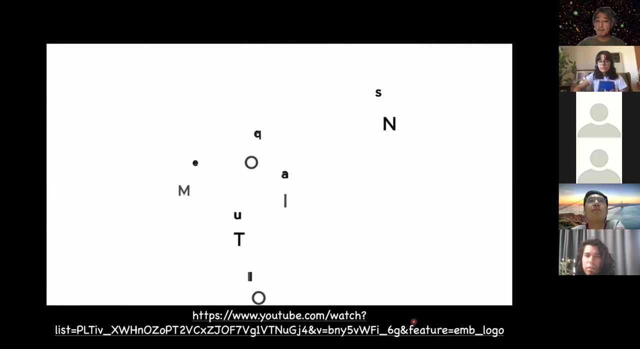 That's kind of crazy. Can they hear the sound? You think that you make something cold by shining light on it. Normally we think about shining light on something and making it hot. Laser cooling does something quite counterintuitive: It makes something cold by shining light on it. 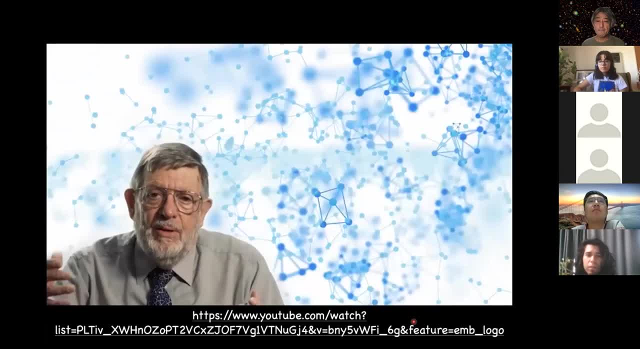 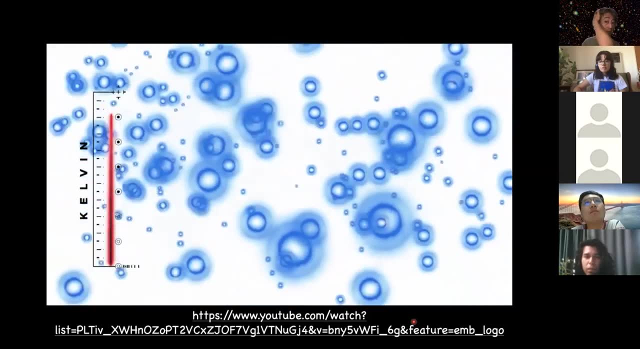 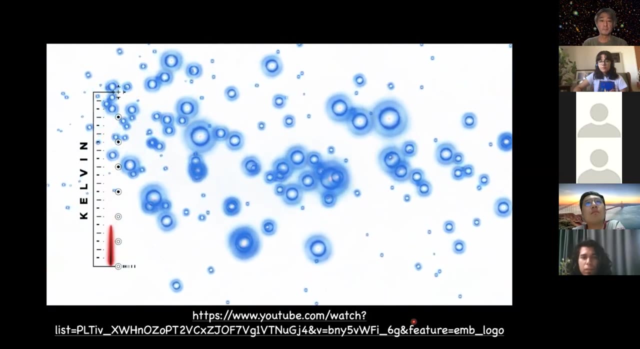 Temperature is about motion. The molecules in the air in this room are moving really fast, about 300 meters per second. If you cool down a gas, you're making the atoms and molecules move more slowly and getting to the lowest possible temperatures. That's the extreme that we're trying to go to. on Cal, 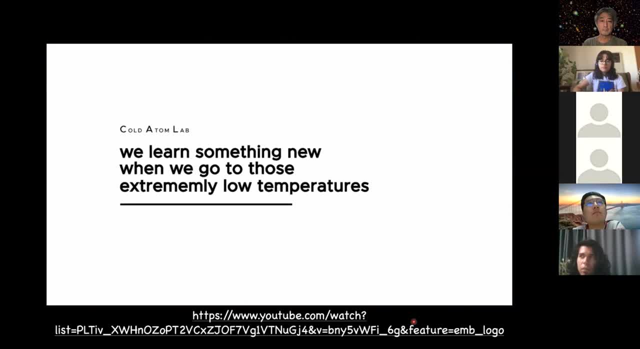 and we learn something new when we go to those extremely low temperatures. We start with atoms that are actually room temperature, even a little bit hotter than room temperature. We just have a vapor of them in a glass cell where we use the radiation pressure from lasers to slow down atoms. 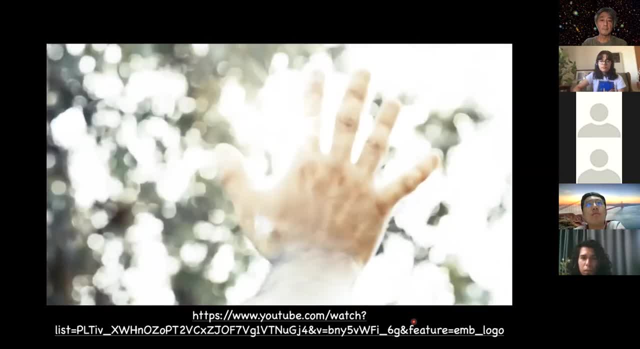 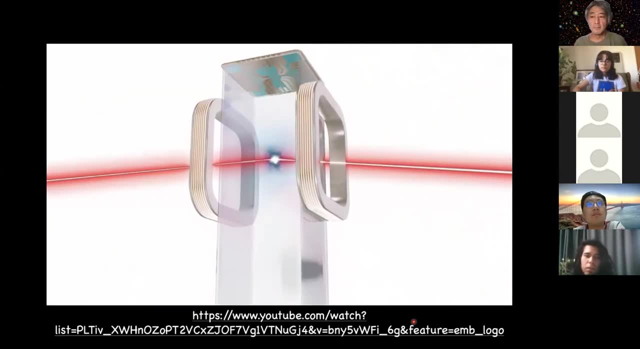 As it turns out, light pushes on stuff. We don't feel it when we walk out in the sunlight, But for something as light as an atom, the push that you can exert by shining light on the atom- in our case laser light- can be really significant. 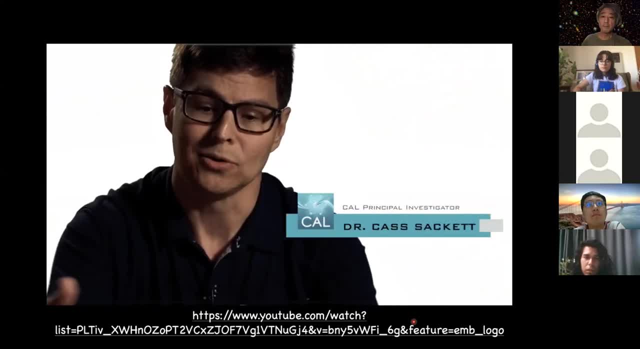 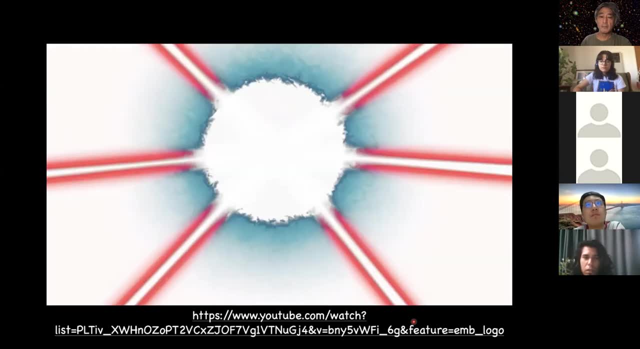 We don't actually use two lasers, We actually use six. So there's two this way, two vertical, two in and out, And so no matter which way the atom's moving, it's always moving towards one of the lasers and that causes it to slow down and cools them down. 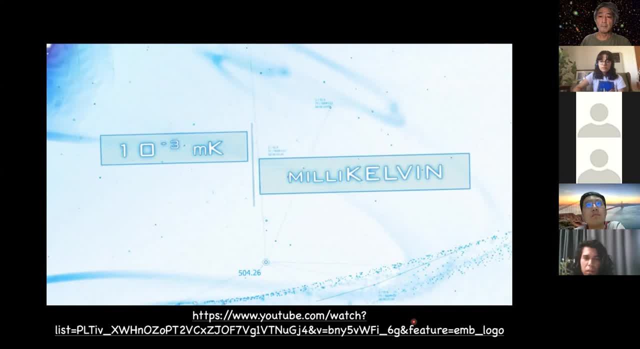 to 1,000th of a degree above absolute zero, But eventually, to get to the temperatures that we need for Cal, we actually have to turn off the lasers, And what we do is we move the atoms so that they're held by magnetic forces. 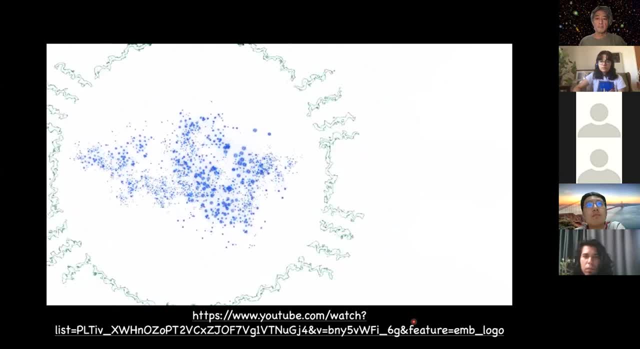 And what we can do now is we can just like turn off the lasers And we can just adjust the magnetic field so that this trap that they're held in is not very deep, So we can make it so that the most energetic atoms just have enough energy to just move off and escape. when they fly away, We can actually pull out just the hot atoms, leaving the rest of them at a colder temperature. This is called evaporative cooling. It's essentially the same as when you blow on your coffee. 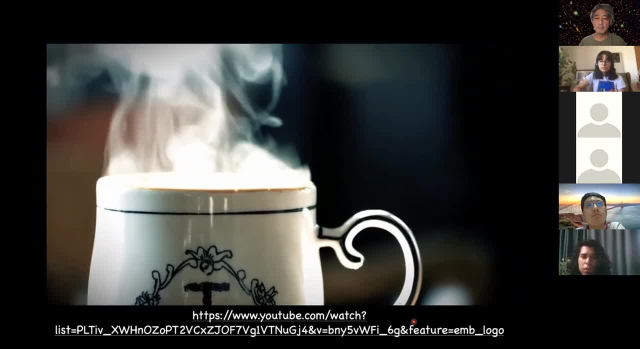 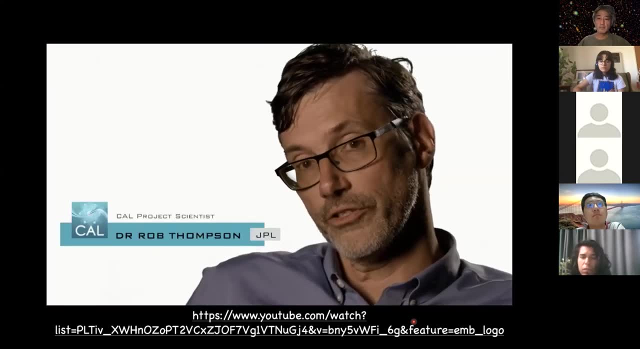 cup. The hottest molecules make it out of the water And if you can constantly be blowing those away, you can cool down your coffee And that gets us all the way down. It gets us all the way down to these temperatures of micro Kelvin, a millionth of a degree above absolute zero. But it turns out you can get even colder by using another really old trick called adiabatic expansion. If you take any gas and you expand it, it'll get colder. So we're doing the same thing on a sort of small scale. 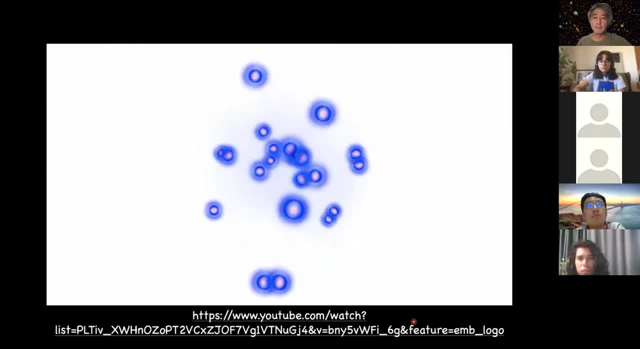 We have this little, small sample of atoms that are confined by magnetic fields, And what we're doing is we're reducing the strength of that magnetic field, which lets the atoms expand out. It's something like a factor of 1,000, which 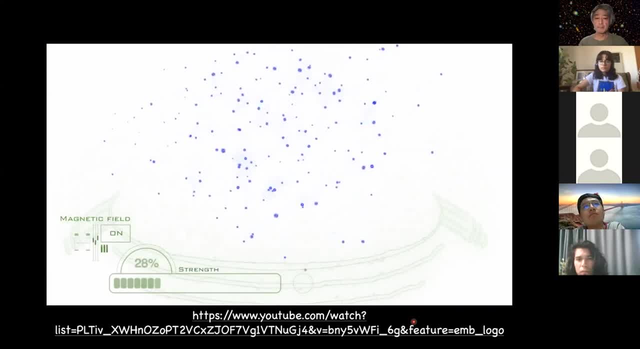 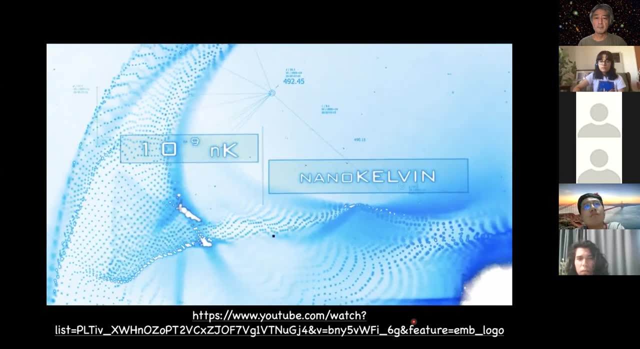 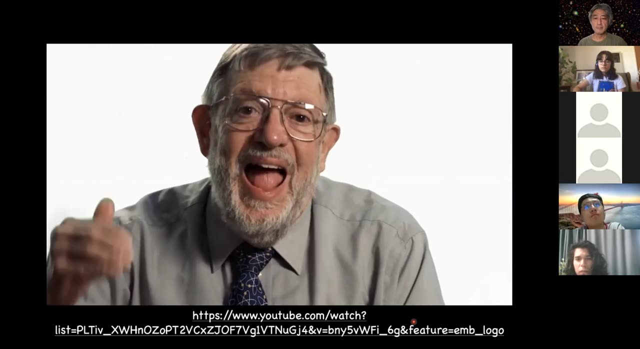 causes them to cool off by a factor of 1,000. This trick works so well. We get down to temperatures below 1 nanotel, 1 billionth of a degree above absolute zero, And it's being done on the cold atom laboratory every day. 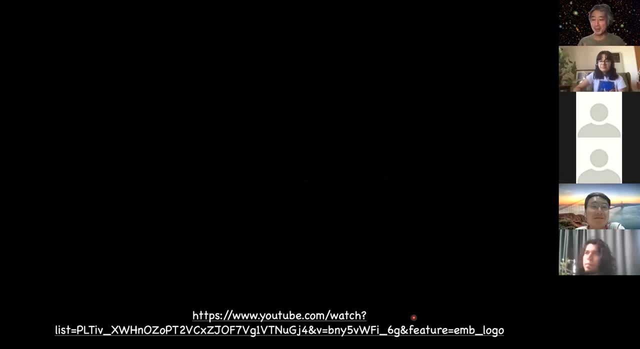 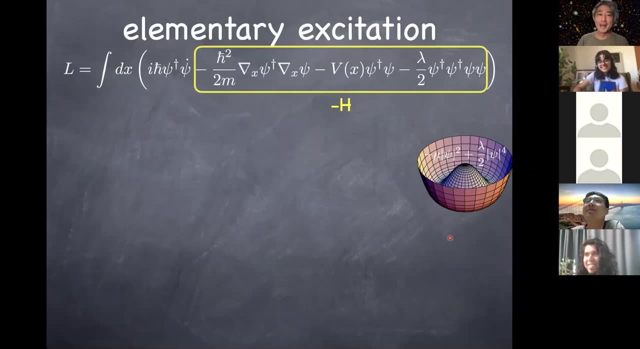 Isn't that cool. So one thing: I realized that now we are stuck with this online teaching, I can show videos which I can't do in the classroom, So there are some benefits to that. So this idea that the cold atoms start to behave like a classical wave, I 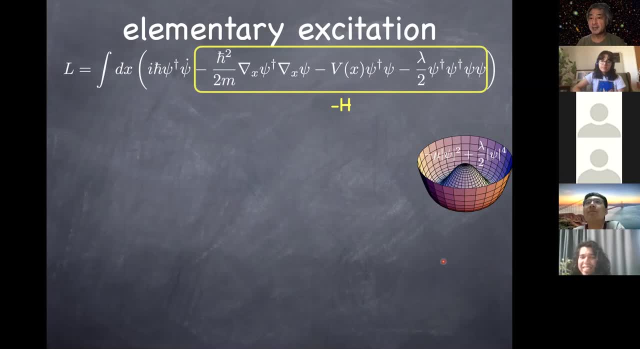 hope that started to sink into your mind now. But we can test this idea much more rigorously and quantitatively, And the way you do it is look for something called elementary excitations. So once you have a system which is very cold, 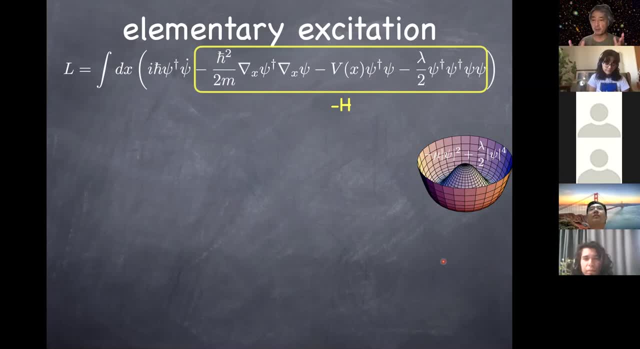 the next question you always ask: which is true in condense matter physics, particle physics, nuclear physics, in any of these systems you ask the questions: what are the possible excited states above the ground state you got And the way you answer this question in quantum mechanics. 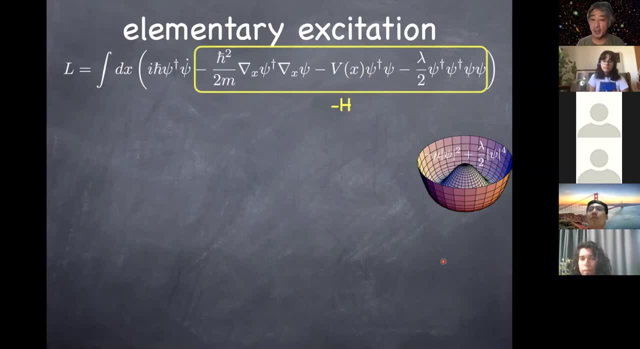 is that you solve for the energy eigenstate Schrodinger equation and first build a ground state and ask the question: what is the next excited state? and so on and so forth. But now that we have the description of the system using a classical field, 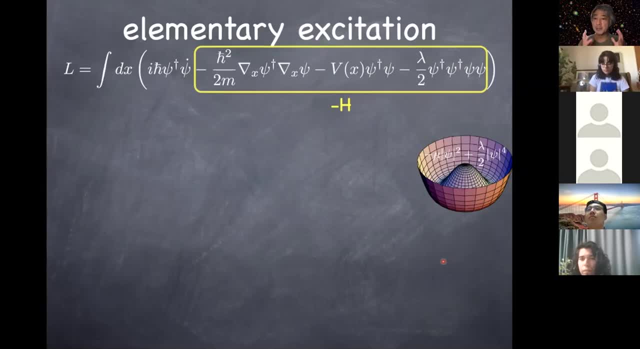 The way you can answer this question is a lot simpler, it turns out. So all you do is again go back to the basics. We have this chemical potential, We have this energy gain for adding additional particle And we have this Euler-Lagrange equation. 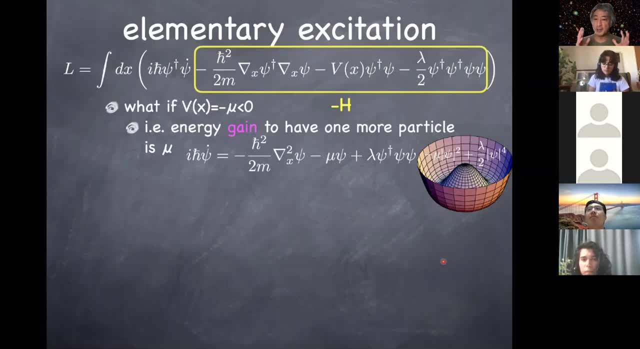 So, because classical physics is all dictated by the equation of motion, it should be same here, Now that we have this classical Euler-Lagrange equation, that should be able to tell us everything we want to know. So how do we go about actually studying it? 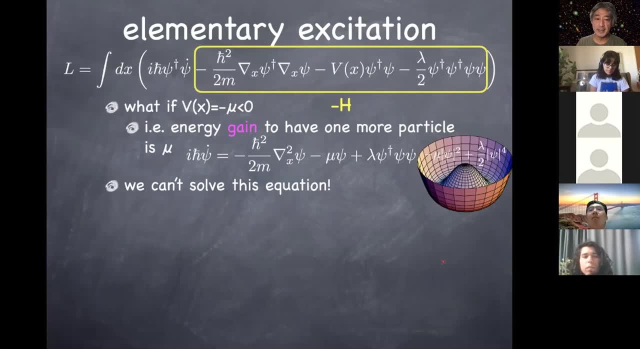 Again, we're facing this problem that we can't solve this equation exactly, but we do have a solution we'd like to start with. So the quantum analogy is that this would be basically the ground state, and now you're looking for the excited state. 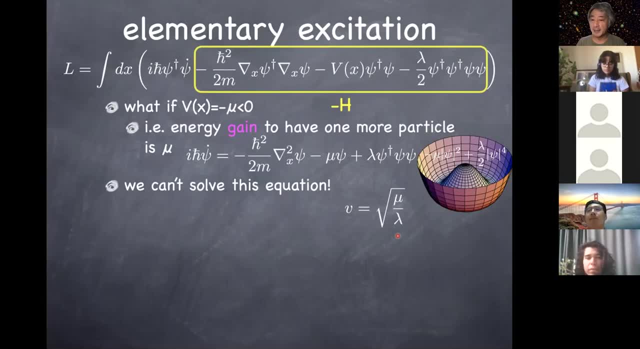 on top of it. The way you answer this question classically is that: okay, this is a solution, exact solution, to the classical field equation. So you look at it, but the small fluctuations around it- And this is the kind of analysis you do all the time- 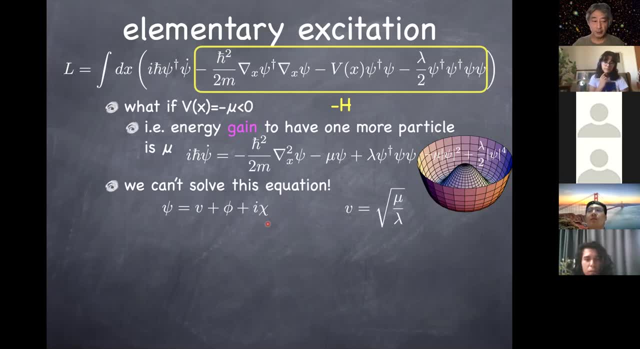 in electromagnetism These days. of course you are, I'm sure you know that we can detect gravitational waves, and this is the way we analyze gravitational waves too. So you have some kind of complicated nonlinear field equation, but you first find a solution. 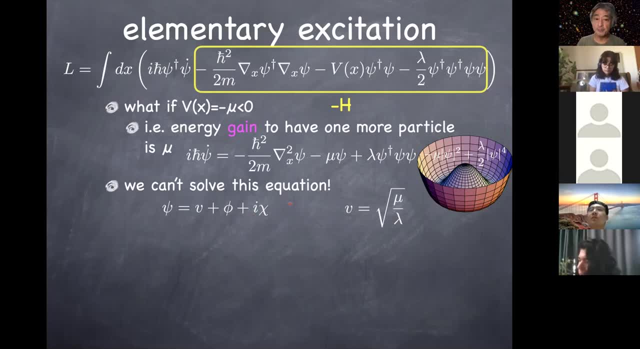 then you perturb around that solution and look at just the first order in this perturbation or fluctuation, And this is the process called linearization. So when you actually expand Psi, which is a complex field, around this one solution V, which is the constant, 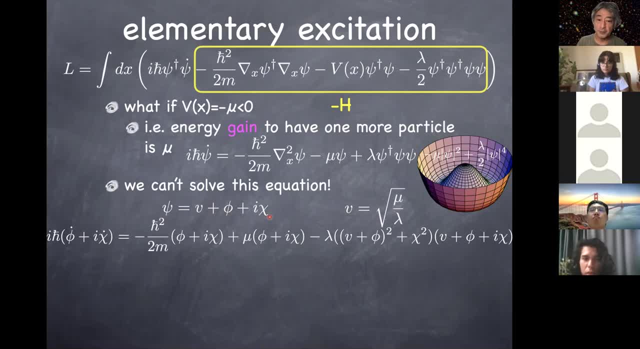 then you need to introduce fluctuation both in the real part of the field and imaginary part of the field. And I apologize, I changed the notation from lecture notes. Eventually I'm gonna edit the lecture notes to conform to the same notation later on. 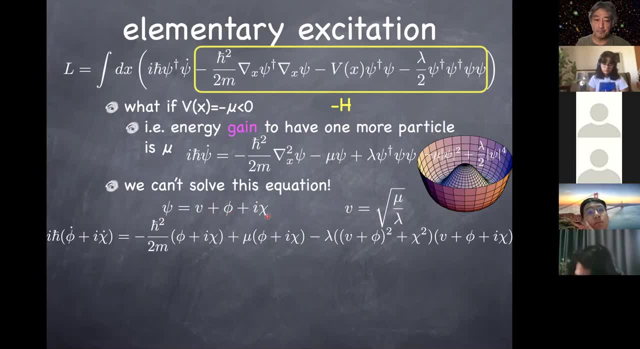 So Phi is the real part, Chi is the imaginary part. I just stick this into the O Edge equation and I find this. So this is still not something I can solve on general grounds But, as I mentioned, like what we do in electromagnetism or general relativity. 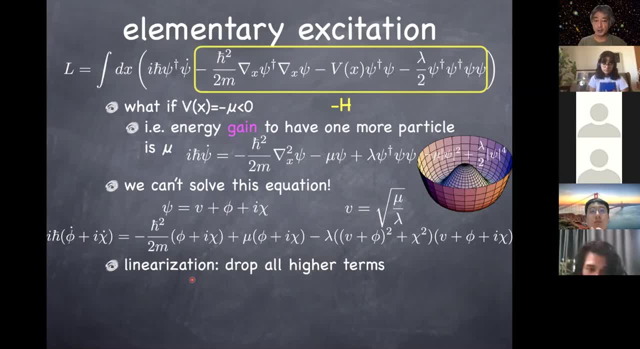 we do linearization of the equation of motion, which is just a fancy way of saying that we only keep the first order terms and drop all the other high order terms. And that is justified when Phi and Chi on theavait off the direction of traffic are equal. if these two Equations are equal, each other are equal, and provisionally복. 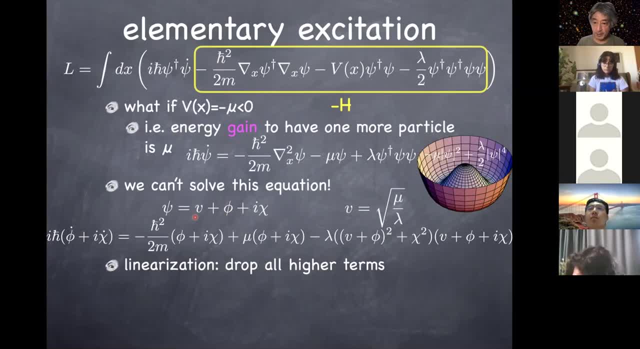 very small compared to V, and once you do so, this equation becomes drastically simpler and equation as a whole has both real parts and imaginary parts. so I separate real parts, imaginary parts, keeping only the first order terms in Phi and Chi, and that's how you end up with these two equations. now you can see. 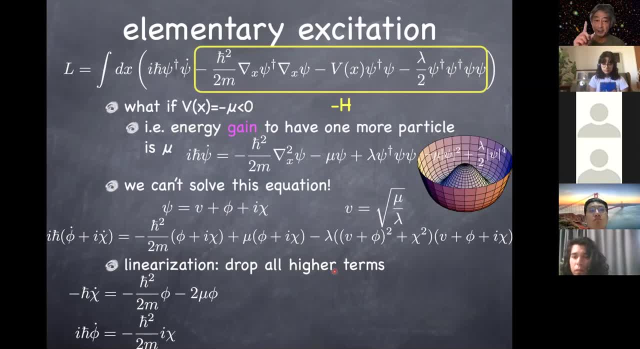 this is very simple. in addition, if you take another time derivative of this equation, Phi double dot, is then given by Chi dot. but we know Chi dot given equals Phi. so I have a second-order differential equation with Phi. only I can eliminate Chi. then you sort of see what you get. so this is Phi. 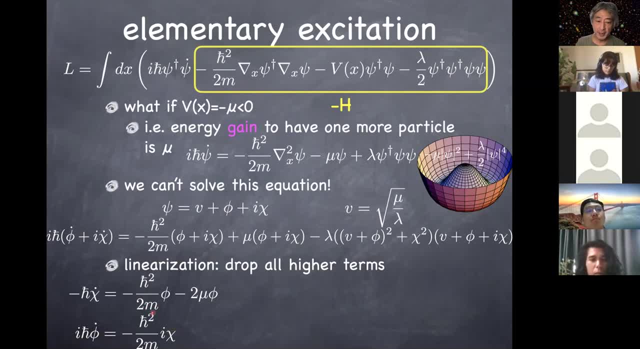 double dot over here and this is Chi dot. you can eliminate Chi by eliminating Chi. then you sort of see what you get. so this is Phi double dot over here and this is Chi dot. and and using this equation I get h bar squared over 2m twice. and I apologize, I made a mistake that. 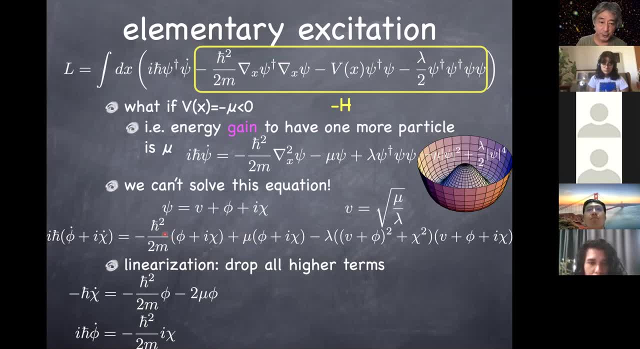 I dropped the spatial derivative here, so I'm going to fix this in lecture notes. so this is spatial derivative squared acting on it. so this is spatial derivative squared acting on here. spatial derivative squared acting also on here. so this is h bar squared spatial derivative squared. 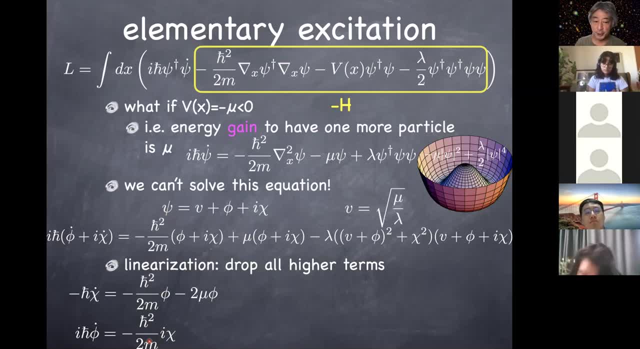 over 2m, which you recognize as the form of the kinetic energy. and then chi is rewritten now by this so big parentheses: kinetic energy, phi minus 2 mu phi in there. so as a result, you know the dispersion relation, namely the relationship between wave vector and angular frequency, or by: 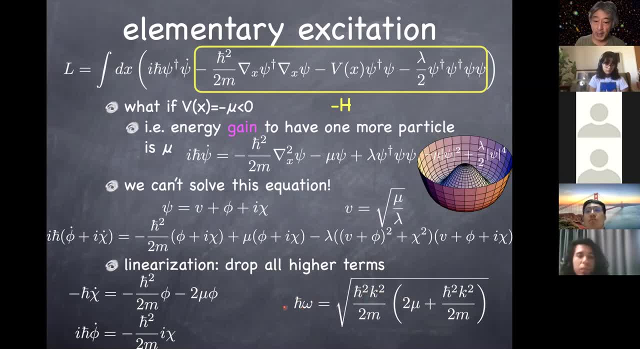 using h bar, momentum and energy. so now I expressed energy as a function of the momentum just by solving this classical Euler-Lagrange equation. so this is what we call the Bogolubov spectrum, namely that energy of the excitation is given in terms of the momentum of the excitation. 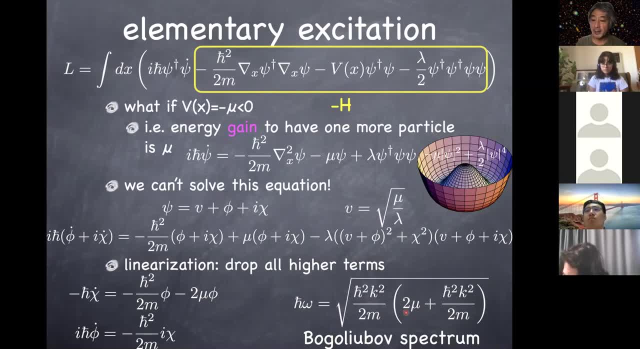 and, as you can see, when you send chemical potential to zero, then you can ignore this. this is square of the kinetic energy, p squared over 2m, and then square root. so it's nothing but energy being p squared over 2m. 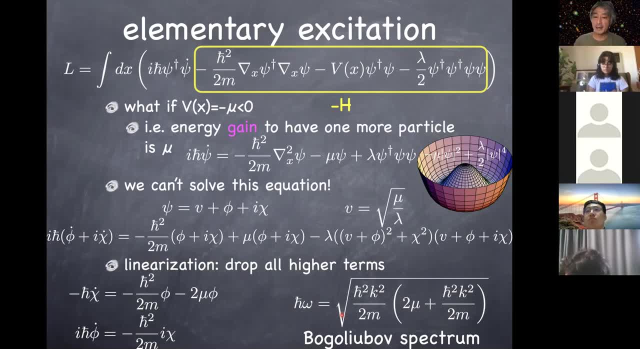 and that's what you would expect, right? On the other hand, when momentum is small compared to the size of the chemical potential, then you can ignore this term instead second term in parentheses. so what you have is something that looks like k squared times, mu squared root. 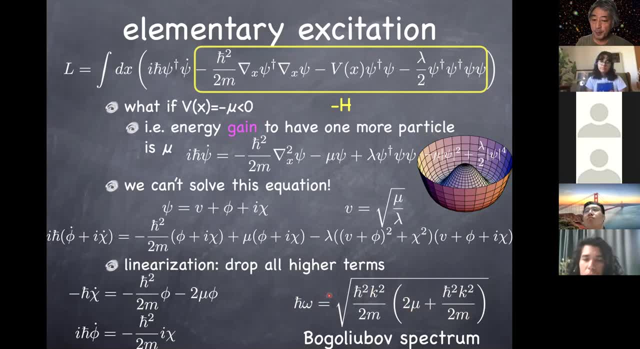 so after taking square root, this term will be proportional to k, so that's linear in momentum and that actually turns out to be very important later on. So anyway, so this is the problem. Okay, so let me pause here. if there are any questions about how you go about and just solve this equation. 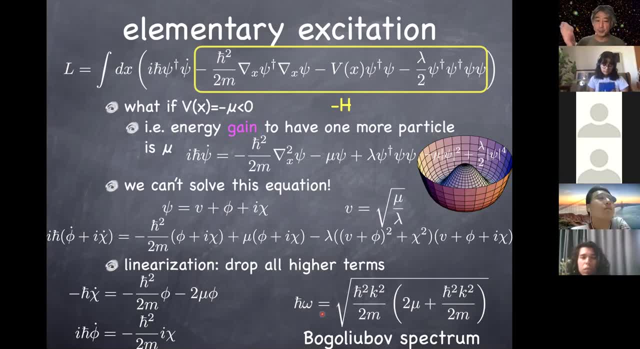 simply by dropping all the high-order terms which comes with this fancy name of linearization. Any questions about that? I might have missed this. but is this dispersion relation just obtained by solving the two differential equations and, you know, by taking the second derivative of phi? 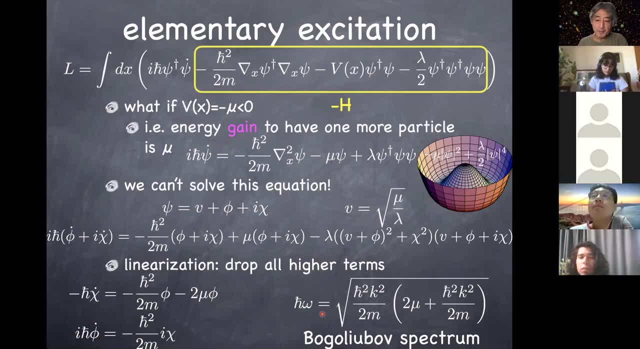 That's right, that's right, yep. So where does, Where does the, I guess the omega get introduced in h-bar? So omega is the angular frequency. so once you write phi in the form of the plane, wave e to the minus i, omega, t and e to the i, k, x, this phi double dot will pull out omega squared. 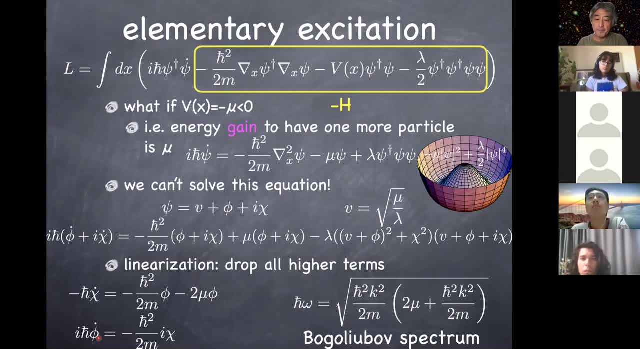 I see. so there's a trial, a trial like standard plane wave solution. That's right. right Makes sense. So, because we did this linearization, the equation is linear, so you expect to have plane wave-like solutions And that's what you use as an ansatz. 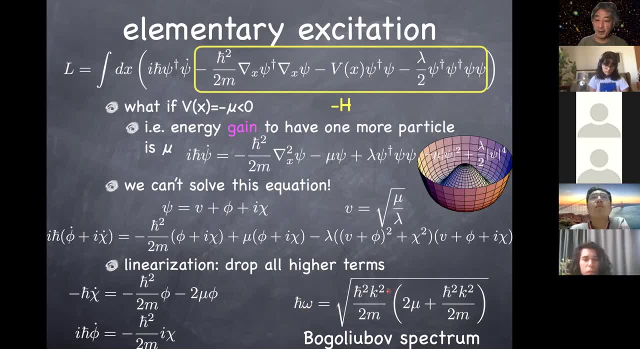 And as long as angular frequency and the wave vector satisfy this relationship, you do find the plane wave solution. Okay, does that answer your question? Yeah, thank you. Okay, any other questions here? Yes, may I ask a question? Go ahead. 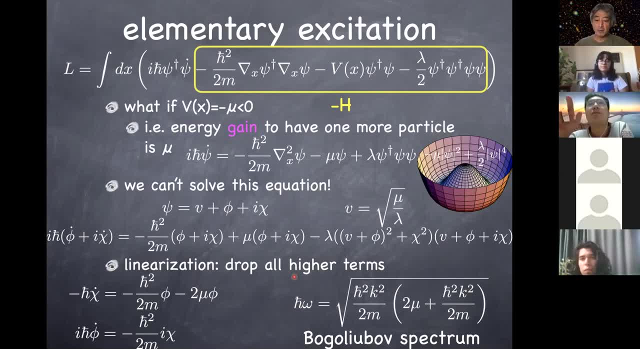 Yeah, so the Euler-Lagrange equation is the equation for psi and psi is the, the annihilation operator, right, Right. But you assume like psi equals v plus phi, plus i, chi and Mm-hmm, v is free on those that were like real numbers. 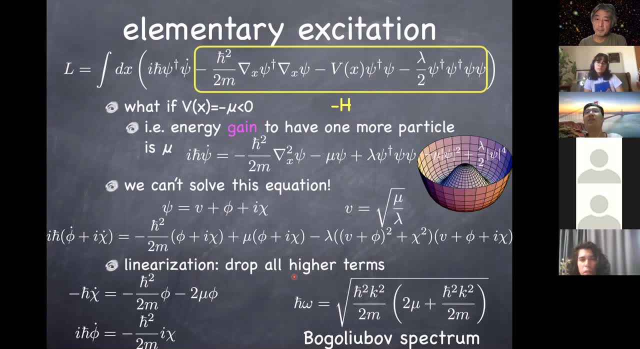 So are you assuming, like the low-energy excitation is still an eigenstate of the psi, Because otherwise you're using a number to represent the operator? That's an excellent question And you know the analysis using classical field theory is actually. 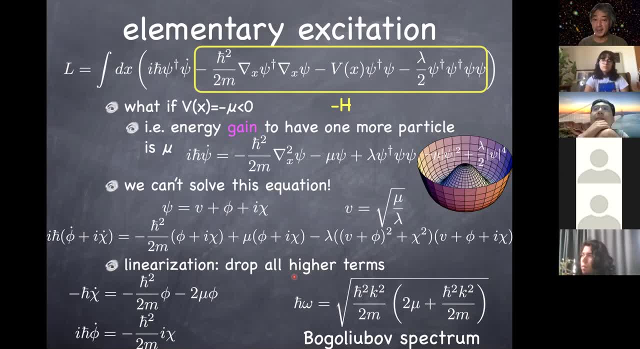 I mean it's a little bit more complicated than you think, but it's a little bit easier than you think. It's a little bit easier than you think. but if you ask the question, you just asked how that is actually shown in terms of Hilbert space and operators. it's a lot more complicated. 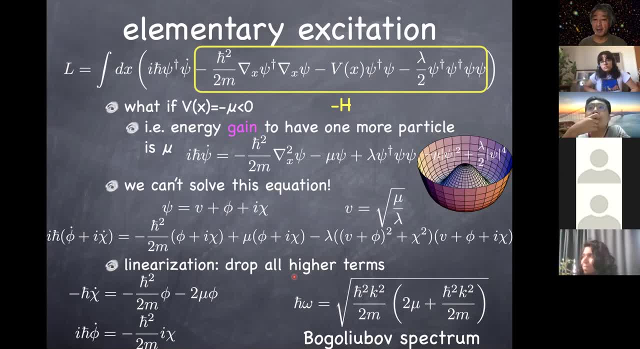 And I actually I don't intend to go through this in class, but if you look at the lecture notes of bosonpdf, you'll find something called Bogoliubov transformation. So you first take the coherent state as the ground state of the system. as I told you already, 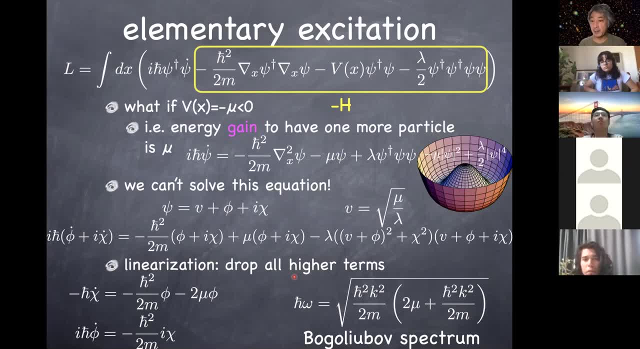 And what would be the excitations around that ground state. And then you write down the Hamiltonian which includes this interaction term. So again, you cannot solve it exactly, So you try to solve it approximately. And the way you do it approximately is looking at this Hamiltonian. 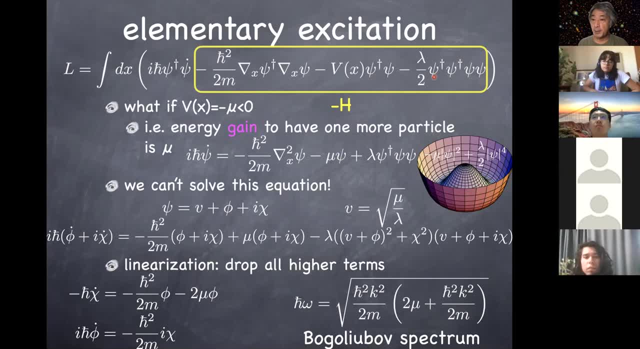 You insert coherent state, namely constant psi, into two out of these psi- diagonal psi- And keep the other two as operators. And that is actually the same idea as the linearization for the equation of motion, Because if you only retain terms that are quadratic in psi, m, psi, dagger. 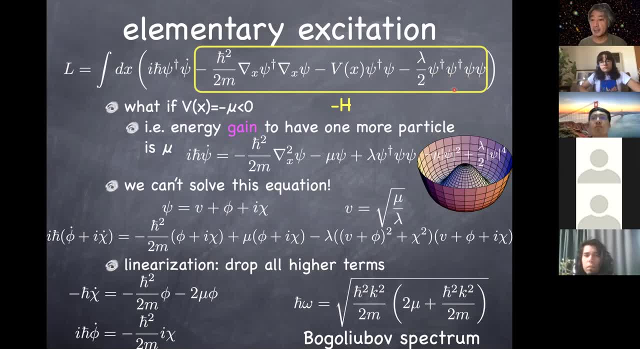 the corresponding Euler-Lagrange equation would be linear. But now using this language you can deal with the operators. So you have Hamiltonian written as an operator. Then you keep only quadratic pieces in operators- psi, m, psi, dagger- but replace the rest by the eigenvalue in the coherent state. 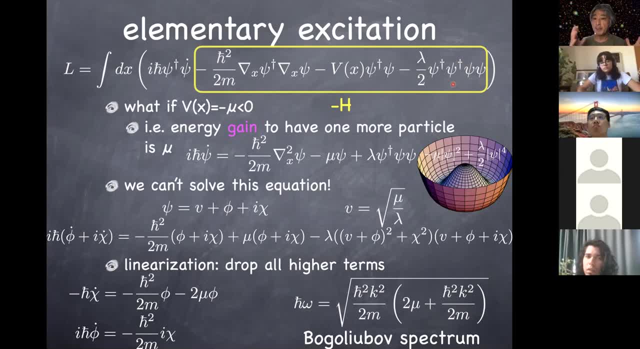 So then you have a quadratic Hamiltonian, But that Hamiltonian looks very weird. So this part is good. This is basically a dagger a creationization operators, a dagger a so far, so good. But if you replace two psi daggers by number, 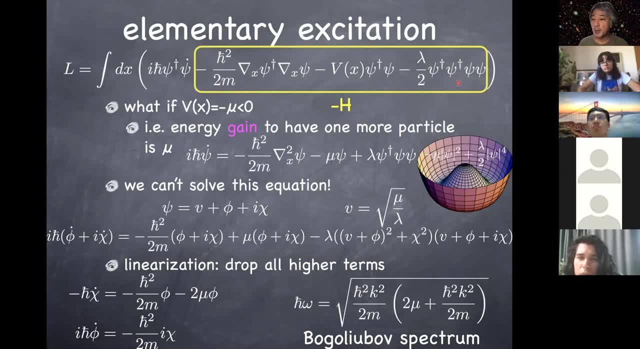 and keep two psi's in it, you have a term in Hamiltonian that looks like a, a, not a dagger, a. You also have a term a dagger, a dagger, if you replace psi by numbers. So you have this weird Hamiltonian. 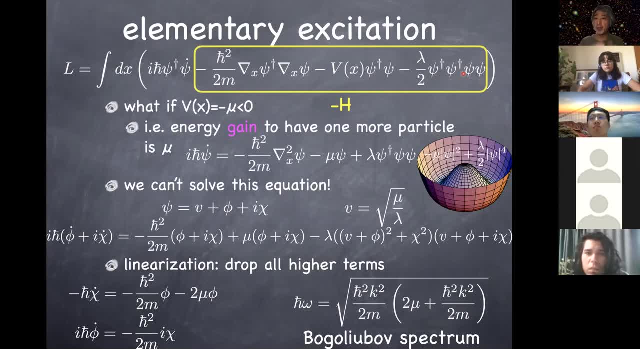 which is quadratic, in a, an, a dagger. but in addition to a, dagger, a terms we're used to, you also have a a in a dagger, a dagger terms in it. But within this approximation you can still diagonalize the Hamiltonian by doing this Bogo-Brugov transformation, where again this is: 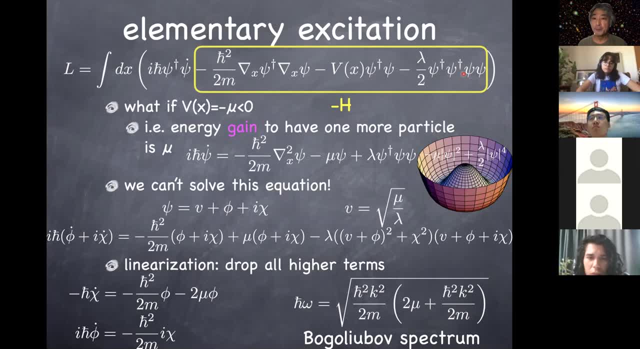 weird. you take linear combination of creation operator and annihilation operator. Then you can diagonalize Hamiltonian And that sounds totally crazy because creation operator increases the number, annihilation operator decreases the number. What the heck does it mean to take linear superpositions of them? But now that we are dealing with a coherent state where number 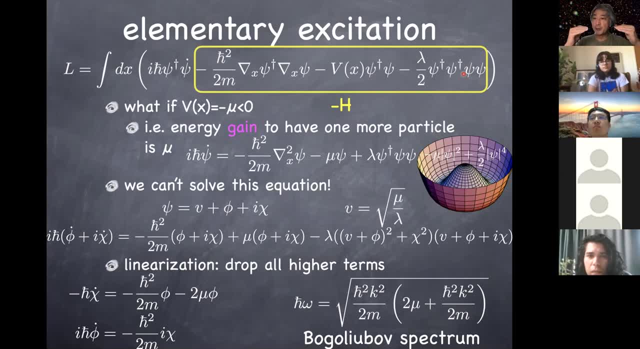 is uncertain. the state you start out with, for the ground state, has some distribution in numbers already. So, starting from this state, creation and annihilation can lead to the same state at the end of the day. So that's the weird thing we have to do, which is far more technical than what I do. 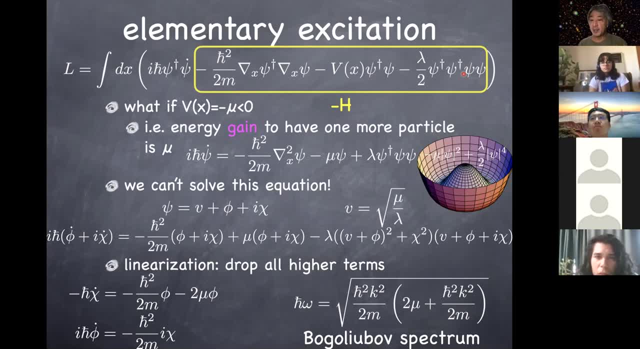 on the slides, but you can do that. You indeed arrive at exactly the same answer at the end of the day of this Bogo-Brugov spectrum. So one advantage you see in this exercise is that looking at the classical field equation is a lot easier than dealing with operators and trying to diagnose the Hamiltonian. 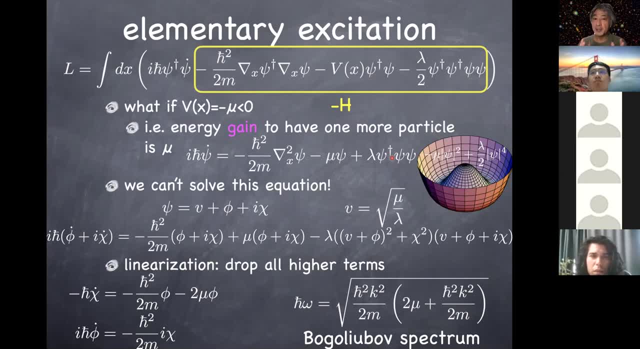 but you get the same answer, And that's the advantage of looking at this Boltz-Einstein condensate as a limit of classical wave coming out of Q, which justifies this very simple analysis you can do on a single page of paper to obtain this non-trivial result. 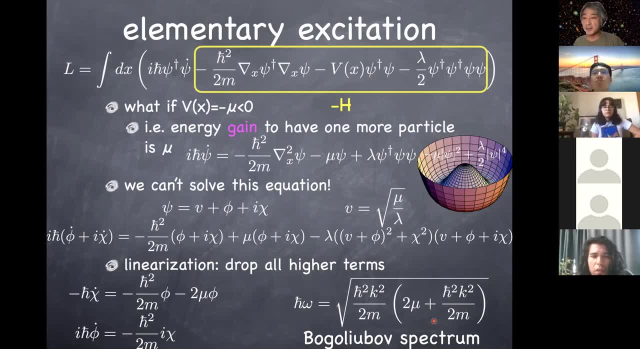 of the Bogo-Brugov spectrum. So that was an excellent question, Ryan, And did I answer your question? I think, if I understand right, you just said we start from a coherent state so we can assume, like psi, m, psi, dagger, to be a number. Then you just like perturb it a little bit. 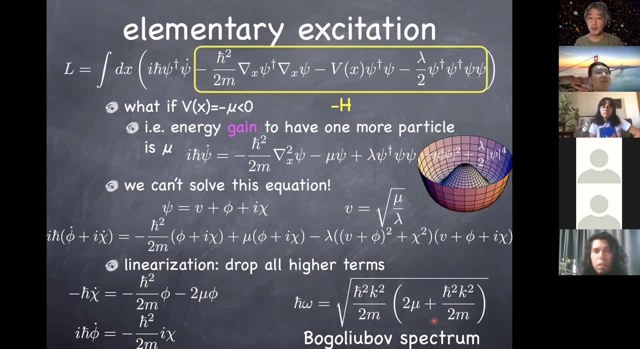 And the perturbation should be also enough. Okay, okay, That's right, Thank you, And is Reggie here? Maybe you want to actually discuss this Bogo-Brugov transformation next Tuesday in the discussion section. Yeah, that sounds good. 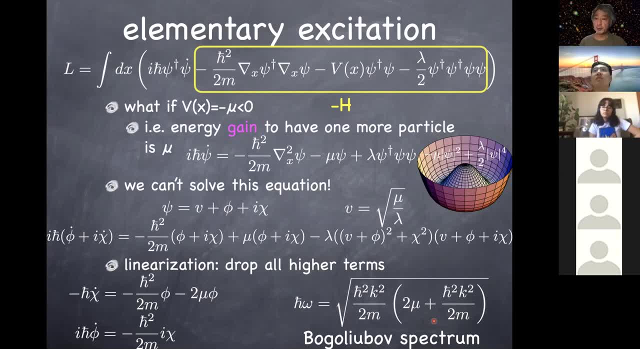 Okay, that'll be great, So don't miss that. So you see that in action, how you actually use operators and do this bizarre linear combination between creation and relation operators to end up with the same result on this Bogo-Brugov spectrum in the. 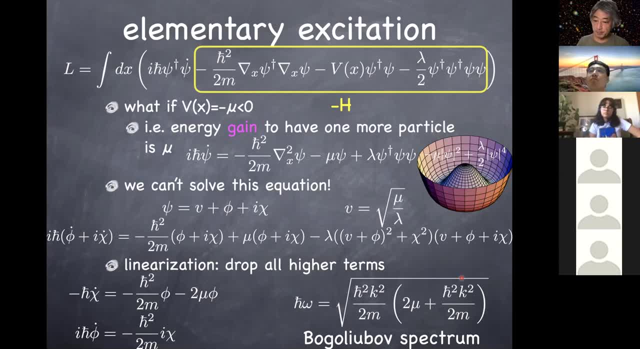 discussion section. Okay, so this is the prediction, And just spend a minute to observe this again Once you start with the Hamiltonian. of course, I made an approximation of the linearization, but there's no ambiguity in the entire process. This is an inescapable 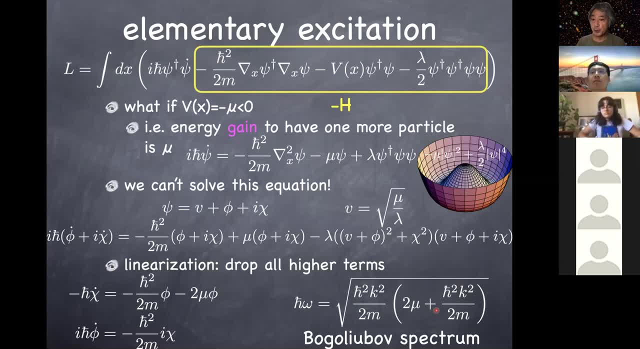 prediction of this field theory. So whether your experimental result really shows this relationship between the energy and momentum of the excitation would be a very, very non trivial test. There's no wiggle room. This is the prediction, And then we confront the data. 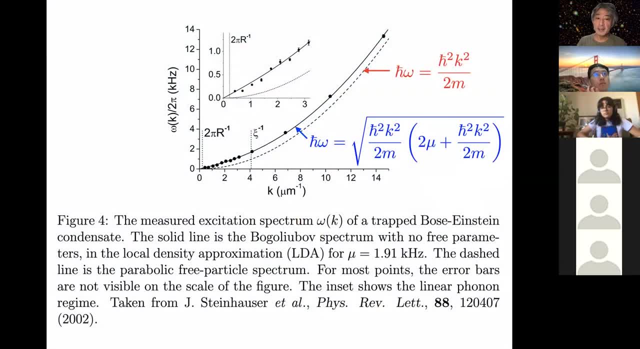 And that's what people did in the end. And here's the data. This is the wave vector. So if you multiply h bar on top of it, that's the momentum. This is the angular frequency. So if you multiply h bar on top of it, that's the energy. And they are supposed to satisfy this Bogo-Brugov spectrum. 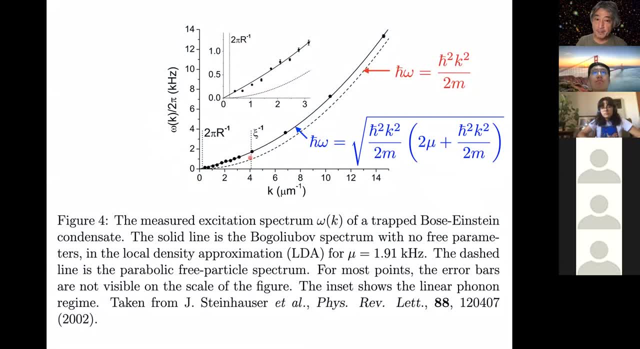 so that's the psychologists and you know, you can see here it's a very, very small p-type of a relationship And that's the solid line And black dots are the data. They're right on. Let me emphasize again, there's no wiggle room. You know the mass of the atom, The 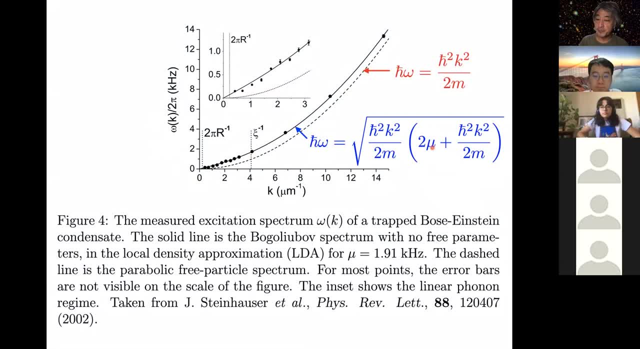 the. the only thing you don't know is the chemical potential, But in principle you can predict that too. So chemical potential is related to the density by this delta function potential lambda, And that's something you can measure too by doing a scattering experiment. 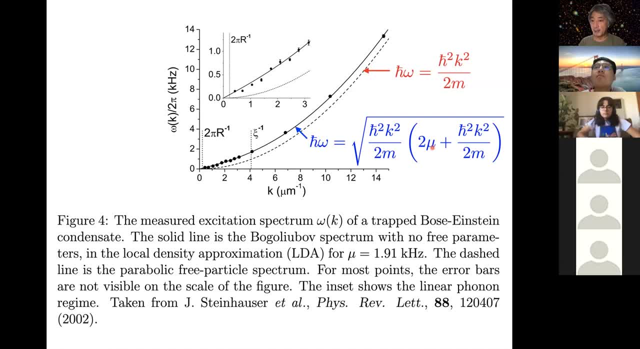 What is the strength of the repulsive force between the atoms. So once you fix that from measurement, and once you know the number, density, you can work out what mu has to be. Then there is zero parameter in this game And that zero parameter prediction. 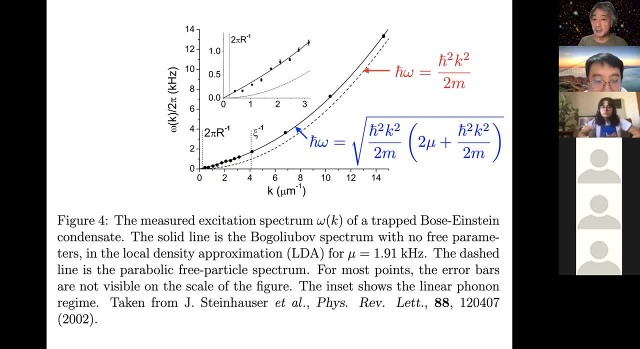 is completely consistent with the data points over this rather long range of the wave vectors. So this is a very rigorous quantitative test that the field theory language we developed to study boson-Shinkansen state really works. So let me pause here and see if there 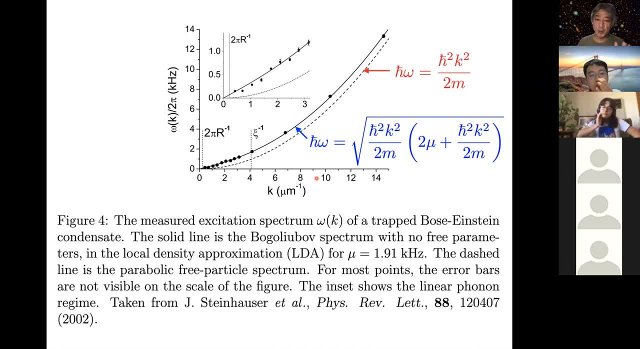 are any questions about this Or just in case you want to know, this was done by Raman scattering, basically by injecting a photon and see how photon gets scattered with different energy and momentum. at the end of the day, You can compute what is the energy momentum. 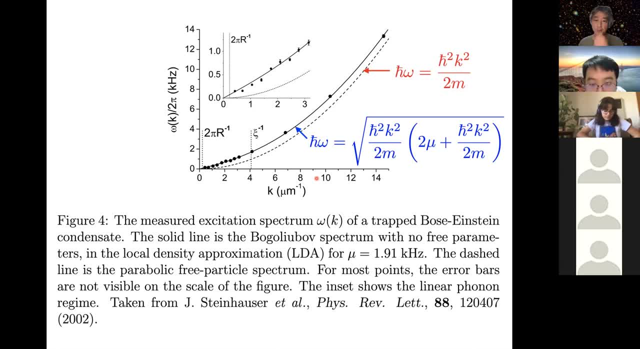 of the excitation you created, just by taking the energy and momentum difference between initial and final states of the photon. So energy and momentum conservation allows you to extract energy of the excitation created and momentum of the excitation you created, And then you just plot them on this k omega plane. 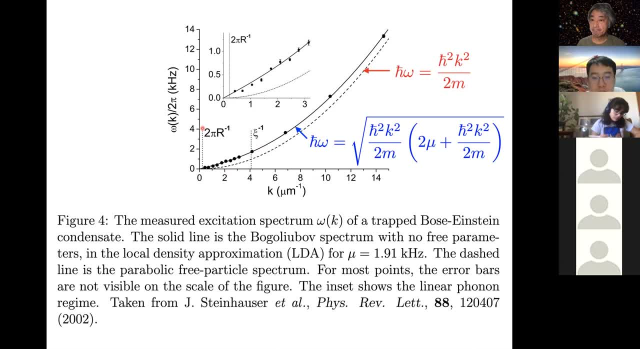 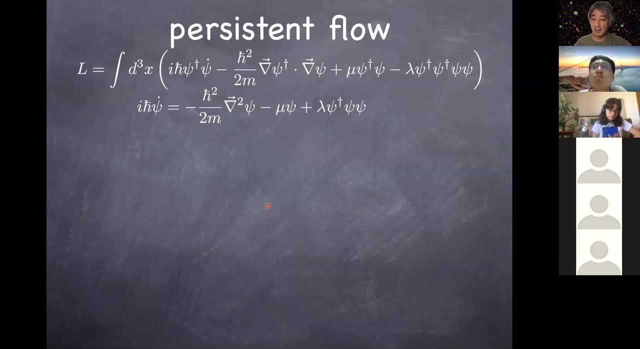 Any questions? OK, if there are none, let me just move on. Let's move ahead. And so that's one very, very important test of this field theory describing boson-Shinkansen condensate. Now I'd like to also talk about yet another exact solution. 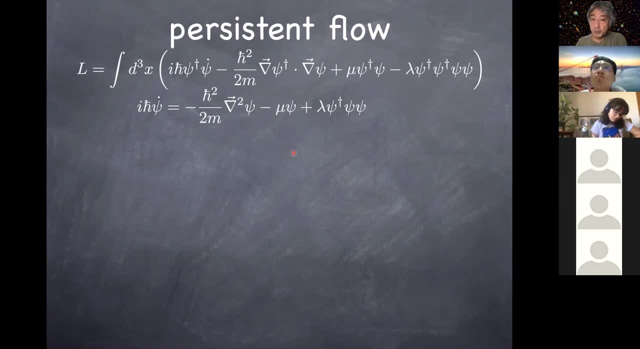 you can come up with to this Euler-Lagrange equation. Suppose you put a boson-Shinkansen condensate into or onto a circle. You can imagine that you create a tube like this and put it inside. So the whole point is that your condensate is now. 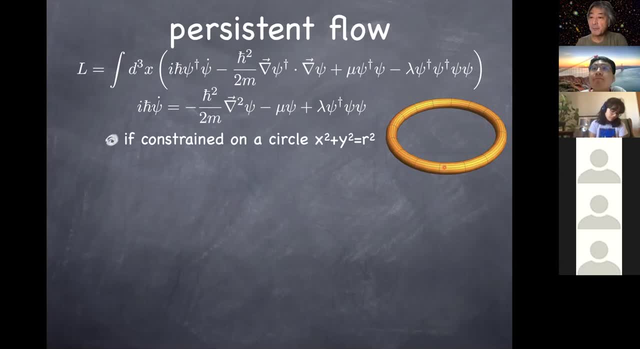 restricted on a circle with a finite radius And there's nothing inside. So condensate cannot be at the center, It has to be on this circle. So that's a situation we have in mind. Then obviously it's a lot easier. 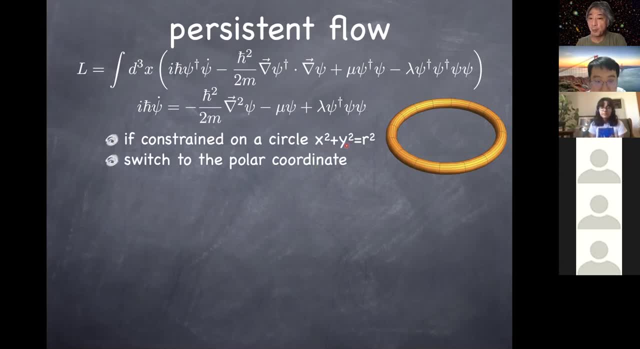 to deal with the polar coordinates r and theta instead of x. And why So? I rewrite this Euler-Lagrange equation using polar coordinates. So this derivative squared is now written by the second derivative with respect to r and second derivative with respect to theta. 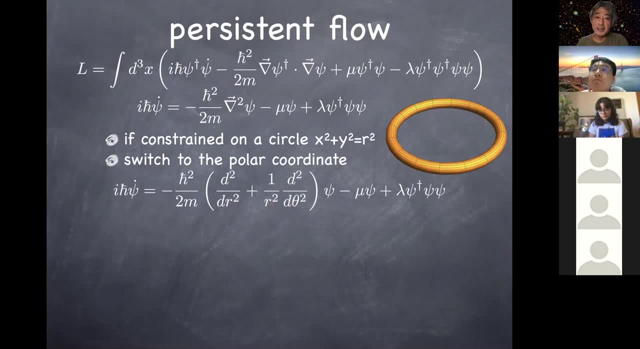 with one of r squared in front. So this is just rewriting the Cartesian derivatives in terms of the polar coordinates. So there's nothing complicated here. And we are now saying this: that Bosangian condensate is restricted on the circle with a finite radius r. 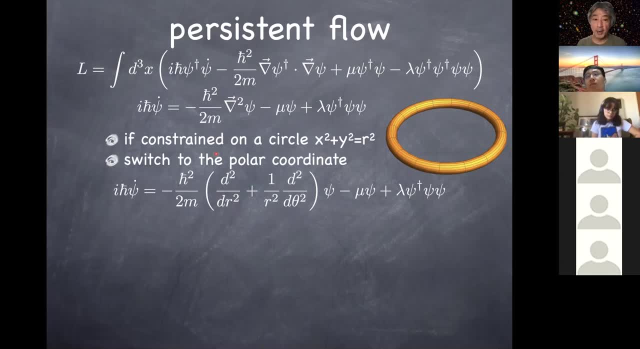 So they are not allowed to move in r direction. So I drop this r derivative right And in addition, this psi, which is now a function of r and theta r dependence, is now fixed, So there's nothing we should solve for this. 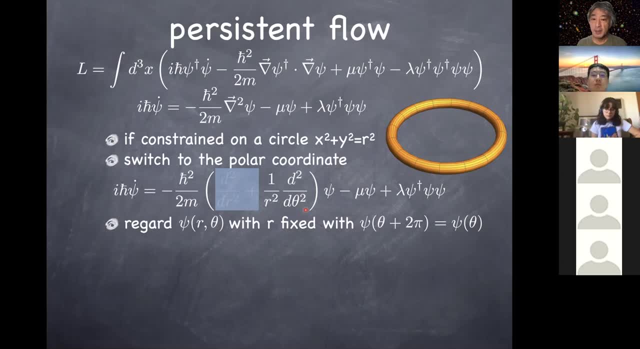 Theta dependence is what we need to solve for, Right, Yeah, But clearly in this theta direction, the polar angle. when the polar angle goes around the circle by 2 pi, then psi has to come back to where it was, Namely that psi should satisfy the periodic boundary condition. 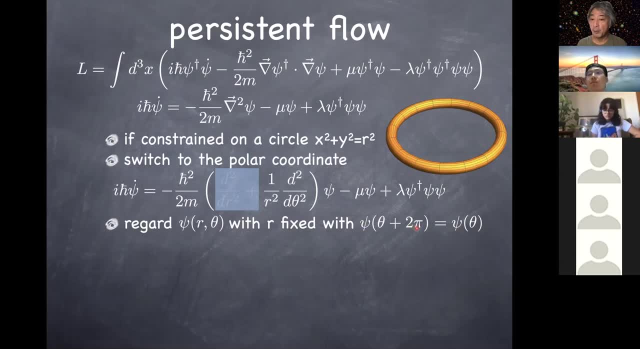 in a polar angle direction. So if you add 2 pi to the polar angle, then it should return to the same, the field psi. Once we know this, you can just go ahead and solve this equation, it turns out. So what we do is to take the modulus of psi. 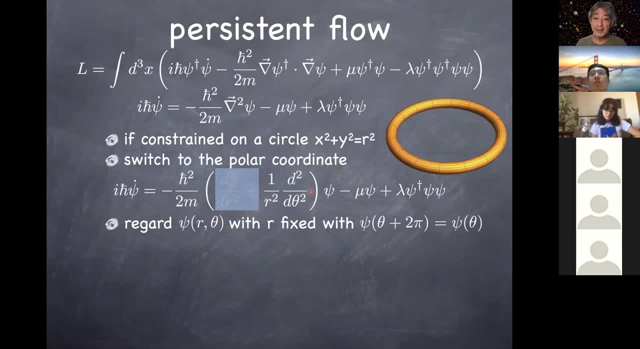 so that the last two terms cancel against each other, And then you make sure that theta dependence and time dependence of psi would balance this term against this term, And that's also easy to do. So this is a solution. It's a familiar factor right now, square root of mu over lambda. 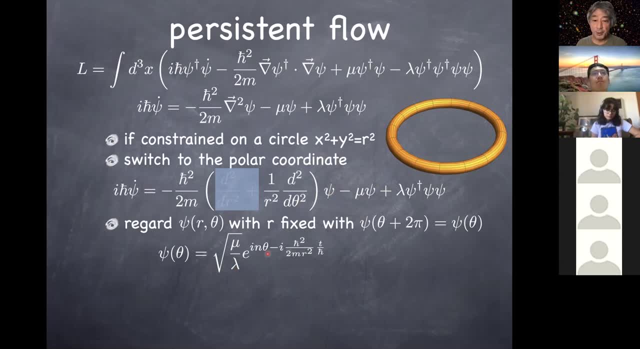 That corresponds to square root of lambda, The number density right, And then you have theta dependence, And because theta dependence has to be periodic, all it can be is e to the i n theta where n is an integer. So that's basically the full EMOs. 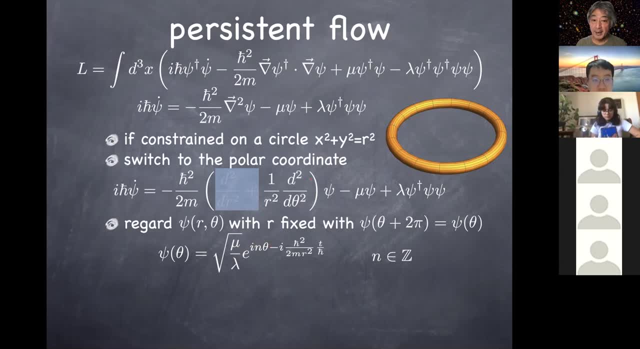 And once you know the theta dependence with this integer n, you know what you get from this And you're supposed to get the same thing from time derivative. So that fixes the time dependence to this value And I apologize, I forgot n squared in it. 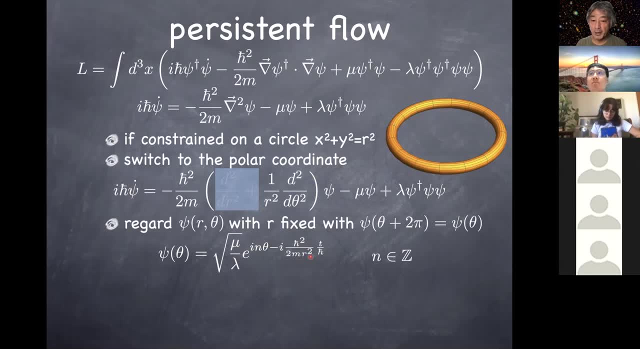 So h bar squared, n squared over 2mr squared is the coefficient of t over h in the exponent. So now you have an exact solution. An exact solution is now labeled by picking an integer. It can be positive or negative, just any integer. 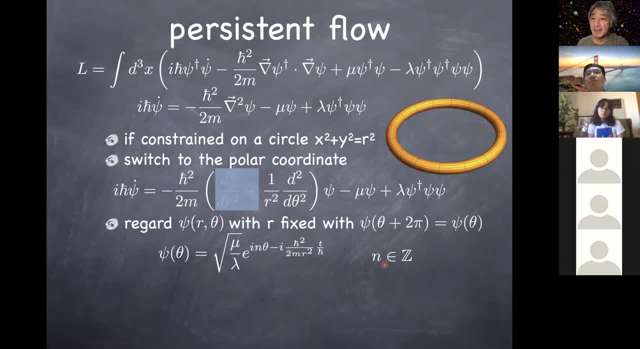 But it can't be a fractional number or a rational number. It can't be 3.14.. It can't be 2.5.. It has to be 1, 2, 3, minus 1, minus 2, minus 3.. 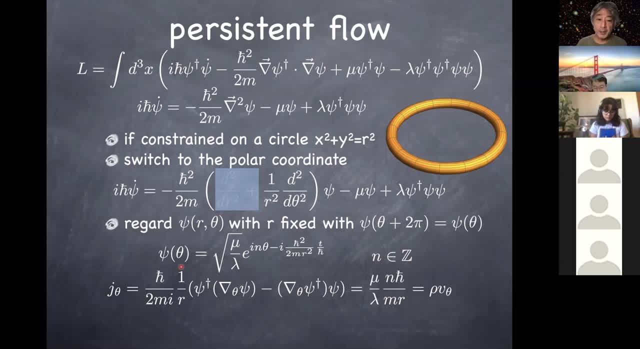 It has to be an integer And once you have psi you can compute the current, which is basically the same thing as saying: you use momentum, which is h bar derivative over 2m, but now written in terms of polar coordinates. So this theta derivative is 1 over r in front. 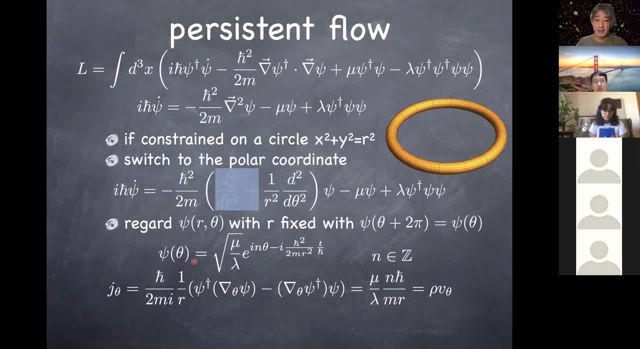 And you use this psi as a classical wave and compute the current of this classical wave by this expression, And that turns out to be very simple. And this mu over lambda again, is the number density, To avoid the clash of notation with n as an integer. 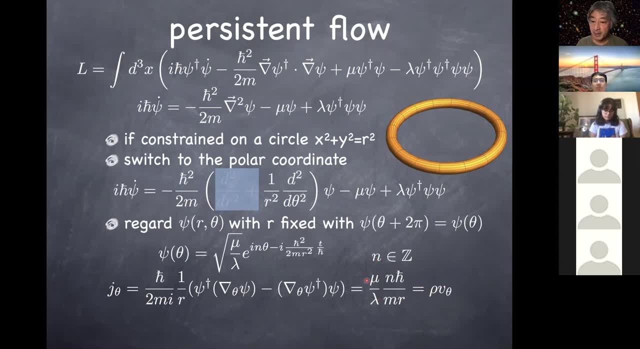 I used rho to represent the number density And the rest is the velocity. The current has to be the same as the number density times the velocity field. That's what we do in fluid mechanics. So now you can. You can compute the velocity which. 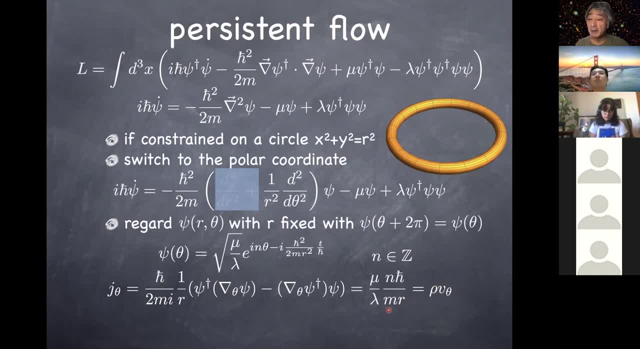 is given by 2 h bar over mr in theta direction And this allows you to compute a quantity called circulation in fluid mechanics This is the velocity. When velocity actually goes around this ring, then you just integrate this velocity around this entire ring. 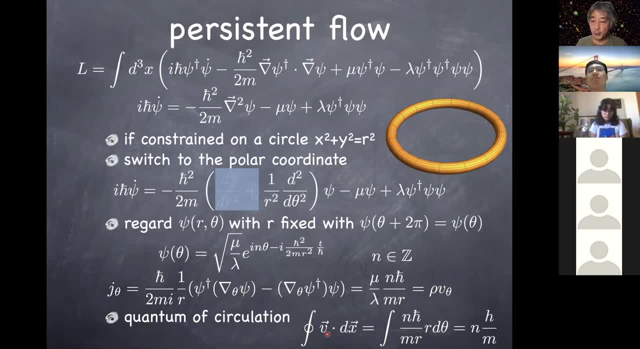 Then that's the definition of the circulation. So you just plug in this velocity, You plug in this velocity into this definition And dx is nothing but rd theta along this ring, r cancels And d theta gives you 2 pi, 2 pi times h. bar is h. 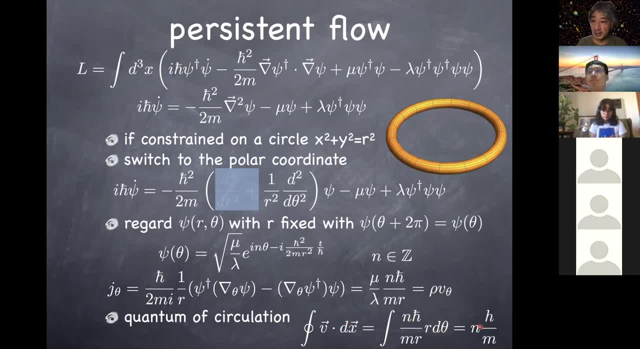 So what do you find in the end is this: circulation is quantized, So circulation basically measures how much flow is going on inside this ring, And But This flow is quantized in the unit of h over m, That's the quantum of circulation. 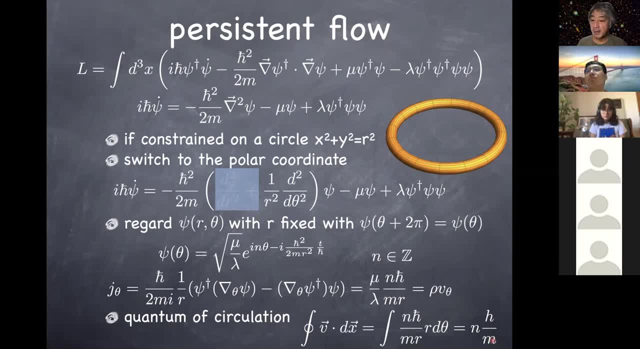 And the flow of the Bose-Einstein condenser inside the ring has to be integer multiple of this. Now we are seeing something really strange. We are dealing with classical field theory, But now you see quantization condition of the circulation of the fluid. 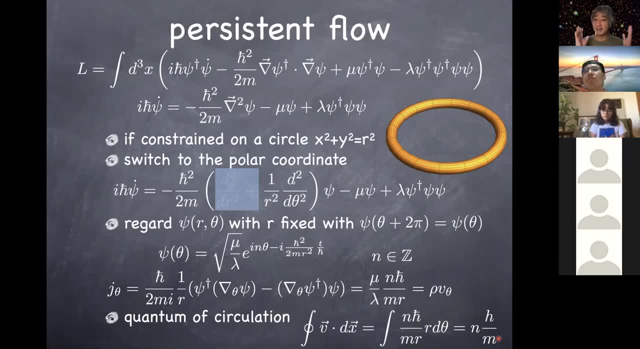 And of course In some sense this is nothing surprising, Even in classical field theory like electromagnetism. Once you put, for example, the electromagnetic field inside a cavity, you have boundary conditions, And then the frequency and wave vectors become quantized. 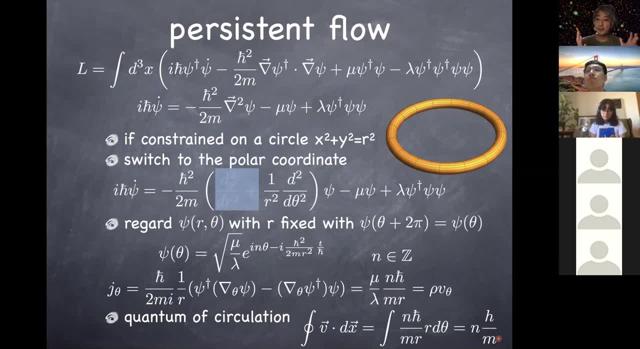 So in some sense this is the same phenomena In classical field theory. with given boundary conditions, you see only discrete modes present in the solutions of the system. So what we are doing here is the same thing, OK, But from the point of view of atoms this is a very surprising result. 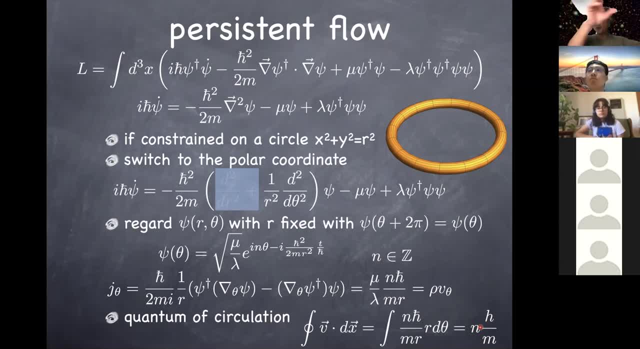 You have these thousands and millions of atoms flowing inside this tube, But the velocity this fluid can have comes with the integer multiple of certain quantum unit. That is more surprising. So from the point of view of classical field theory, getting this kind of quantization is not too surprising. 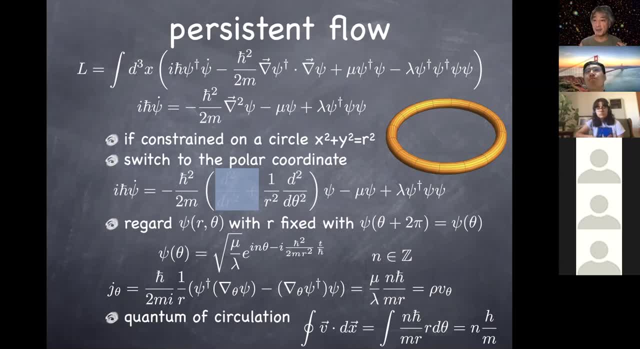 because they are basically resonant modes inside a cavity And stuff like this. But from the point of view of individual particles this is surprising because the particles are allowed to flow in a velocity only in some discrete units. Current inside this tube is quantized. 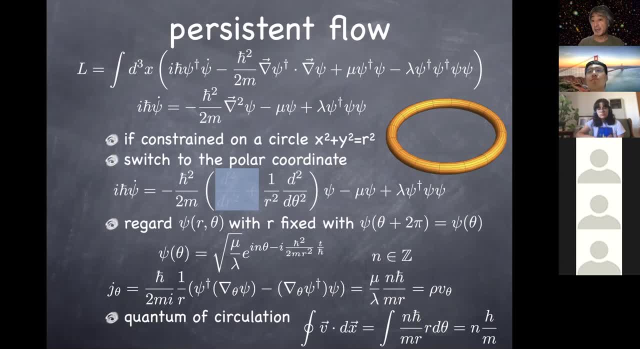 And that's a prediction we get from this classical field theory, But it's a very surprising result. If you go back and think of this as a system of macroscopic number of atoms, this is a very surprising result, But that's the prediction again. 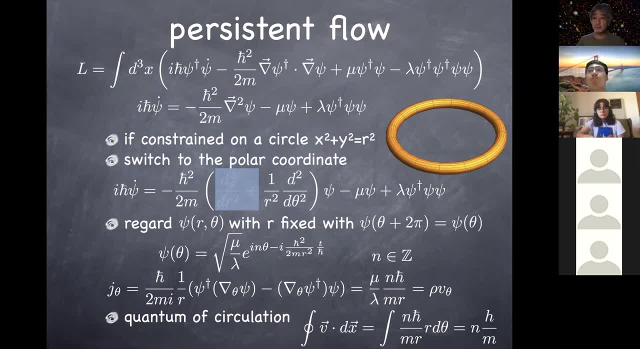 Any questions about this discussion here? I just had a question on where do you get the quantization of n in the solution of psi n? Yeah, This is just because of periodic boundary condition. Oh, OK, Yeah, If you go around the circle, then psi. 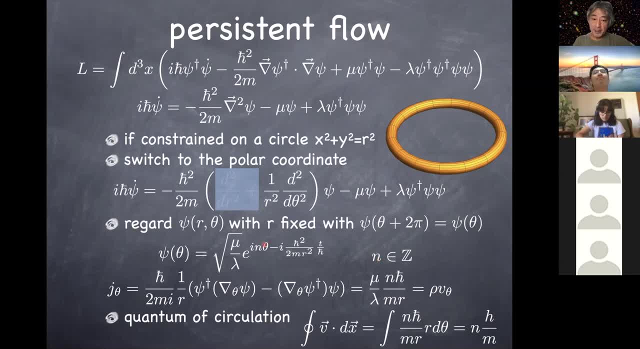 has to come back the way it started with, And that's why theta dependence always need to come with an integer, Yeah, Yeah, And that can't be 1 and 1 half or minus 2.4.. It has to be an integer. 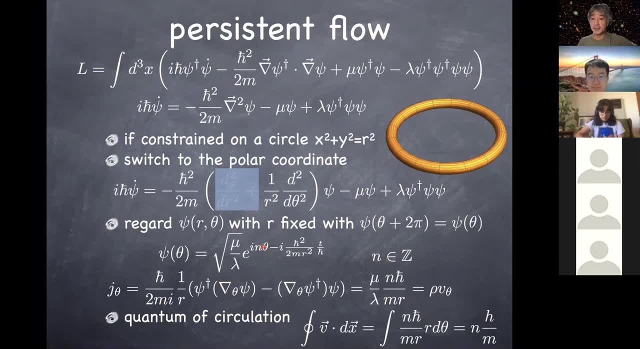 OK, OK, Makes sense. So that's the boundary condition in this system, using this analogy to the cavity electromagnetism. Any further questions? No, OK, So now the flow of this pulsation condensate inside this tube is quantized. 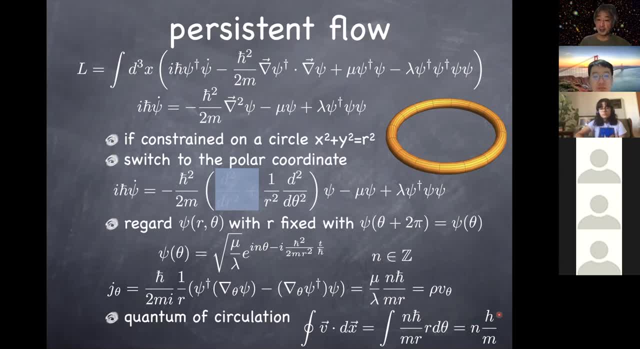 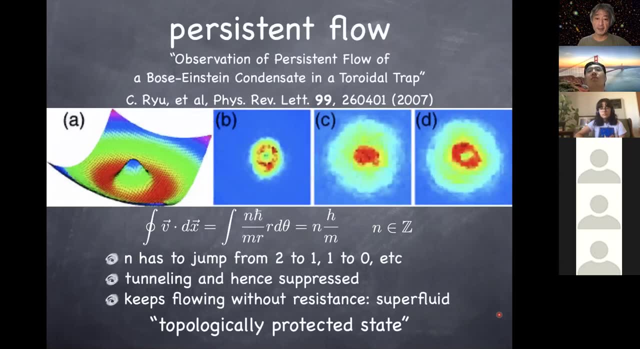 It's quantized in this unit of the circulation. Most surprising thing you can deduce from this is the following fact: There has to be a persistent flow, And what it means is that suppose you already have the flow, with this n being 2.. 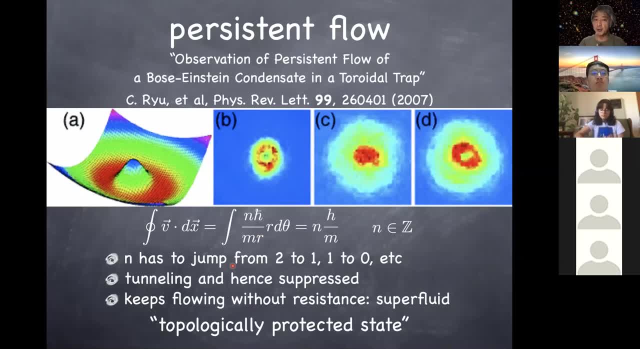 So you have twice the quantum circulation. So suppose you have a pulsation condensate of that sort, What do you do is to first produce a potential trap so that fluid can be around this center but not at the center, And this is the situation that would sort of realize the tube. 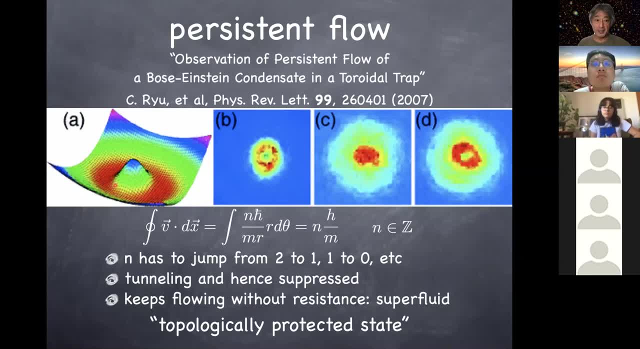 in an ideal setting. I talked about it on previous slide, But this is something you can do experimentally, So this is sort of the best you can come up with which corresponds to the tube on the previous slide, And you can indeed trap a pulsation condensate. 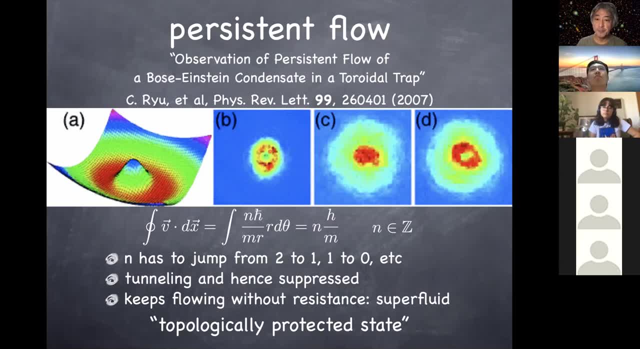 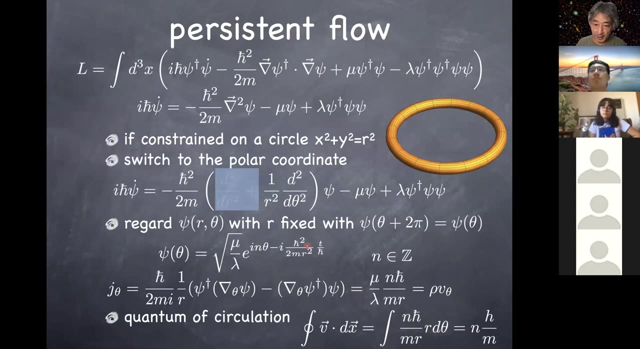 at the bottom of this potential. OK, So this is the tube. And suppose you created a pulsation condensate with n being 2. And n would correspond to the kinetic energy, which is n squared. So that's all I forgot to write here. 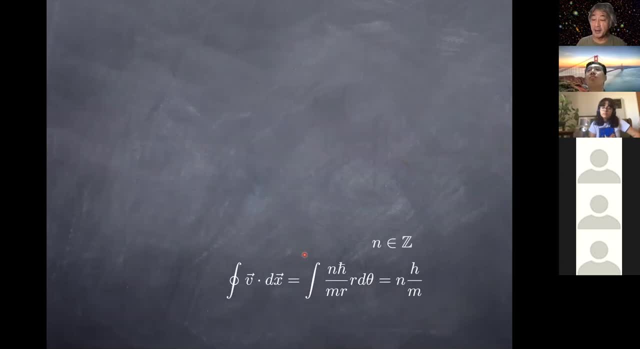 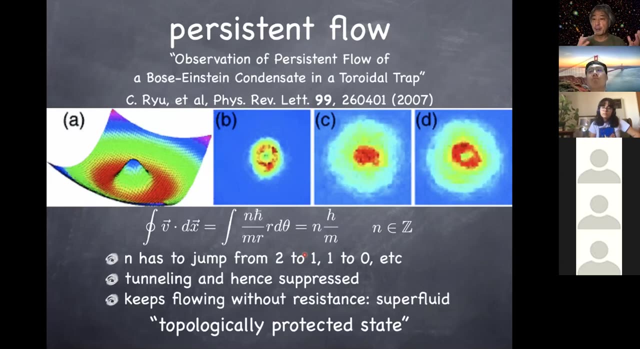 So n squared is the kinetic energy. So the larger the n is, you have higher energy. So you would think that if you start out with a pulsation condensate of n being 2, you will probably decay to n equal 1.. 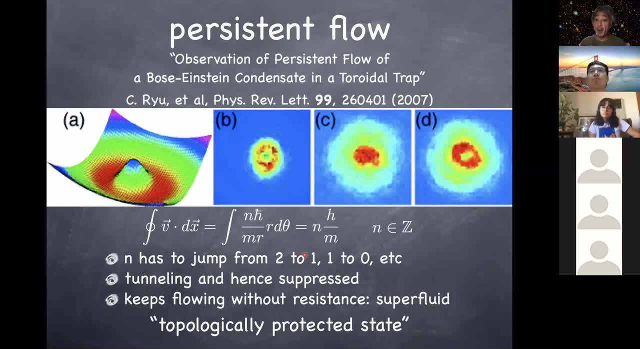 And indeed that can happen. But you can't go in between. n has to go from 2 to 1 without decreasing 2 to 1, but rather has to jump, because n has to be an integer. It can't be 1 and 1 half. 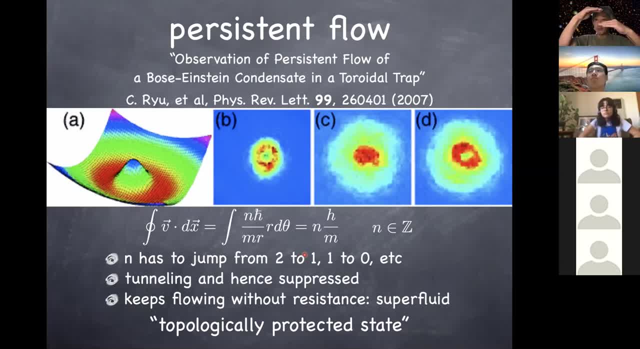 It can't be 1.97.. So you have to jump from 2 to 1, which basically corresponds to a tunneling process. So, just like you have a potential barrier between two states, you can't hop over classically because you don't have energy for it. 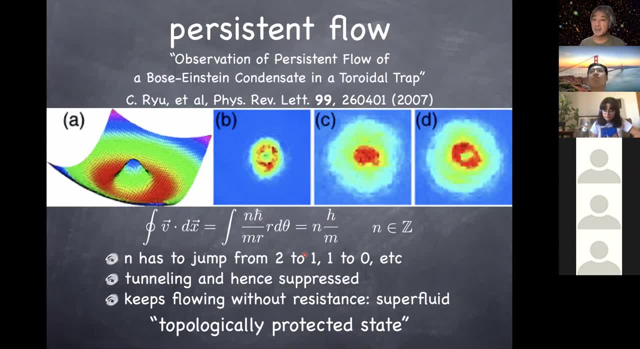 You have to tunnel through it, Then the tunneling process is exponentially suppressed in terms of its rate, And that's a WKB approximation you might have heard of in the quantum mechanics class. Actually, I don't know. Have you studied the WKB? 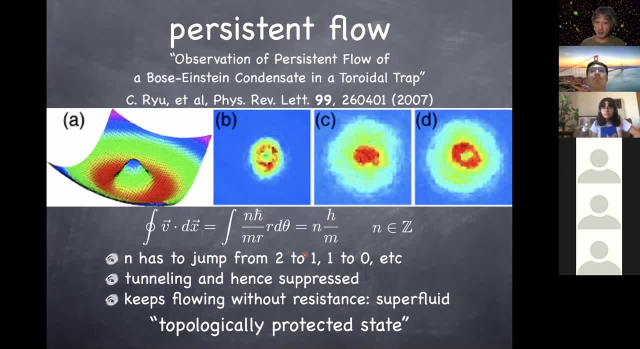 OK, good, good. So the tunneling process is always exponentially suppressed because of this. And exponential suppression, what exponent in this case is proportional to number of products you have in the system. So it's actually quite a bit suppressed, So it doesn't happen very quickly. 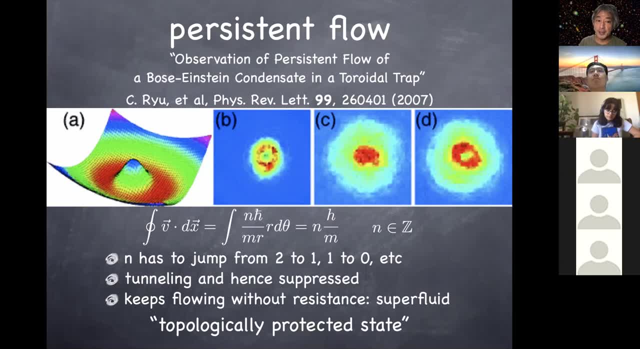 So once you actually trap the system along this bottom, this potential inner circle with n greater than 1, it will stay with that number for some long time. So sort of the idealization is what is called a persistent flow. Of course that's really idealization. 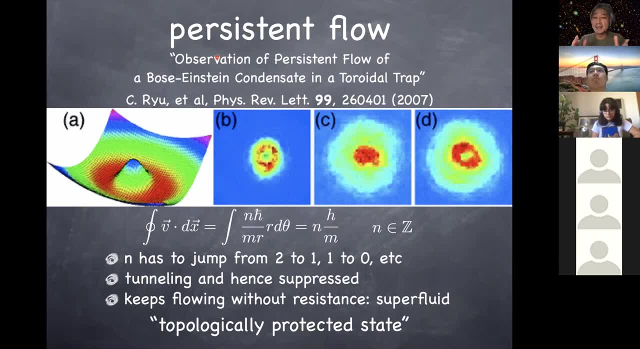 It doesn't last forever, But it can last at least for a long time, And this is an example of the phrase you might have heard of, especially in condensed matter physics, called topologically protected state. n is an integer, And this has to do with something called topological invariance. 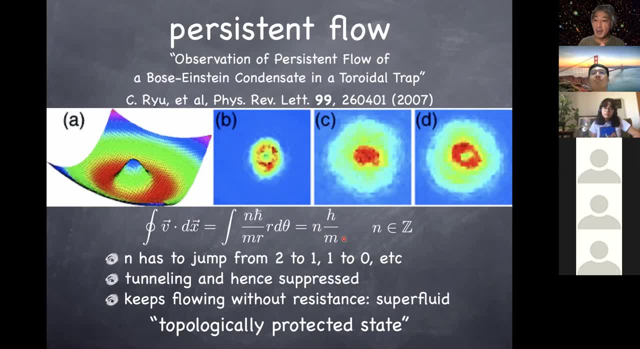 And so n being an integer doesn't allow you to go smoothly from 2 to 1, 1 to 0. You have to make a jump, And the jump is always exponentially suppressed. Therefore, this state is protected And it can survive for a long time. 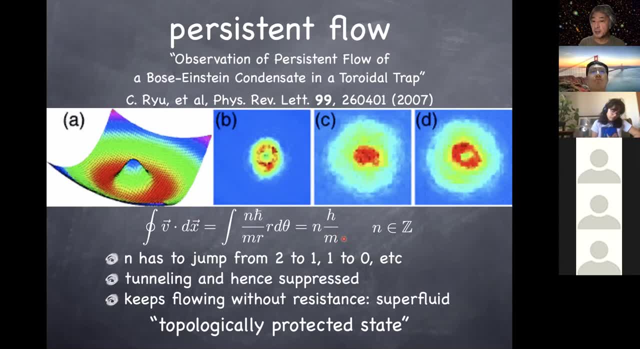 And that's the feature called topological protection. So this is one example of topologically protected state which you may hear about, especially in condensed matter physics. But same ideas also appear in particle physics, cosmology and so on and so forth. 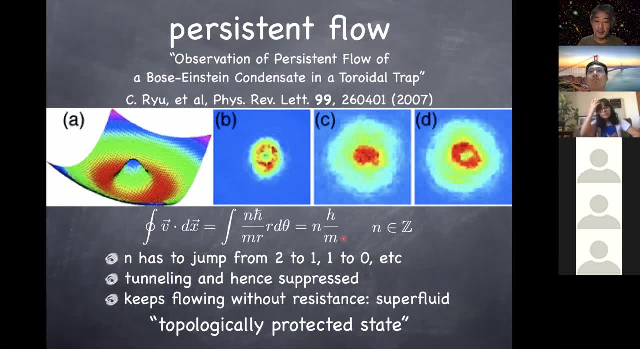 So this is the first example where you see this topological protection, And the second is the topological protection of quantum states. So let's look at how long they survive on the next slide And we can come back and talk about this conceptual idea after this. 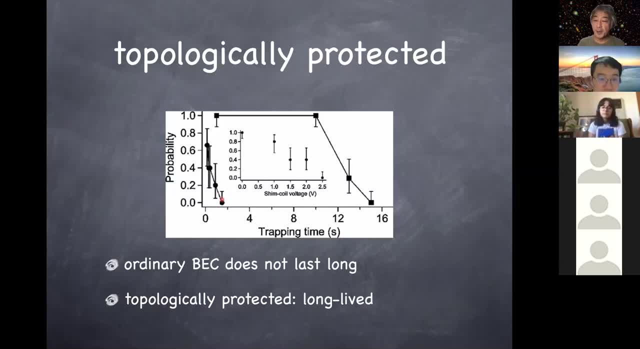 So this is the plot. So if you have a flow with n equals 0, that's the normal Bosangian condensate- you actually lose it fairly quickly, within a few seconds, And the reason being that inside this Bosangian condensate, 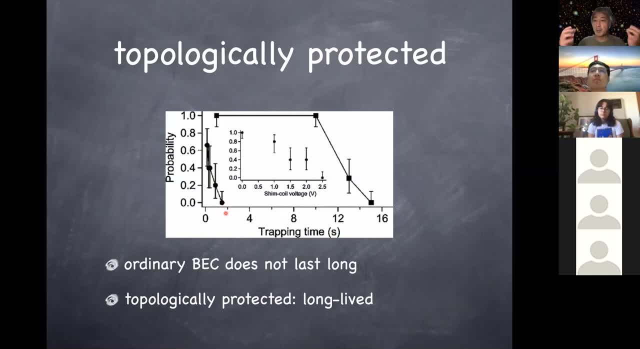 let's say you have two atoms scattering against each other. But you have, we have already taken care of you know, Lagrangian, this lambda psi, psi, psi, dagger, psi, dagger, psi, psi term is this two-body reaction between two atoms. 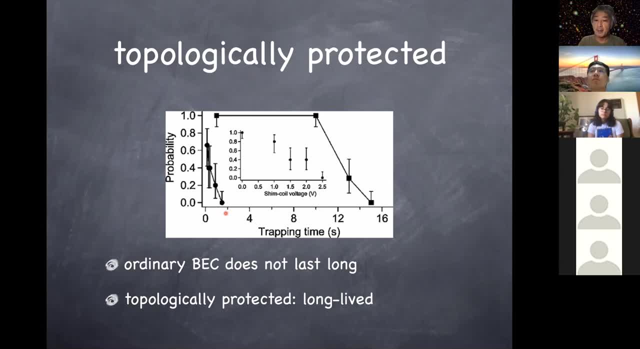 So we have taken care of that already. But very rarely maybe three atoms come together. When three atoms come together, two of them might decide to stick and form a molecule by releasing energy, by kicking out the third one. Then your gas of atoms start to look different. 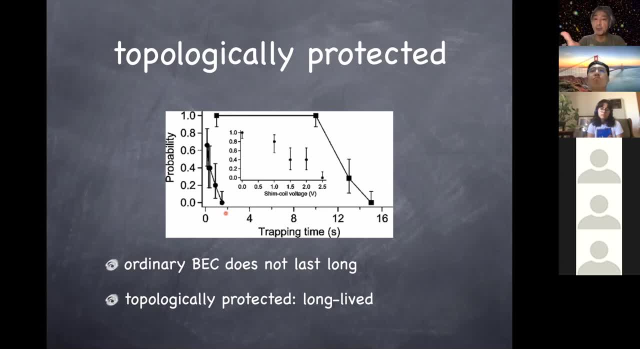 by forming these clusters of molecules in it, And that's how you actually lose the system. And that's why we have to make the gas very dilute, And that's why we require this incredible temperature to start with, So it would eventually, you know, disappear. 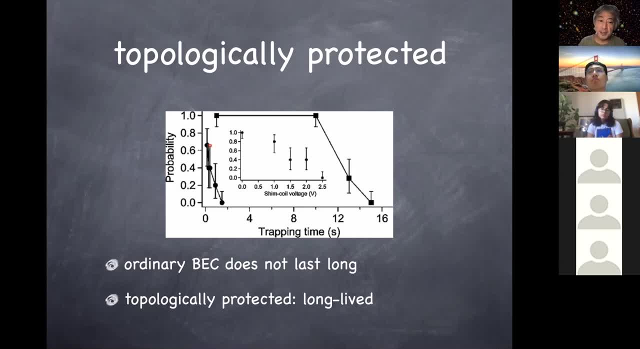 The Bosangian condensate don't live forever because of that. So ordinary BEC doesn't last very long, But if you have this BEC flowing at the bottom of this tube with a finite n, it stays that way much longer. 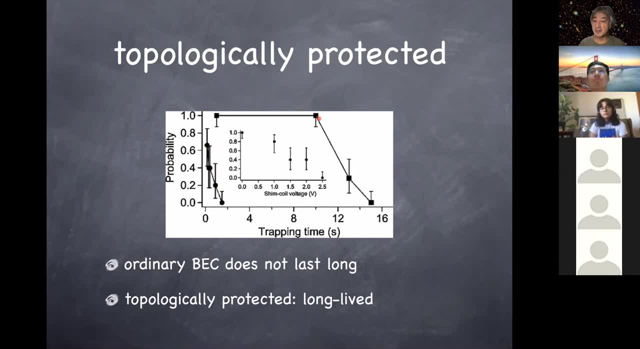 And that's an evidence of this topologically protected state. It's not persistent- That's an exaggeration, I have to say- But it's definitely long-lived compared to a typical Bosangian condensate by almost an order of magnitude. 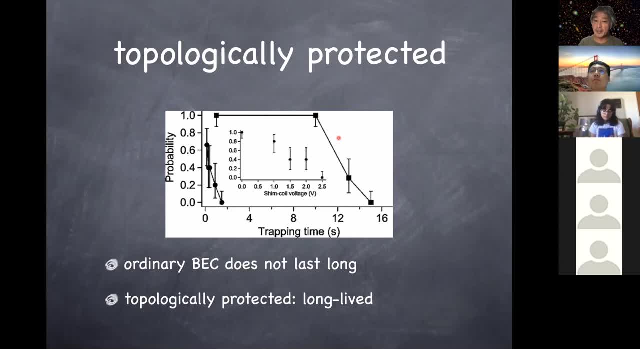 So the fact that this fluid of Bosangian condensate flowing inside this tube is characterized by integers- not real number, not fractional number, but integers- they come in discrete steps- provides a protection for this state to last long, compared to the state without the protection. 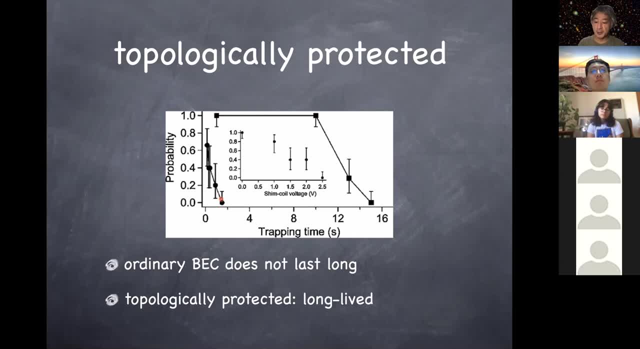 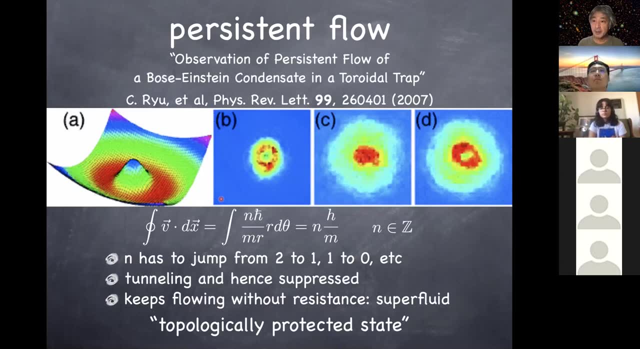 So that's an experimental evidence of this topological protection. Okay, so any questions about this concept over here, And you'll see more examples of this as we go on, So hopefully you get used to it at the end of the day, This is the first time you see this idea. 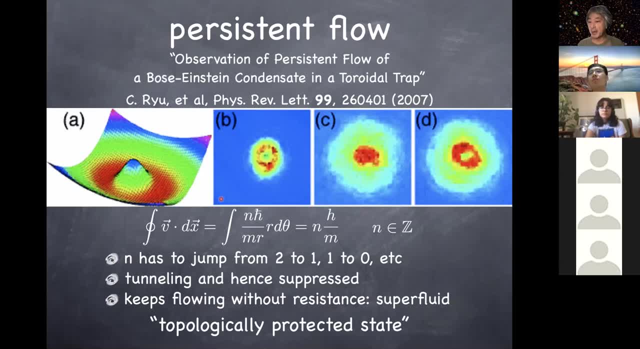 of topological protection. So I pose four questions: How exactly does the exponential suppression arise from this quantization? Yeah, so, because n cannot be between 1 and 2, it's basically the same thing as having a big potential that you can't be in between. 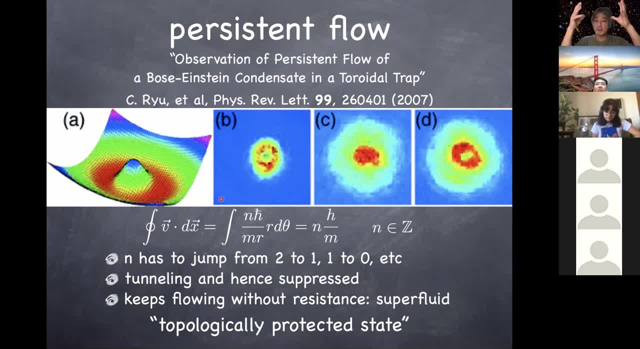 So that's an analogy which I can justify more clearly once I actually do this, A field theory calculation of it, And I don't do this in class, but it is something you can try. So even in field theory you can ask the question. 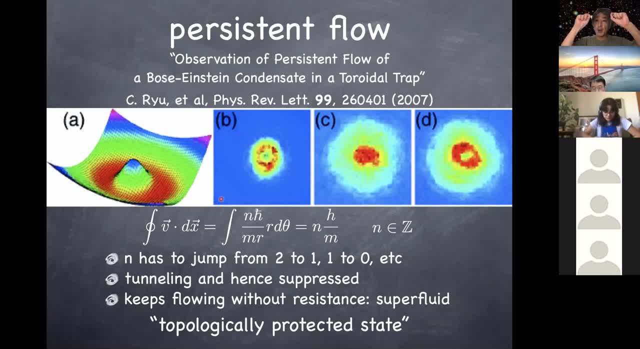 how you can tunnel from state 2 to state 1 through a potential barrier, And the tunneling process is something you can compute with WKB approximation And you have learned that WKB approximation gives you exponentially suppressed amplitude where exponent is given by x integral of p. 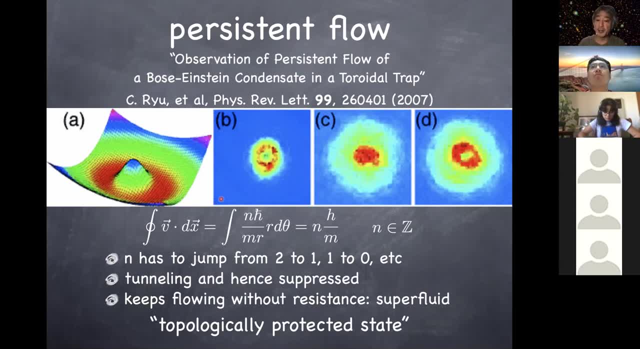 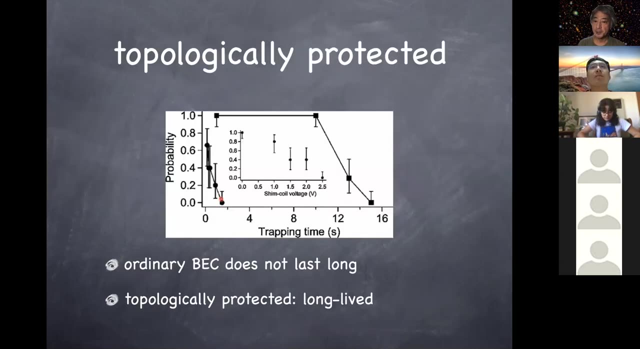 over h. So that's the exponential suppression. Okay, Makes sense, Right? Any further questions on this? Okay, Is this okay too? All right, So now you see, many, many predictions can be derived out of just simple classical Euler-Lagrange equation. 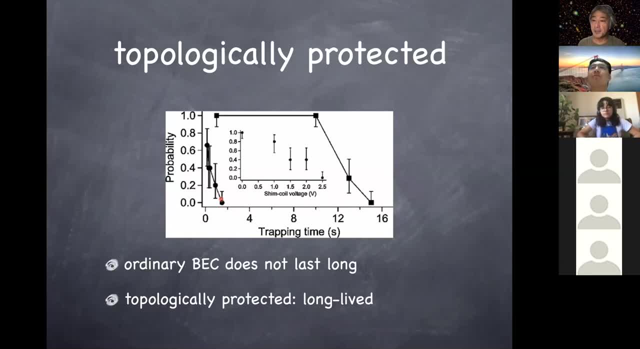 We have not touched any operators in all of these discussions, but we could work out the excitation spectrum in Bogorio, spectrum which really agrees with experimental data, extremely well. We could also derive this topological protection of a flow along the circle And we could actually verify. 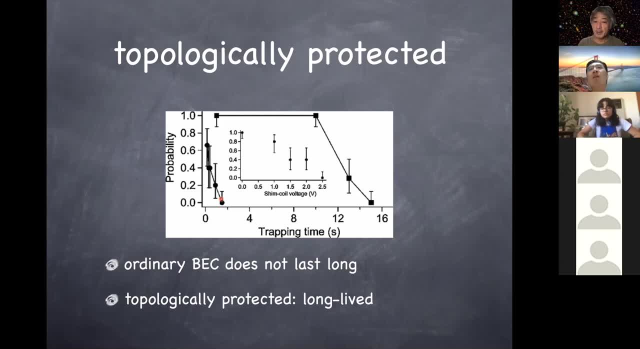 that experimentally as well. Now you can ask the following question: So you have now this potential where the Bose-Einstein constants are flowing at the bottom of this potential. Suppose you remove it, What happens to it? Clearly something is going around. 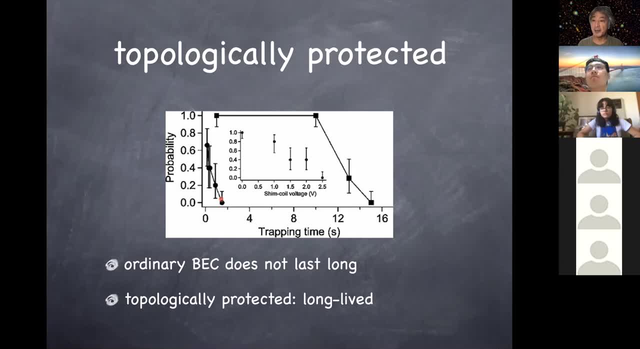 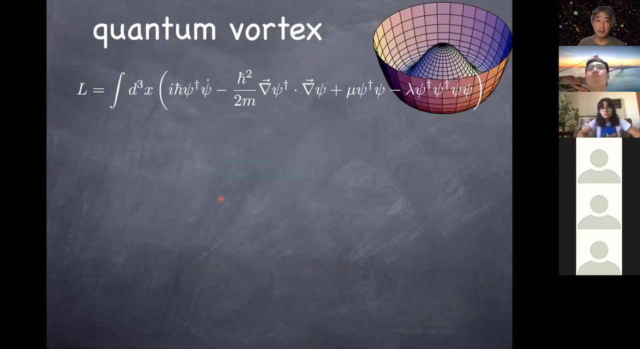 There is an angular momentum associated with this state And angular momentum is conserved. So you are supposed to get something non-trivial even after you remove the potential, And that is actually a vortex Of the fluid. So quantum vortex is actually a little bit complicated. 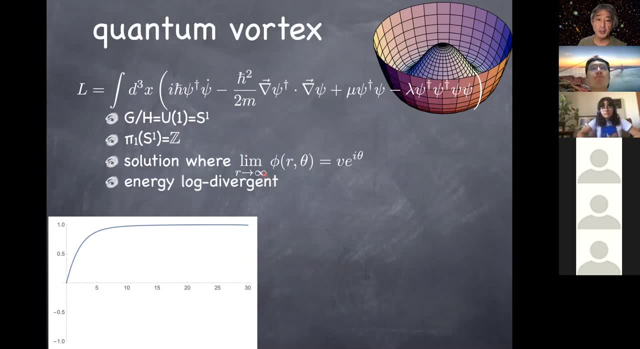 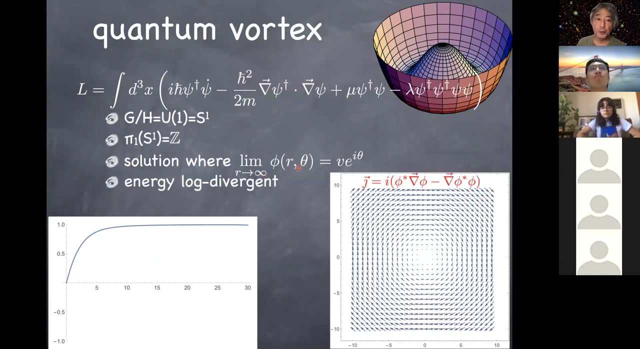 And you solve the Euler-Lagrange equation we have done before And you find a solution that looks like this: This phi. I'm sorry, I borrowed this slide from some other lectures so I haven't actually had to correct this. So this phi is meant to be the same thing as psi. 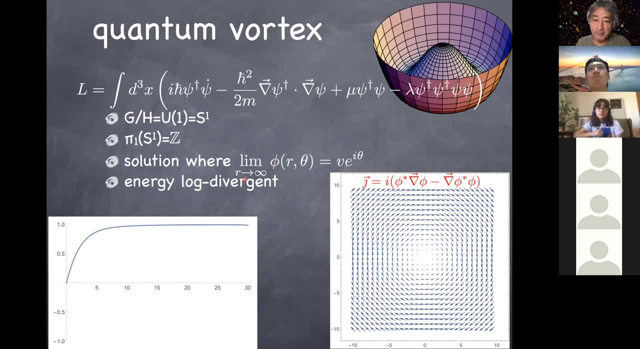 I apologize At the spatial infinity. it would approach the square root of mu over lambda. That's the ground state value of psi. But I can force this psi to have this phase factor we have seen on the previous slide. e to the i theta. 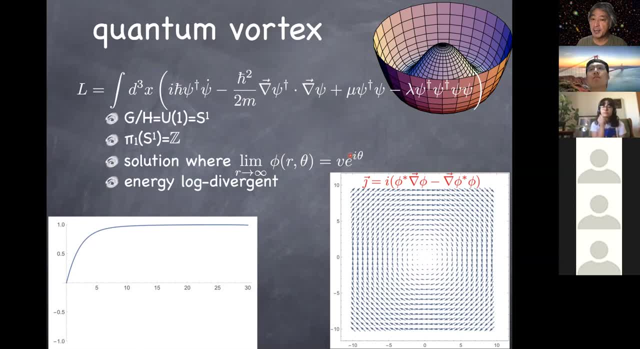 It can be e to the 2 i theta, 3 i theta minus i theta, but e to the i theta times integer. Here I'm looking at the simplest case, with the integer being 1.. And this v is the square root of mu over lambda. 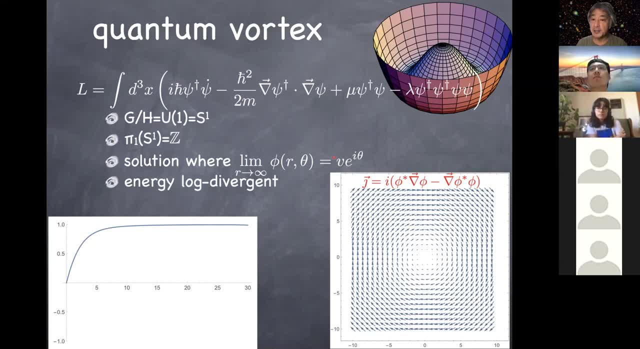 That's the asymptotic value, And so this is the situation you would see once you remove the potential out of that tube, right? So you have this e to the i theta behavior, But now that the potential is removed, this fluid can also be. 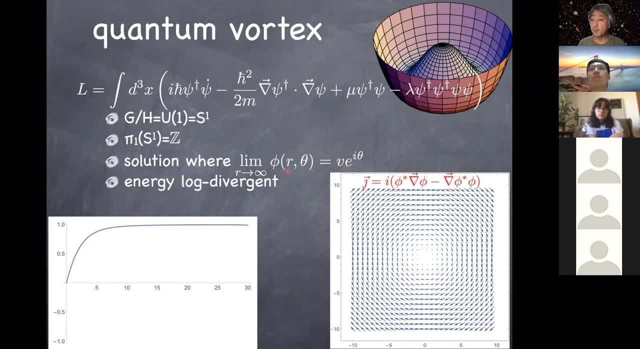 at the origin. But at the origin, in a polar coordinate, theta is ill-defined, So the only way you can make everything consistent is to force this psi to go to zero at the origin, so that you don't have this multivalued function. 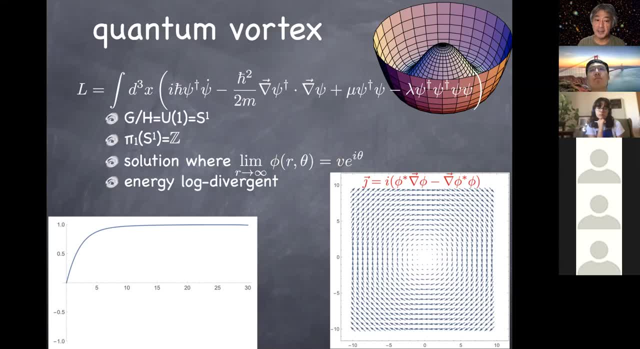 So it's still single-valued. So even though there's e to the i theta here, psi vanishes at the origin. Then you can interpolate between zero and the ground state value for the modulus of psi from the origin to infinity, which unfortunately you cannot do analytically. 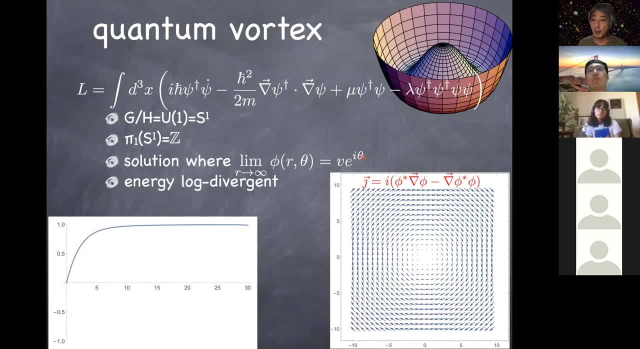 because of this nonlinear nature of the field equation. But you can do it numerically and that's what I have done with the Mathematica. So it's a smooth interpolation between zero and this ground state value. But the interesting thing is that, again because of this, 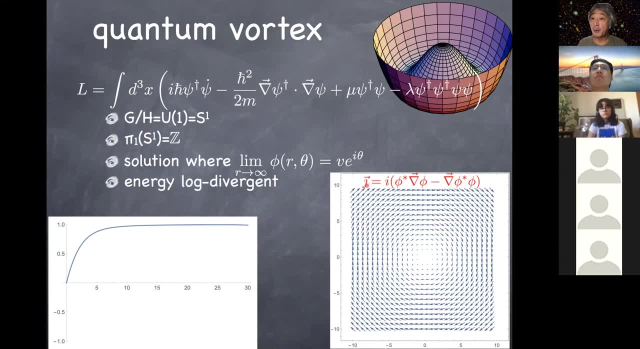 e to the i theta factor. when you compute the current, then it looks like this: It really does show that there's something going around, right, And that's the vortex. So you have a boson-strand condensate. and if you actually produce a boson-strand condensate, 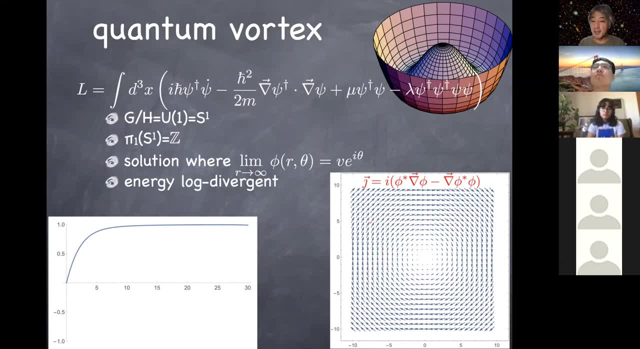 and you can rotate the system. then it starts to flow like this, But remember the circulation around the origin is still the same: quantum n times h over m. That hasn't changed. So you can create a situation of a condensate. 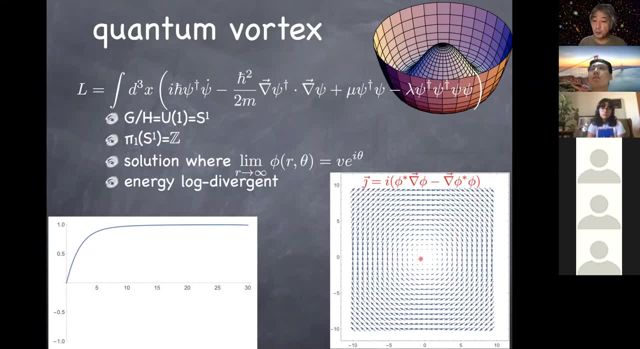 with an oval rotation which requires the condensate to vanish at the origin, And that's the vortex solution. Again, I can show the solution analytically, but I can show the solution numerically. And this is indeed the velocity field looks like. 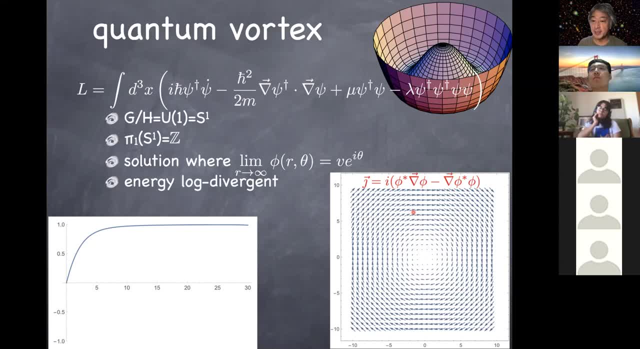 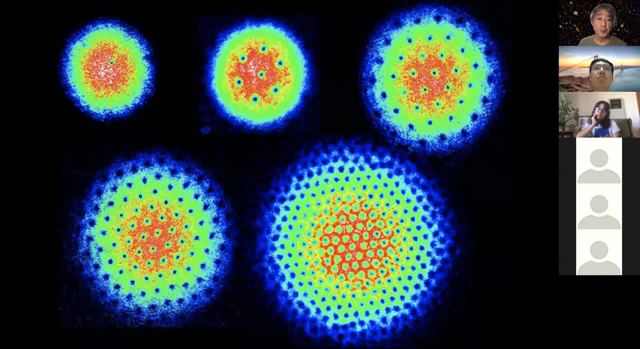 And the question is: can you really see this in an experiment? And the answer, of course, is yes. This is a boson-strand condensate with one vortex in it. This is a boson-strand condensate with. 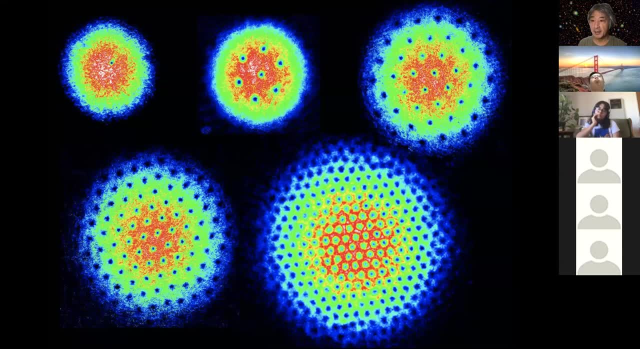 1,, 2,, 3,, 4,, 5,, 6, 7 vortices in it. It turns out that vortices would repel each other. They don't want to be as far away from each other. 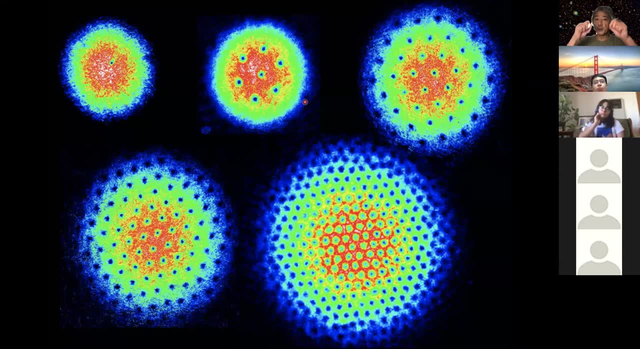 And when you have this plane, where you have things that repel each other to keep the maximum distance from each other, the best arrangement would be a triangular lattice. So you end up having this triangular lattice of vortices with higher and higher angular momenta of the boson-strand condensate. 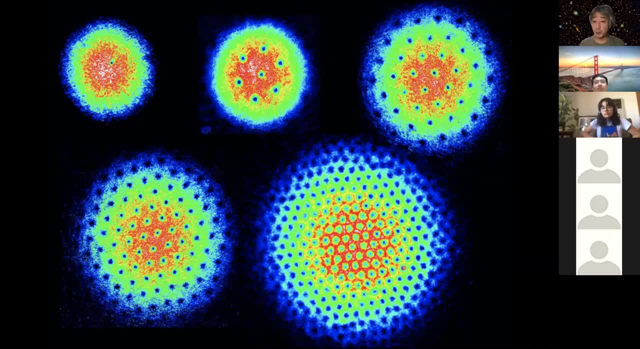 And that's something you can create experimentally and observe like this. And you see these blue dots, because this is where the condensate vanishes. Number density goes to zero at the center of these vortices, So it's sort of like a hurricane. 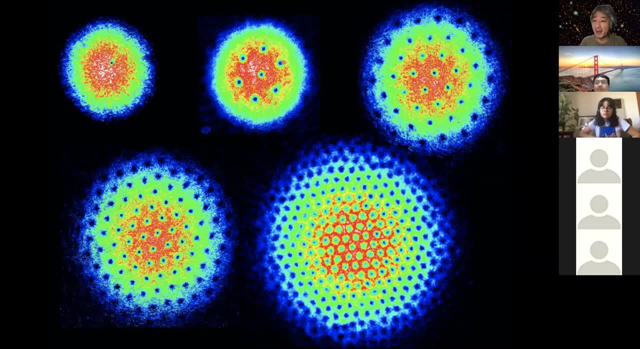 and these blue dots are the eyes of the hurricane, So everything goes around it. The center is a special place. So in the case of boson-strand condensate, centers of the hurricane are special places where the size of the condensate vanishes. 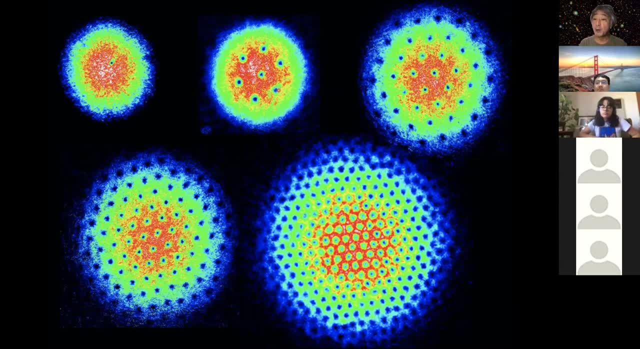 Number density goes to zero, so that the theta doesn't cause any ill-defined feature of this field: psi. So this is the way. just the classical solution to Euler-Lagrange equation led to so many different predictions by now. Vogelio spectrum quantized circulation. 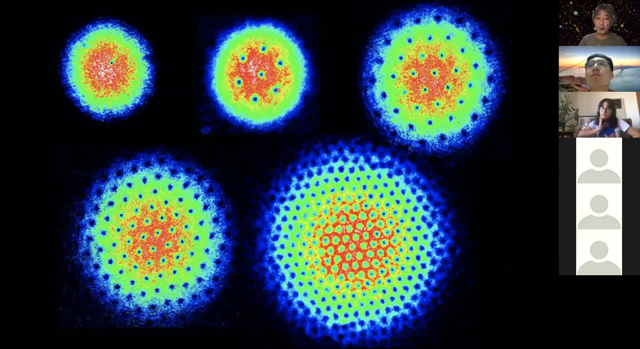 in the donut-shaped ring, and also rotating boson-strand condensate that leads to the triangular lattice of vortices, And all of these things follow from the single classical Euler-Lagrange equation. So this is a set of demonstrations. 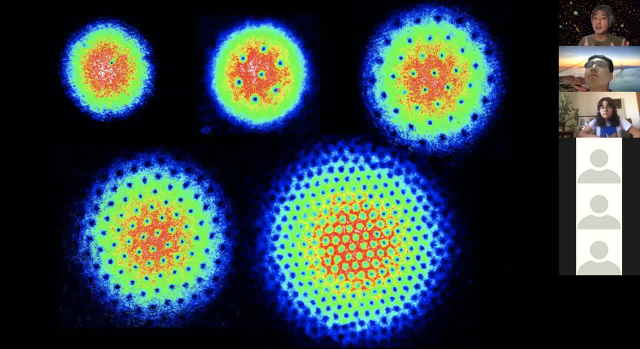 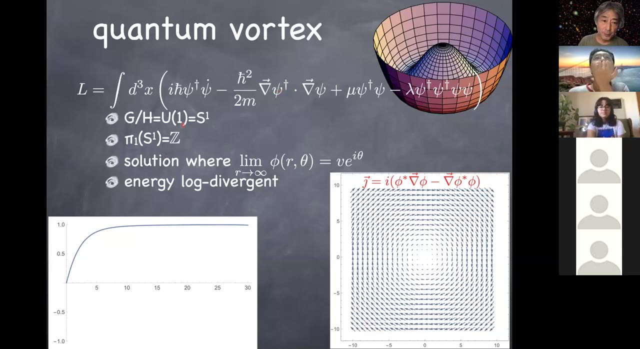 where classical wave is the right description for the boson-strand condensate. Okay, let me stop here and pose for any questions. These are beautiful pictures, but I think this is better to look at And just in case you're also wondering, 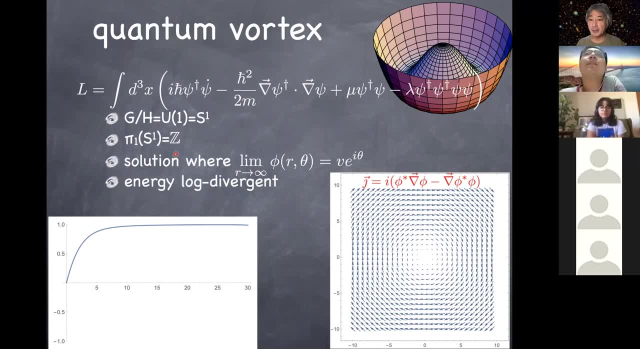 what the heck is this symbol over here? this is the way you actually analyze what is called algebraic topology. So these things are topologically protected. Again, there's some language to understand the topology of these things, which is primed by the integer. 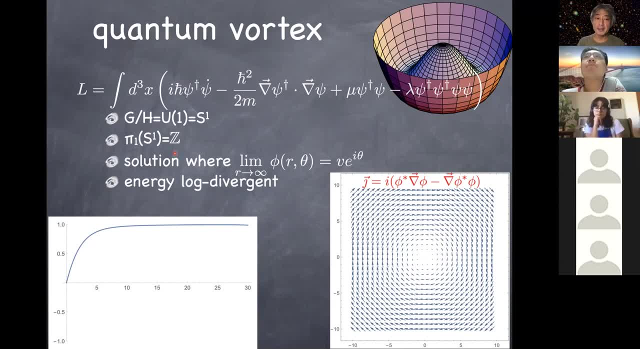 And it turns out that this is described by the same kind of topology when you take a rubber band and put that on the bottleneck, And rubber band corresponds to the infinity of space And the bottleneck corresponds to the phase of this field. So if you take the rubber band, 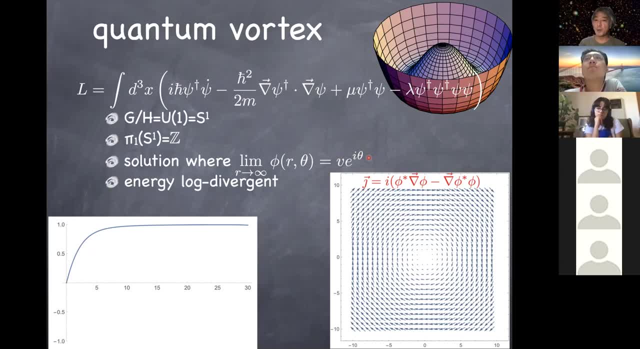 and put that n times over the bottleneck. that is what corresponds to e, to the n i theta, because spatial infinity would wrap around the phase of this field psi n times. And this is what mathematicians study as a map from one-dimensional circle to another one-dimensional circle. 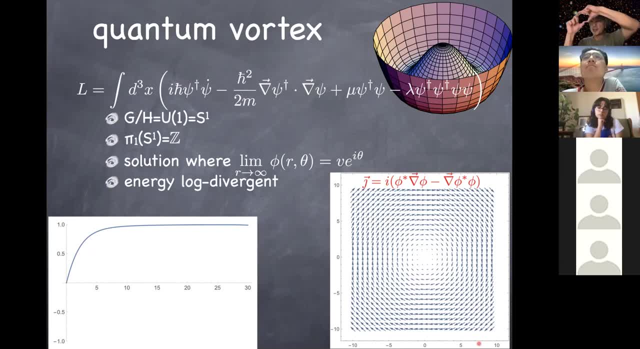 The first one-dimensional circle is spatial infinity. Another one-dimensional circle is the phase of this field, And writing the field as a function of spatial coordinate is nothing but a mapping from spatial infinity to the phase of this field, And hence it's the same problem. 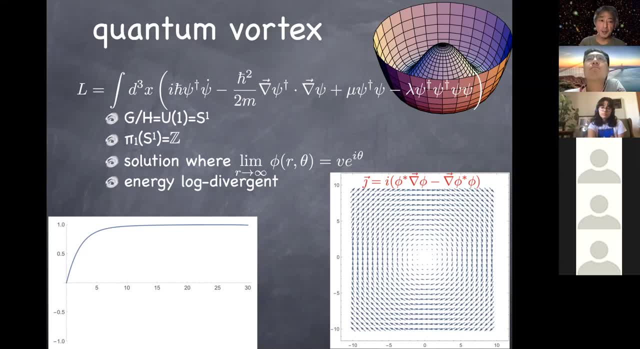 as the rubber band wrapping around the bottleneck, And that is what mathematicians say by writing down. this funny symbol is meant to be how many times you wrap around this rubber band on the bottleneck or phase of this field, And that is parameterized by the integer. 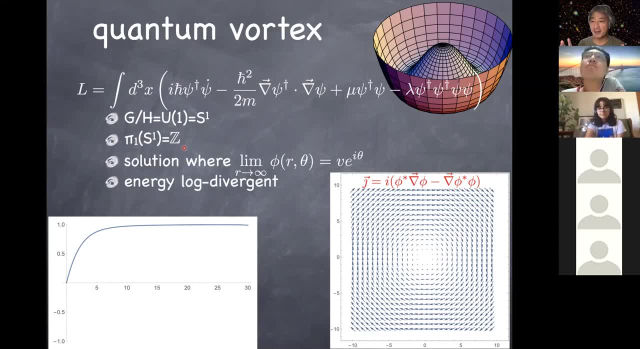 It's such a trivial statement, but this is the mathematical equations they use to represent that fact. So if you don't care about this algebraic topology, don't worry about it. We are not relying on this. We can still rely on this intuition. 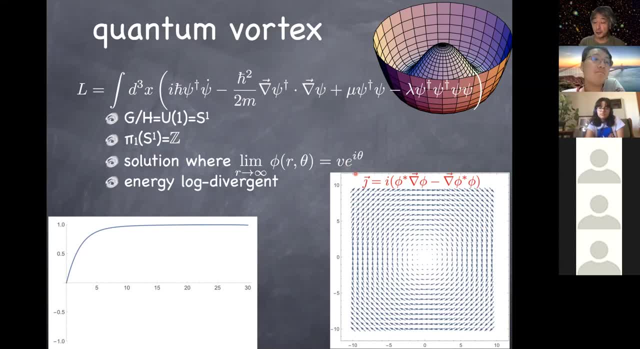 to wrap around the phase of this field: integer times. And it has to be integer because you have to come back to the same psi at the end of the day. So theta going to 2 pi gives you periodic boundary condition, And this is just a fancy way. 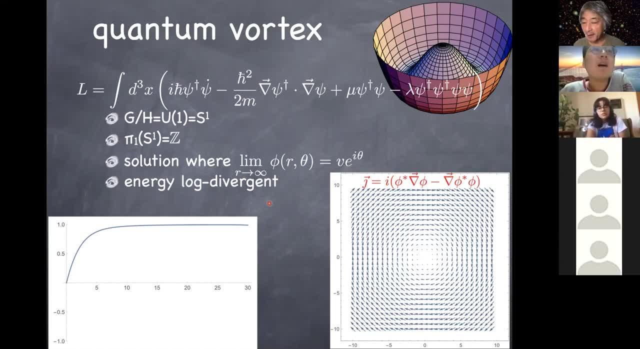 of expressing that. So any questions about this vortex solution? Anna wants to speak. Yeah, We've created the previous topologically protected state And then we remove the kind of toroidal potential that we've created. That's definitely one way to do it. 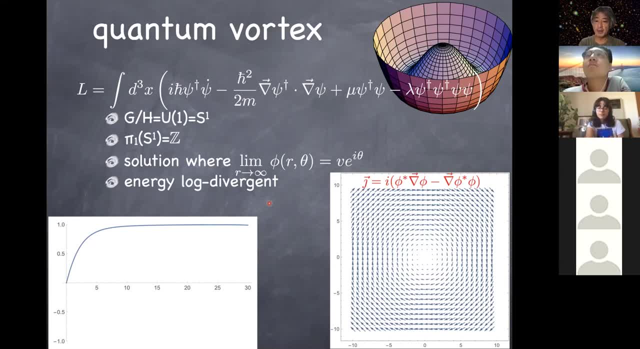 It turns out that you can also do a similar thing with an actual bucket. And so far we talked about the gas of cold atoms, But it turns out that low temperature liquid helium-4 can also exhibit the same behavior. It turns out that that is a superfluid. 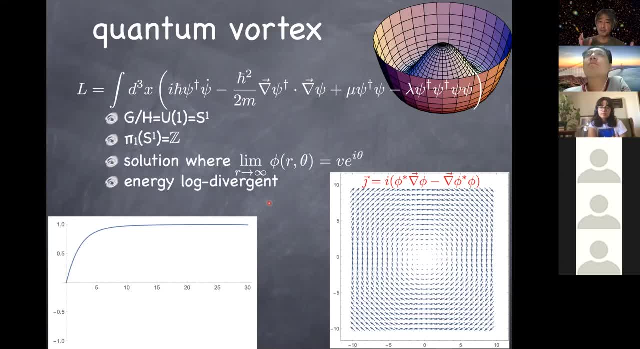 You might have done an experiment in a lab with a superfluid, I don't know. So the superfluid of liquid helium-4 can be described by the same machinery it turns out. So in that case you have a bucket and you fill it with liquid helium. 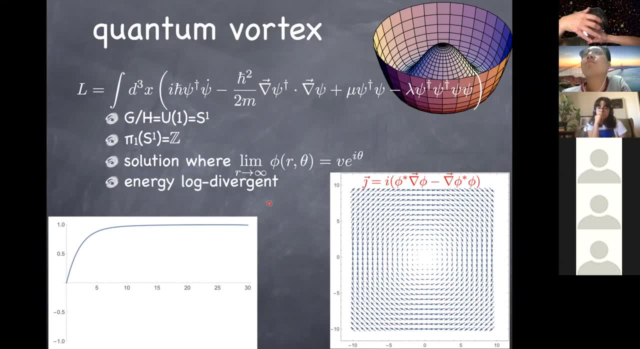 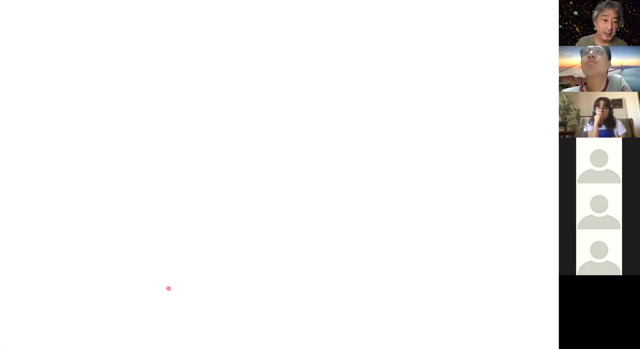 You cool it below the critical temperature of the limit and it becomes a superfluid, And that would lead to the vortices as well. And I don't think I have time to finish the discussion today, so let me just flash a picture of it. 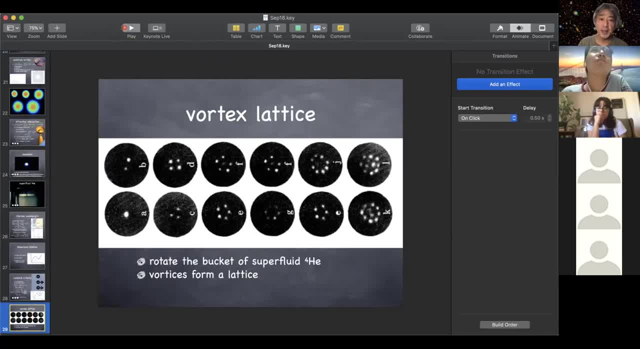 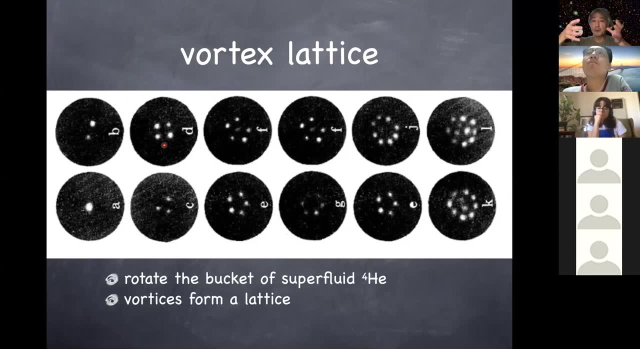 and then discuss it actually on next week. So this is the lattice of vortices of liquid helium and you literally rotate the bucket and depending on how much you rotate the bucket, you start to produce one vortex, two vortices, three vortices. 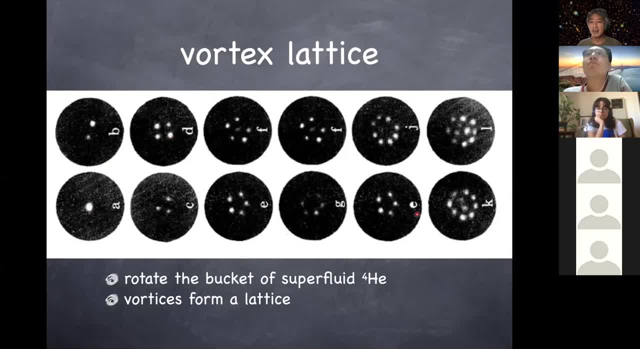 four vortices, so on and so forth, And they all line up neatly in triangular lattice. So that's another way of producing this lattice of vortices. Okay, so let me stop here and I can pose four more questions And the 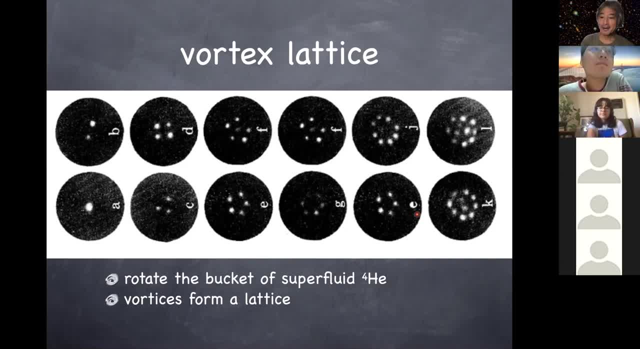 lecture is over Questions. May I ask another question? Go ahead. So the take-home message should be like: the vertices carry angular momentum, or if the BEC has angular momentum, it should have vortices, right? So the whole argument doesn't care. 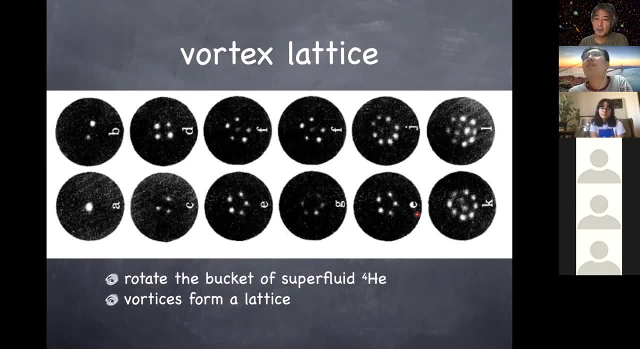 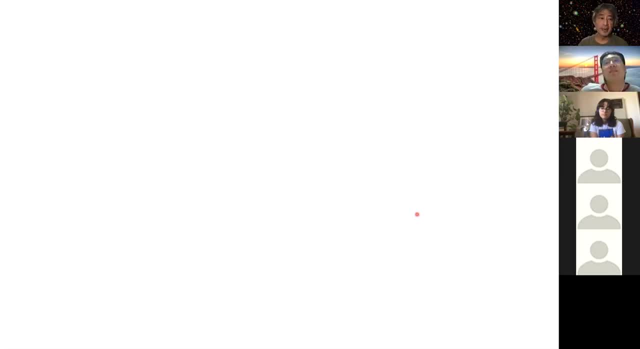 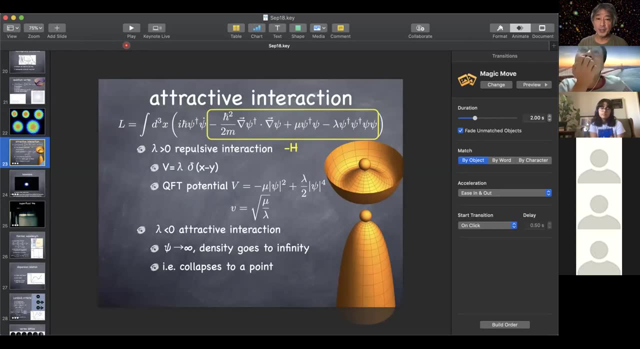 about lambda equals zero or not, like the hook you give. Yeah, that's an excellent question. So there's something special about lambda being the repulsive interaction and I meant to talk about this but I didn't get to it. So you can ask the question. 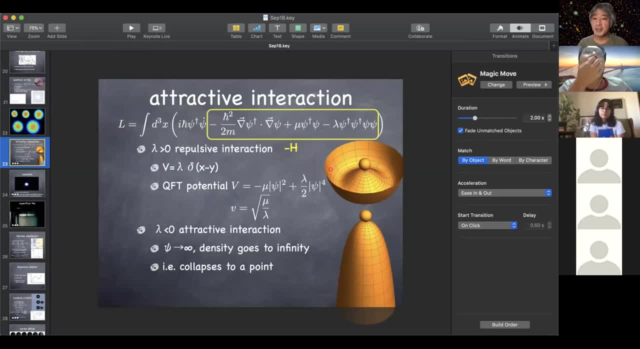 what if you change lambda? And once you actually change the lambda from positive to zero and negative, this potential I talked about this is the potential of the field, or Hamiltonian as a function of psi, with this shape to that shape, Then you can immediately see. 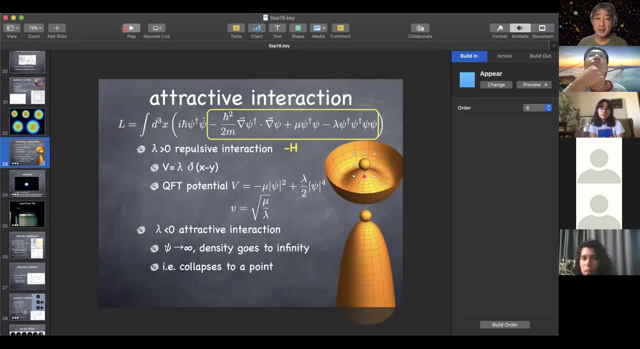 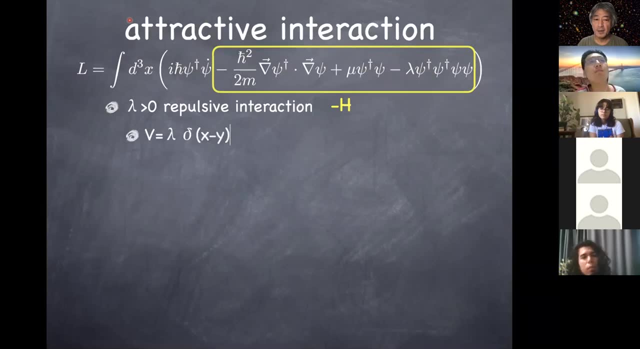 this would lead to a stable minimum. Sorry, And I'm going to actually talk about this again next week because we didn't get to it, But just for those of you who are still hanging out here, So this would drop to the stable minimum. 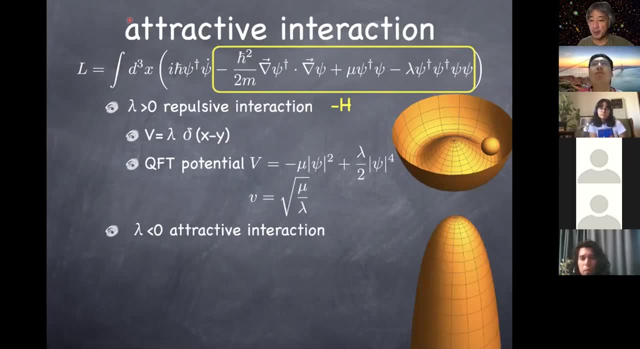 That's this one. But when lambda is negative, when you have the attractive interaction among the atoms, certainly this starts to drop indefinitely on this potential. So the field psi would eventually go to infinity, which means that density goes to infinity. In other words, 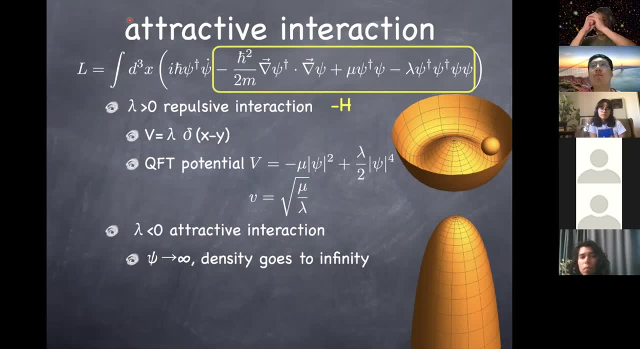 the Bose-Einstein condensate would collapse to a point where the density becomes infinite. So it's an implosion of Bose-Einstein condensate And you can do this experimentally, it turns out. So in some atomic systems you can change the repulsive. 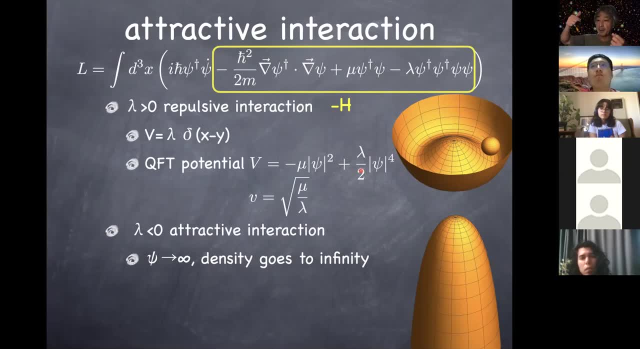 interaction to attractive interaction by dialing the magnetic field acting on the atoms. So you go from repulsive interaction to an attractive interaction by turning a dial on the apparatus And then, indeed, the system implodes. It collapses to a point And after it implodes. 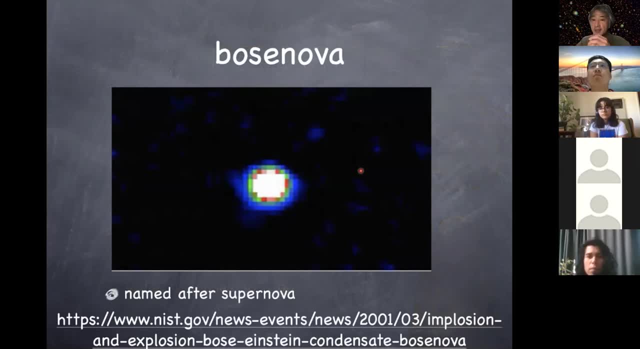 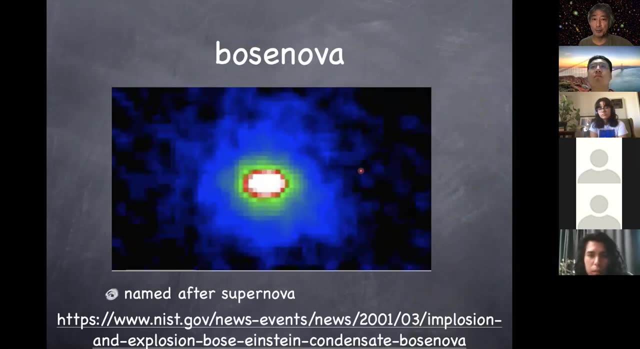 then there's a bounce, That whole thing starts to explode. And that's this movie, And it's called Bose Nova, And that's a joke, You might know, of a supernova. That's an explosion of a star that led to the discovery of dark energy. 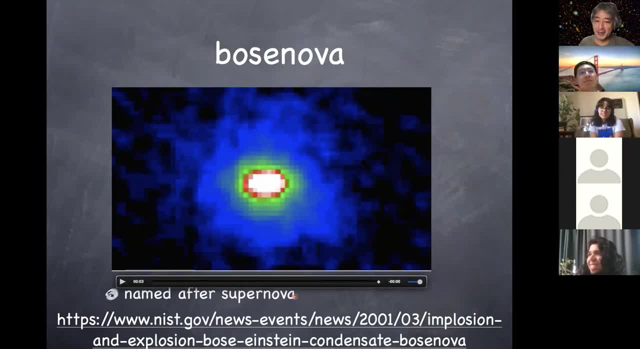 by Saul Perlmutter, one of our colleagues. So instead of a supernova, that's an explosion of a macroscopic star, we are talking about a Bose Nova, which is the explosion of this tiny Bose-Einstein condensate, And that's what you can see here. 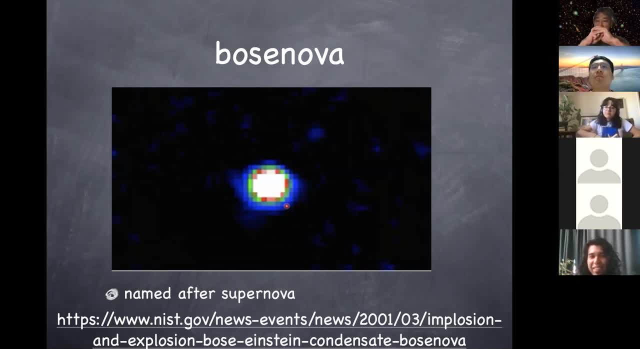 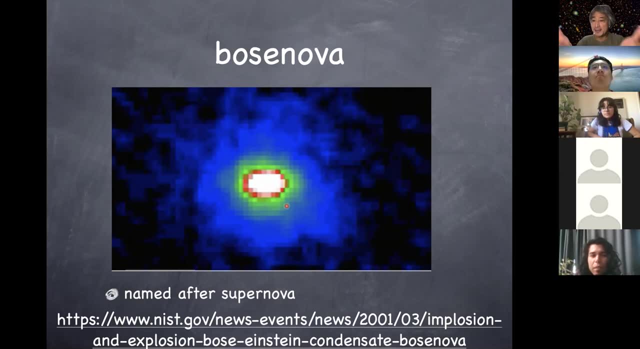 By turning the dial, Bose-Einstein condensate first implodes, bounces back in this explosion and that's the Bose Nova. So the sign of lambda, as you said, has a very important role in all of this business. Okay, I see. 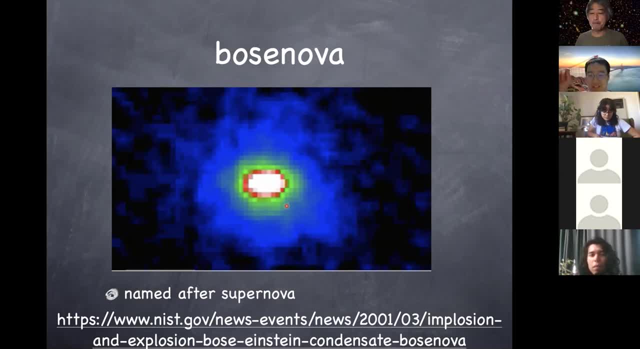 Thank you, And I have another question. Okay, So in Type II superconductors we know we can also have vertices because the magnetic field can penetrate through the superconductor. Does that mean the superconductor has like angular momentum? But I don't see anything like. 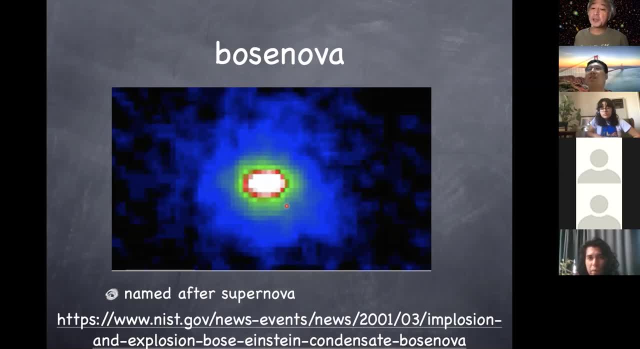 floating inside the superconductor. It is floating actually, Yeah, also inside the superconductor. when you have this flux tube, then there is a supercurrent going around it And that's something you can understand from classical field equation again, and we will talk about this. 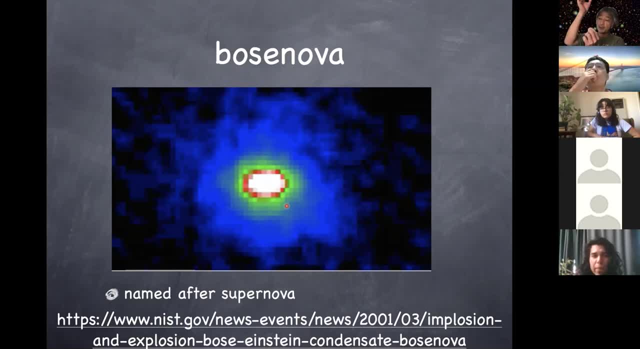 So in order to have the magnetic field trapped in a tube like this, you can use Ampere's law that the current going around it should correspond to the magnetic flux going through it. So if you have a trapped magnetic field in a superconductor, 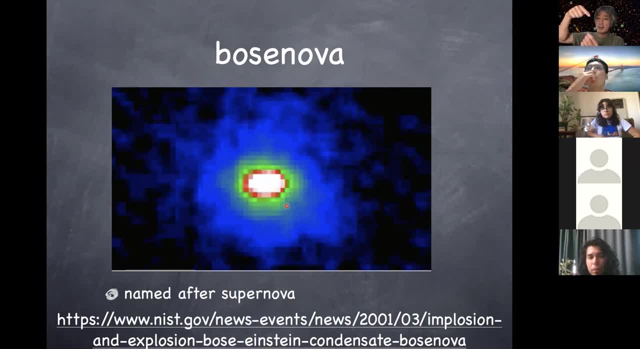 there has to be a current around it, And that is a supercurrent which is the analog of this circulation in the boson-Zheng condensate we talked about. So boson-Zheng condensate is superfluid and once superfluid. 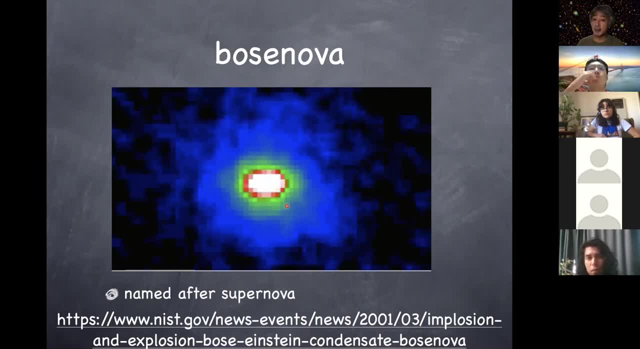 carries electric charge. that is the case of superconductor. and it becomes a superconductor where you expect to have electric current flowing in a persistent way, again topologically protected and hence the supercurrent, with zero resistivity. So we will talk about that. 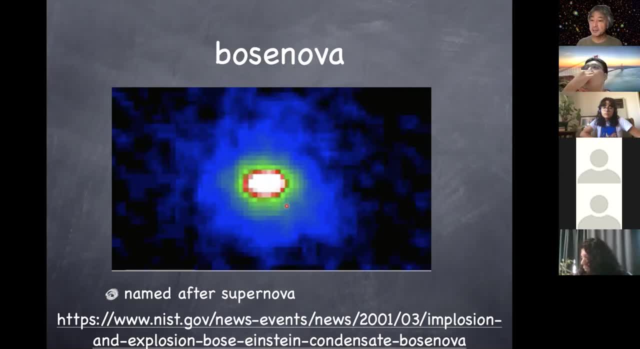 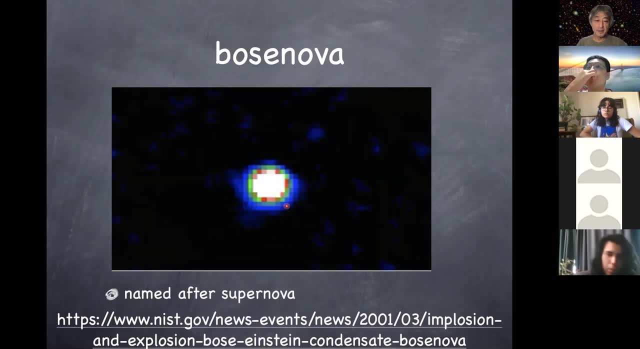 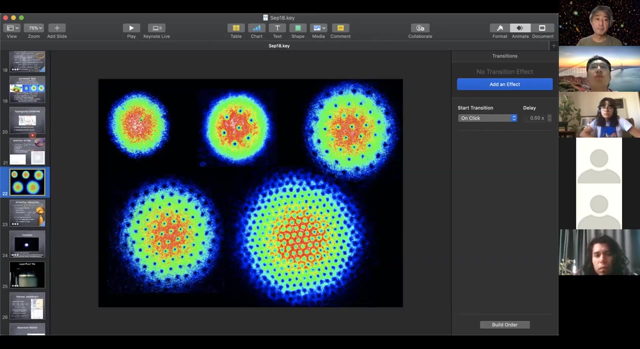 Okay, I see Any other questions on this. I just had a very quick question on the formation of vortices. It's a result of the conservation angular momentum, and that's either by acting on a torque or rotation in the superfluid helium case, or 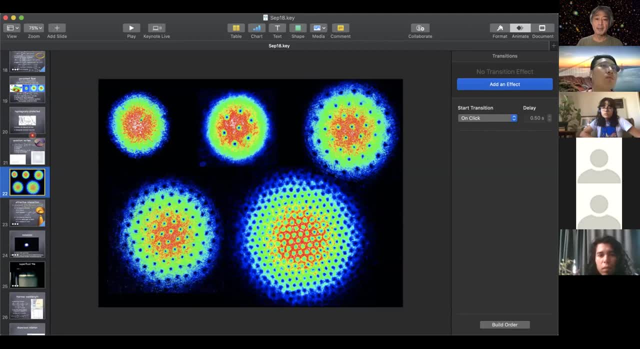 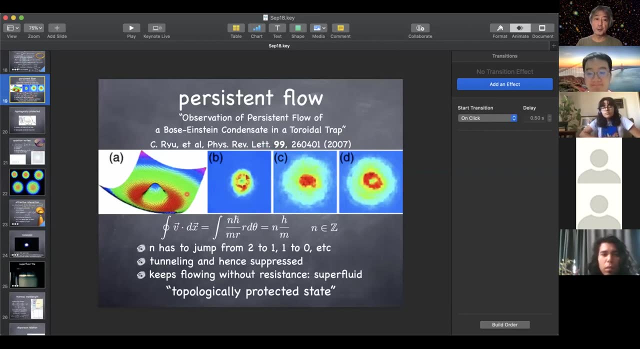 doing potential. So those are two different ways of forming these vortices. Right, right, that's right. So you can first form a boson-Zheng condensate with this kind of trap and, if it happens to be circulating already, just removing. 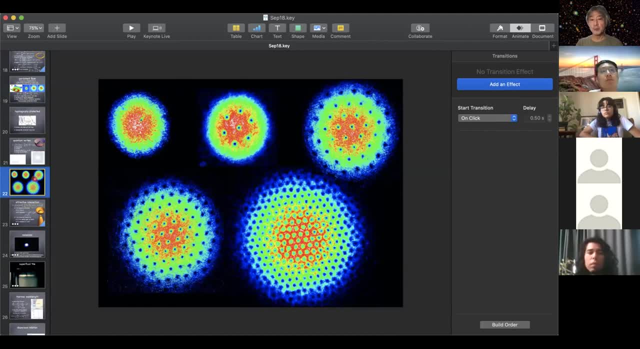 the trap would lead to this set of vortices, or you first form a boson-Zheng condensate and find a way of exerting a torque on it to force it to start to rotate. Either way is fine. Okay, makes sense.